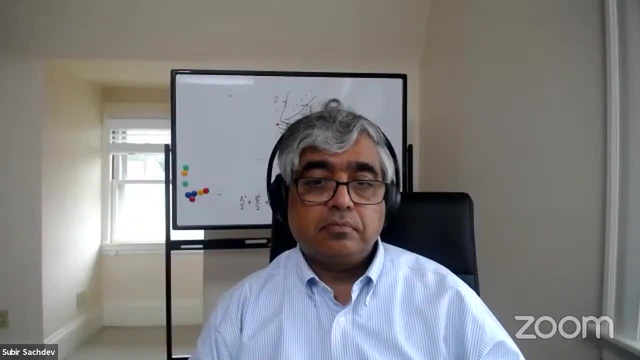 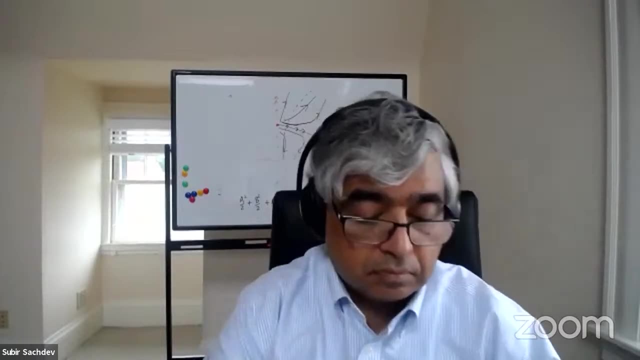 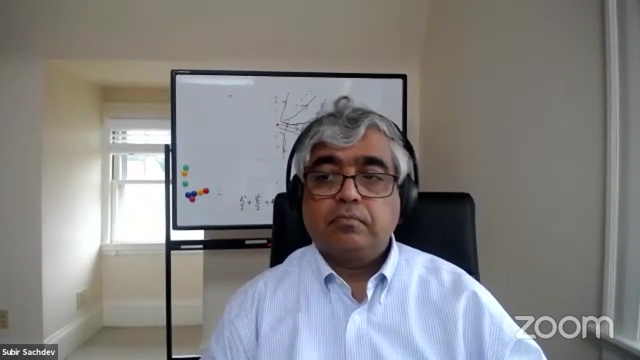 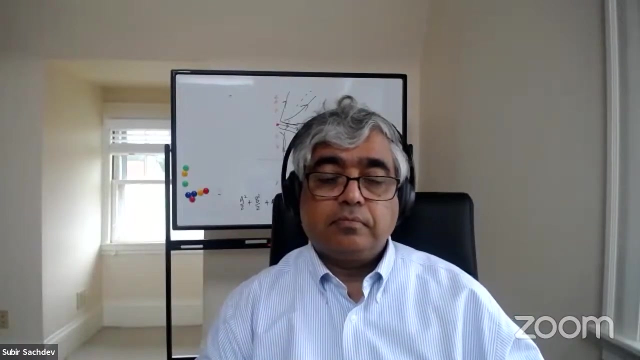 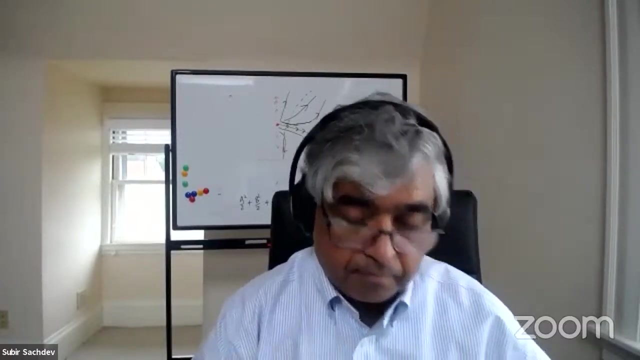 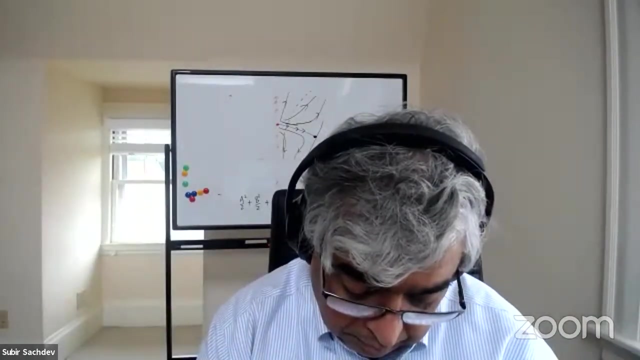 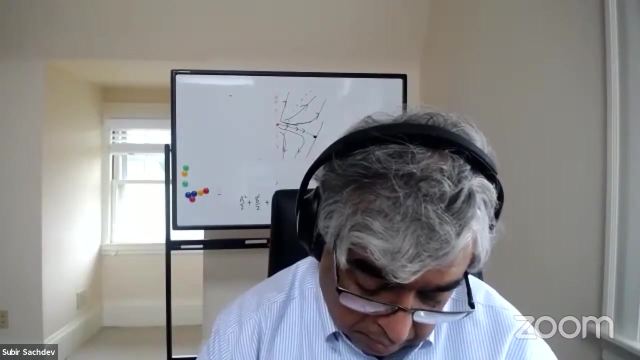 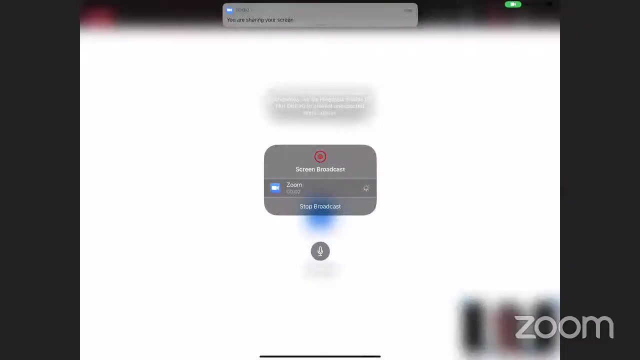 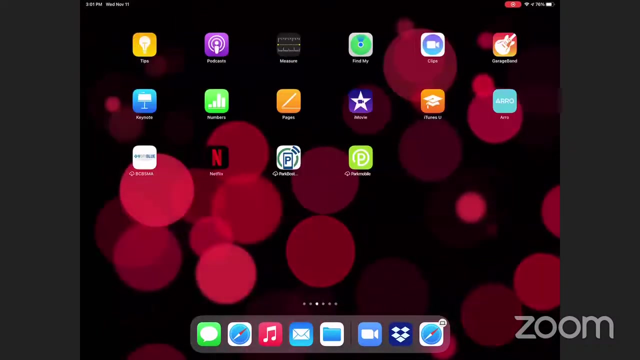 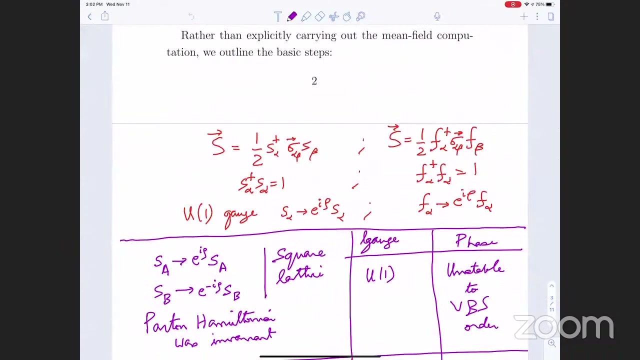 Thank you, Thank you, Okay, good afternoon everyone. So we are talking about chiral spin liquids at the end of last lecture and I want to continue that discussion And finally show you our long-awaited example of Chen-Simon's topological phase, described by Chen-Simon's gauge theory. 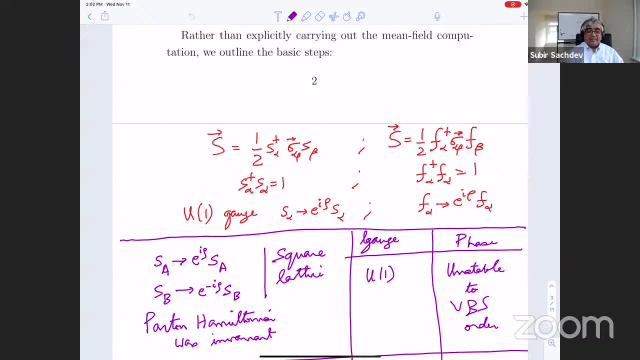 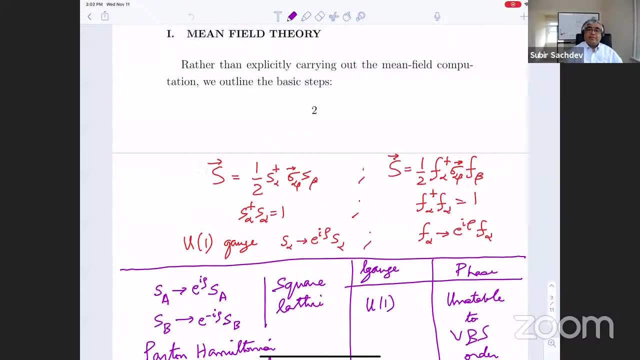 where we are actually emerging from some microscopic Hamiltonian of electrons on a lattice. Okay, but before I start any questions, Also I should note from the last problem set is on the website and I made some corrections to it today and added a few more hints- 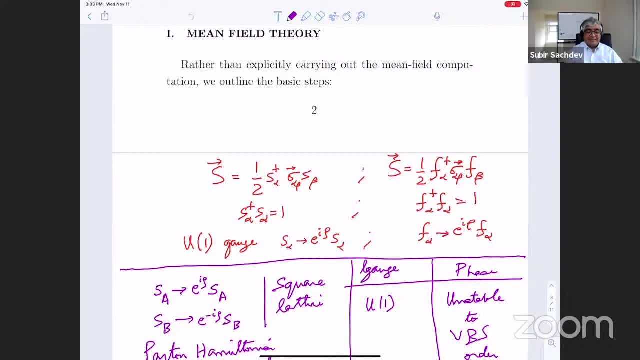 I'm a little worried. I'm overburdening you with this last problem set and also preparing for your presentation. So well, let me know if that's the case. And also, like I urged you, I'm a little worried about the quality of the presentation. 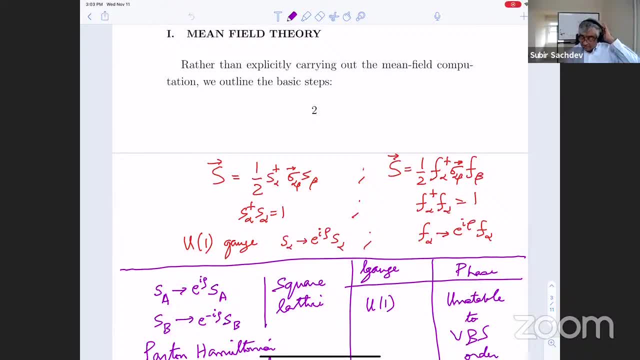 So let me know if that's the case In my message on Slack. look at the problem set soon and I'm sure Hayu and Darshan will be happy to take you along. you know a fair bit of the way towards the solution of any problems you get stuck in. 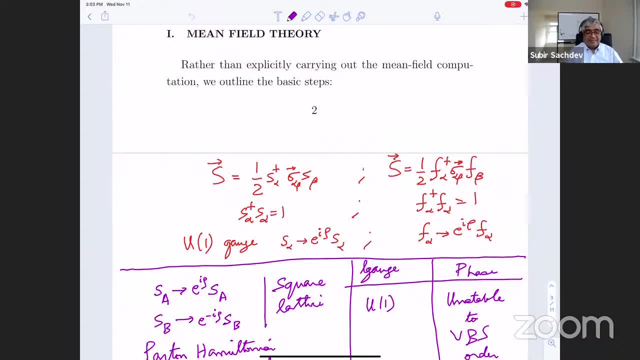 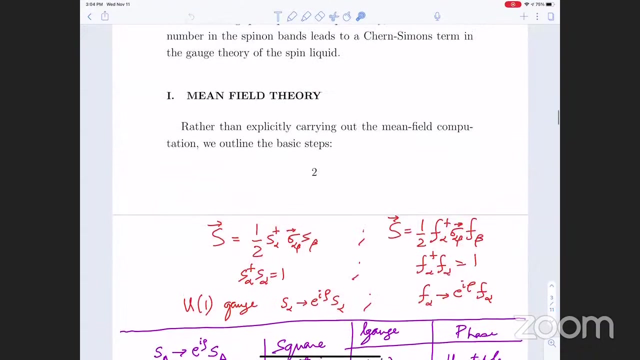 I mean, I think they're all relevant problems. We'll give you a better understanding of all of this if you go through them. All right, any comments or questions? So in the classification we talked about last time, with these different Schroeder, bosons and fermions, I was a little confused why we start with the same microscopic Hamiltonian but we just rewrite it in terms of different variables which are supposed to be equivalent representations, right? 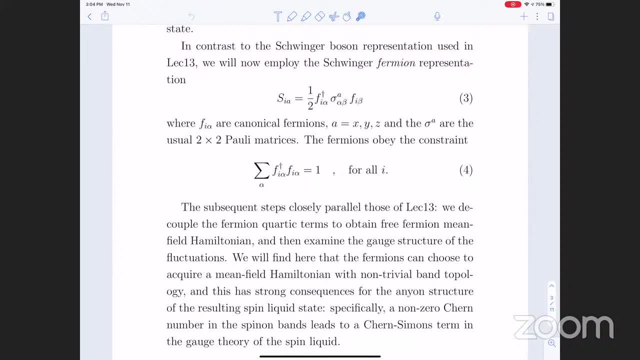 But in the end we get different phases. Is it because we're just looking for different settles, Or are we changing the microscopic Hamiltonian? No, well, you know we don't. as you can see from the way we proceed, we just guess some effective Hamiltonian for the partons. 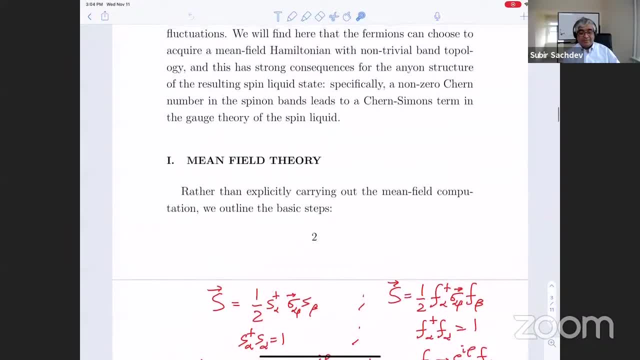 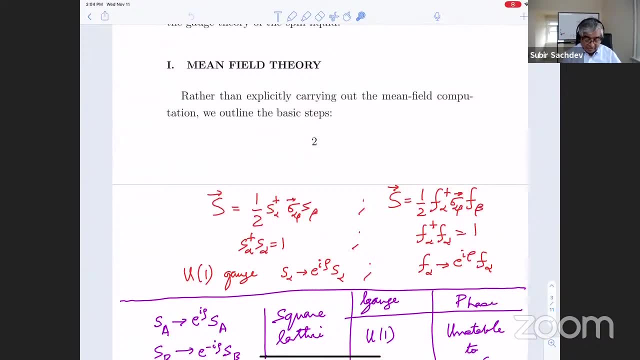 We don't actually work it out, But in principle, if you really work hard enough, you should be able to start from either this representation or that representation and end up with the same answer. Now what happens is that sometimes there are certain states, like the chiral spin liquid state, where that answer emerges very nicely from a very simple mean field theory of these partons, but to get it from the other partons requires a much more complicated procedure where you have to can't treat them as just free particles. basically is what happens. 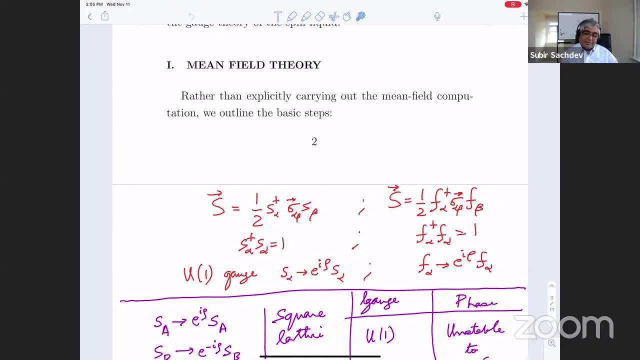 So, so. So, basically, you try to use different representations because they give you rather different saddle point, That is, their mean field. theories at the mean field level are rather different, But if you treated it more exactly you should be able to get it from either side. 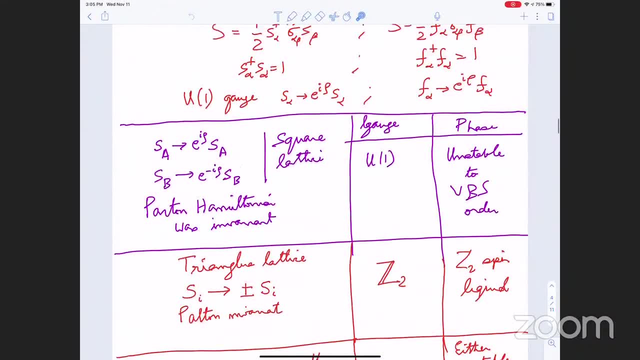 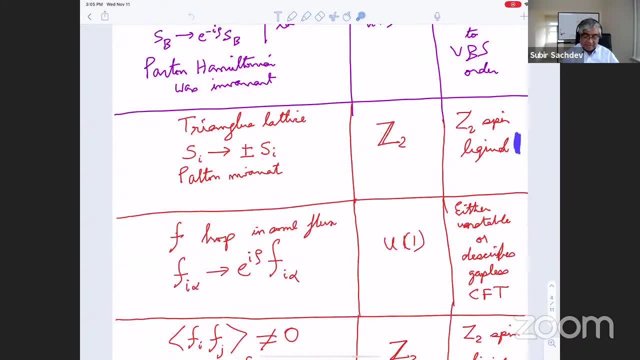 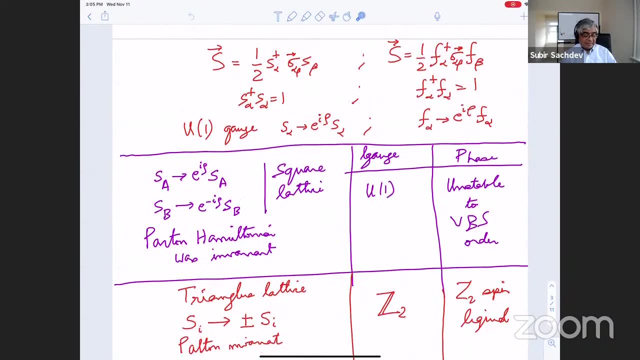 Now there's one exception to this case, where we can get the same answer from either approach, And that's the case of the Z2 spin liquid. We can start from the bosons S And just do the pair them up and then get the gap state and you get a Z2 spin liquid, which is what we did in the triangle lattice. 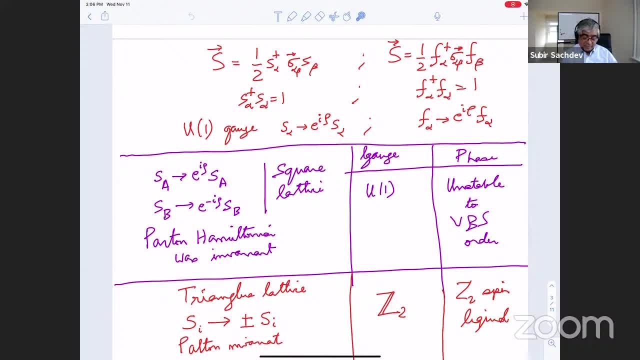 And then the S boson itself becomes the E particle of the Z2 spin liquid. Conversely, you could address exactly the same Hamiltonian using the F particle, And then the F particle becomes the epsilon particle of the Z2 spin liquid. Now which is the better approach? 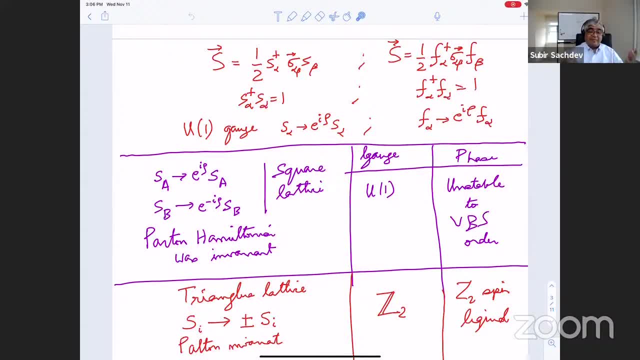 Even though, at least topologically, They're in the same state. Well, again, that depends on numbers. Depends on the specific Hamiltonian. in which case is the S particle lower in energy? in which case is the E particle lower in energy? in which case is the epsilon particle lower in energy? 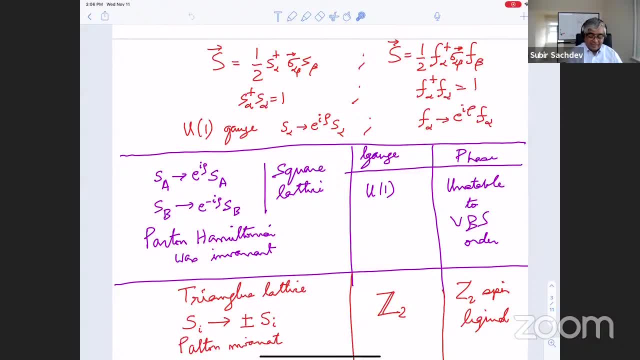 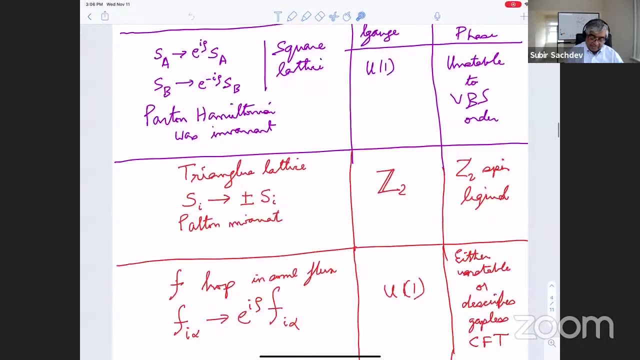 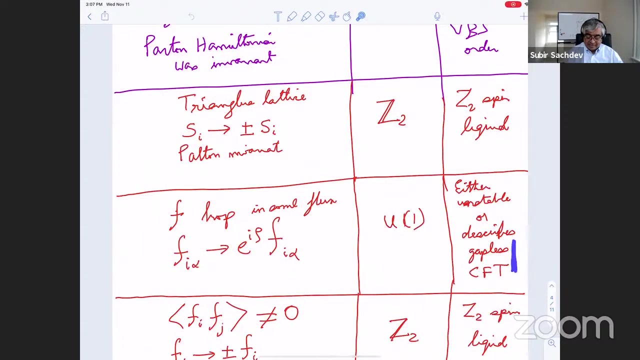 That's an invariant statement which you can't predict ahead of time without doing some very careful calculations. And then, towards the end of the course, you're going to see that the same trick will help us understand Even these gapless CFTs. for the gapless CFTs, there are dualities that emerge at long distances. 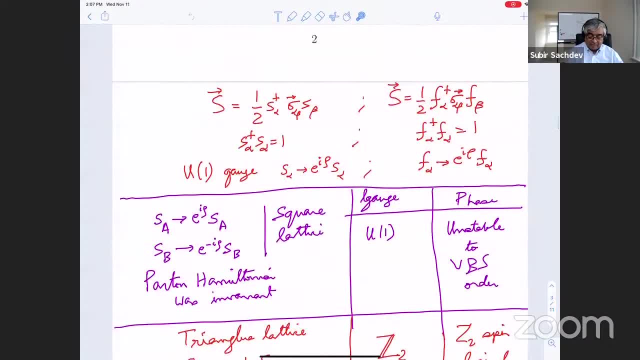 And those dualities help us see the equivalence between the bosonic protons and the fermionic protons. OK, I see, Thanks, Yeah, But really we just, you know, We just We're just trying whatever works. I mean, that's the honest answer. 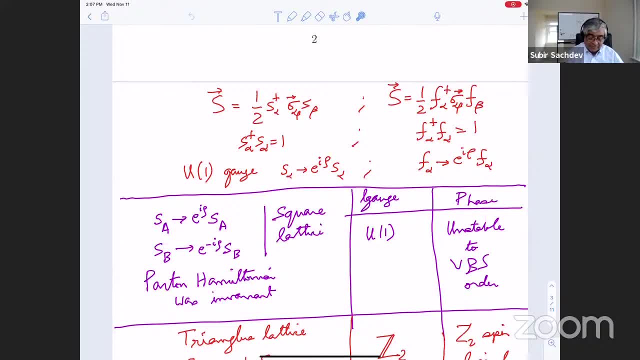 And because we do some very simple mean field treatments and then hope to get some understanding of the topological phases And the, And I think the remarkable thing is that essentially all known topological phases, certainly those that have anything to do with any experiment, can be described by some kind of very fairly simple mean field theory on some part on construction. 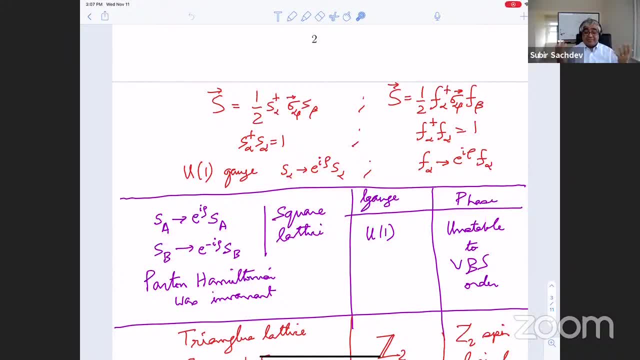 Which is why I'm using it. It seems to work in practice, So it just becomes a matter of finding the right part on construction to describe a particular state in at a mean field level, And that's really what all I'm doing in this course. 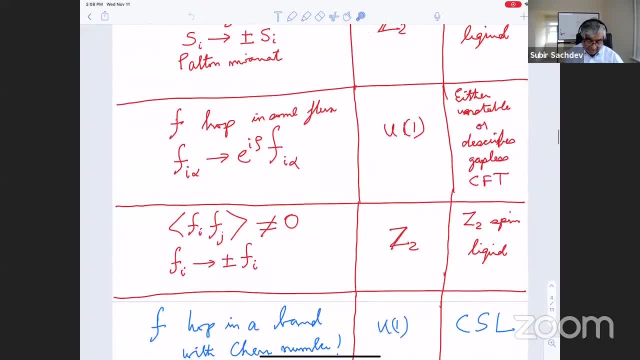 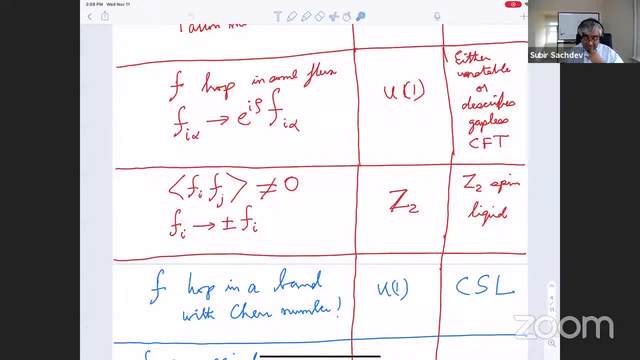 So for the carl spin liquid. in fact it was written, written down as a theory of bosons by Laughlin and Carl Meyer about a bosonic protons, But actually no, they did it in another very clever way. but the simplest way to get it, which is the way when Milchik and Zee got it, is by using fermionic protons in a band of a Chern number. 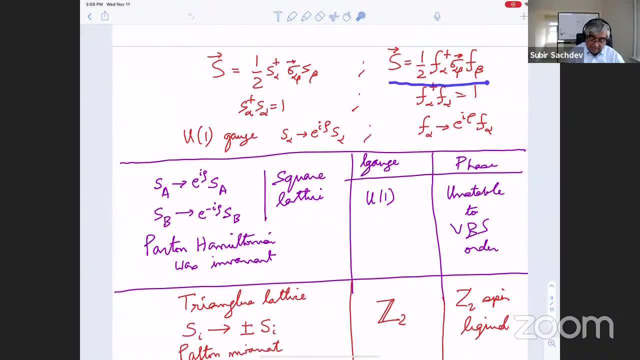 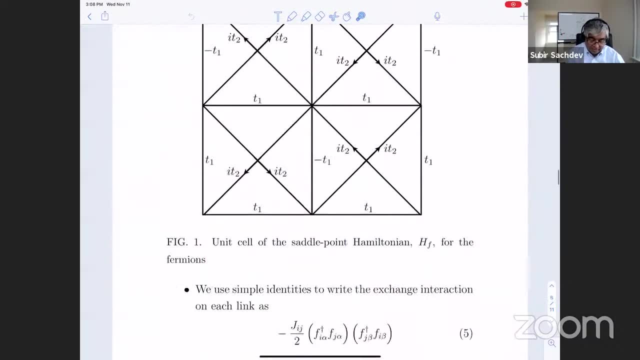 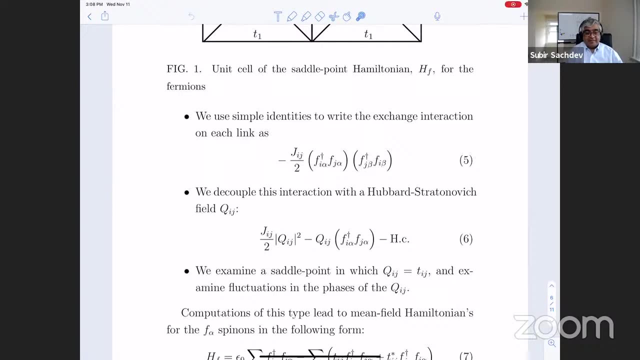 So so what we do is we take this fermionic proton construction, You put it into your favorite anti-ferromagnetic Hamiltonian And then you So then, After some rearrangement, you get a term like this: A four Fermi term, an interaction term from the exchange interaction, GIJ. 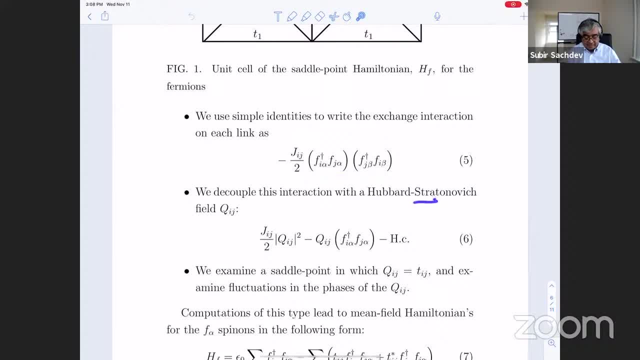 Then you do a mean field theory on it by a Habert-Renovitz transformation, by introducing this field Q. Notice now it's F, dagger F, rather than B, dagger S, dagger, S, dagger, as we had before. And then you just replace Q by an average value. 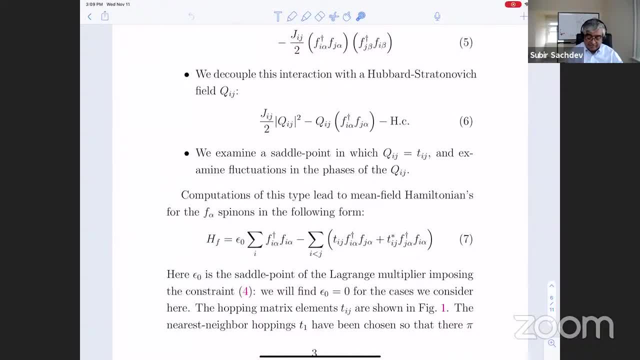 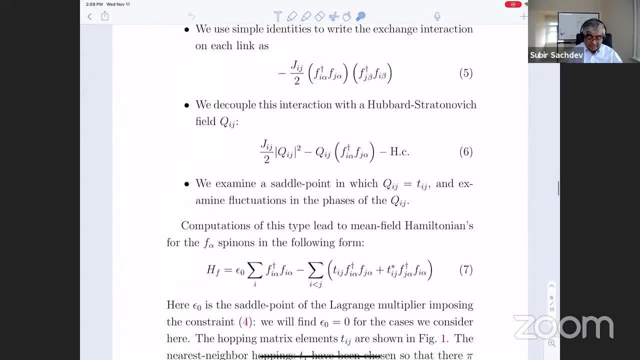 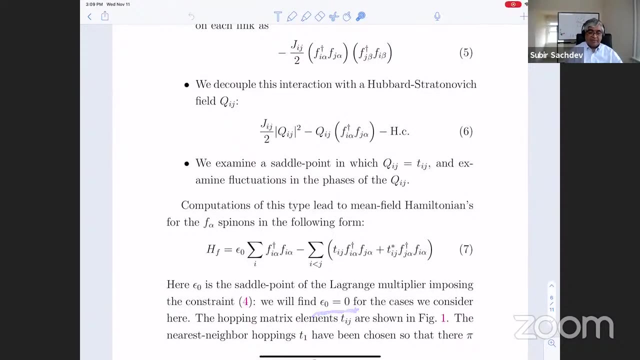 So when you do that, you get some hopping, some free Fermi on Hamilton. So this is the Hamiltonian. There's also a on-site term that imposes the constraint, And it turns out here that there's a very simple solution of the constraint, that this is just zero by particle, whole symmetry. 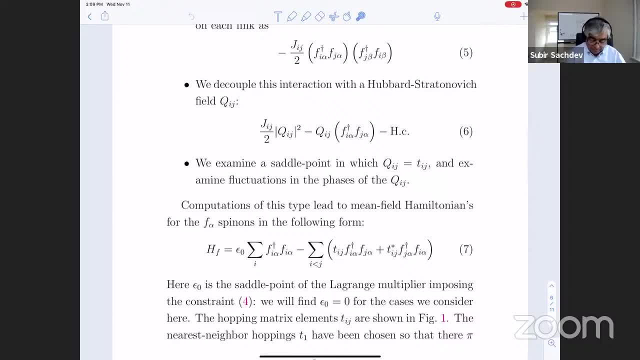 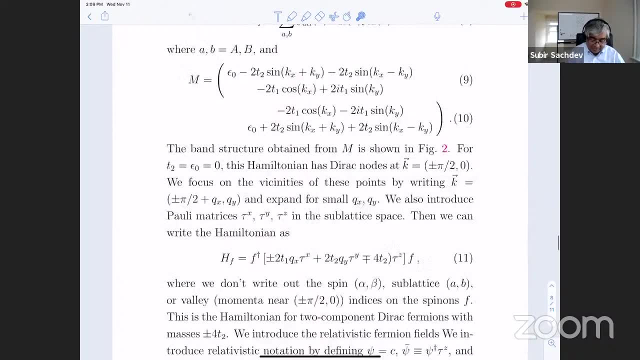 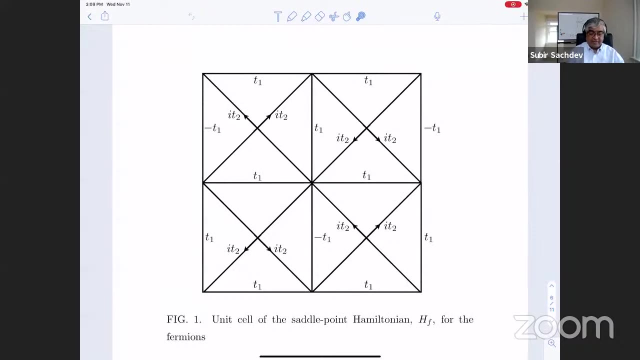 You want to be at half filling, And so the chemical potential is just zero. So now we just focus on this. Hamiltonian and people's work has shown us Where did it go Right here That this is the. these are the values of QIJ that seem to do well on on the class of models that give you this curl spin liquid. 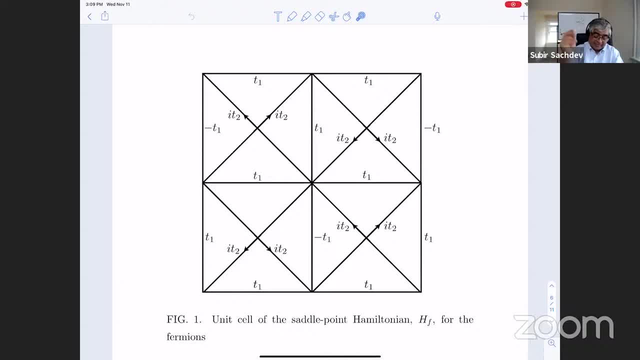 So this is really, at this point, you know, a very crude guess, but it's. it's a guess that allows us to build new types of states. That's kind of what we're trying to do. So. so this configuration has the feature that, if I compute the flux which is the product of the phases of the TIJ around any triangle, 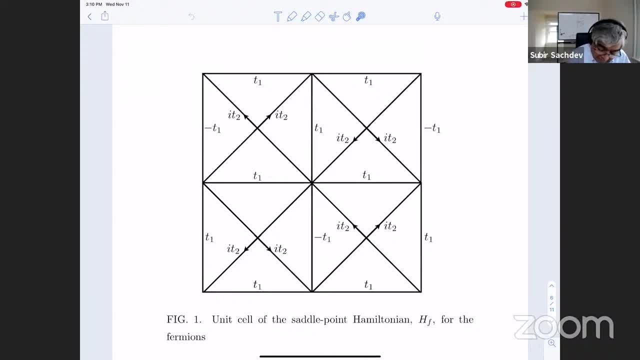 I get PI over two. So, for example, if I go anti-clock or no, let's, let's go clockwise this way, clockwise around this triangle, Then I. here's plus one, here It's minus I, because of going against the arrow, and here's minus one. 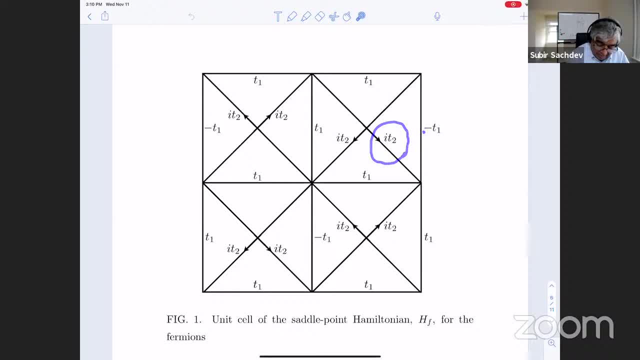 So that gives me an eye. clockwise around this triangle gives me an eye. How about clockwise around this triangle? I get an eye Clockwise around. You know this one here. So you would go clockwise and I'm going clockwise. That's anti-clockwise. 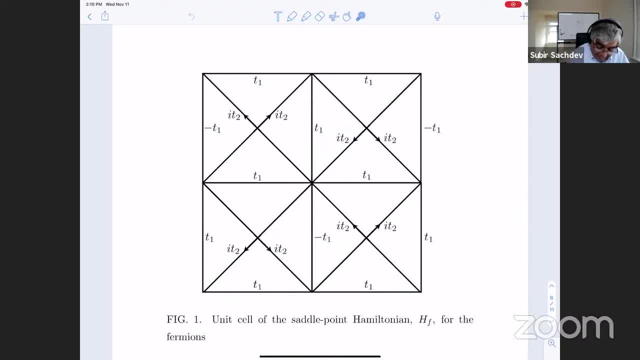 This is clockwise. You get an eye and a plus and a plus and then the fourth one, which you may well, which is the fourth one. Anyway, pick any triangle, any right triangle like this. there's four in each square and all of them clockwise. give you an R PI over two phase. 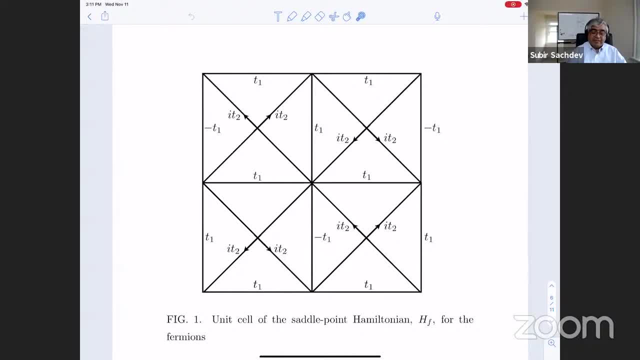 So, basically, this is like a half straddle problem, where there's a flux Of uniform, flux of PI over two in every right triangle, small, small right triangle. So. so that makes it very likely that you're going to get bands with shown number. 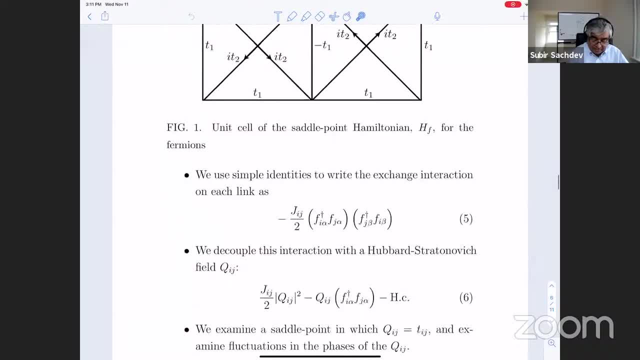 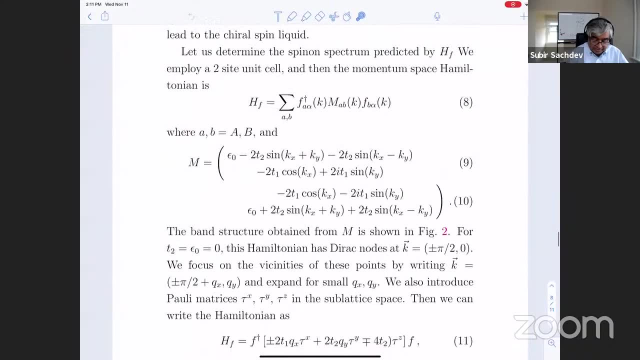 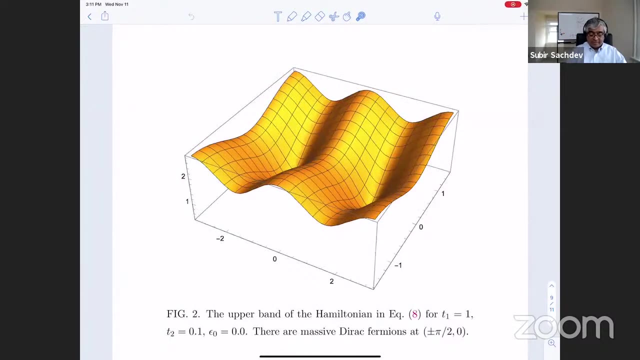 And indeed that's what you find if you diagnose this Hamiltonian. This is what it looks like in momentum space And you just work out the band structure of that. You get this band structure here. So this is the upper band And there's another band which is just the mirror image of this uh at negative energies, and you occupy the the uh, the mirror image band. 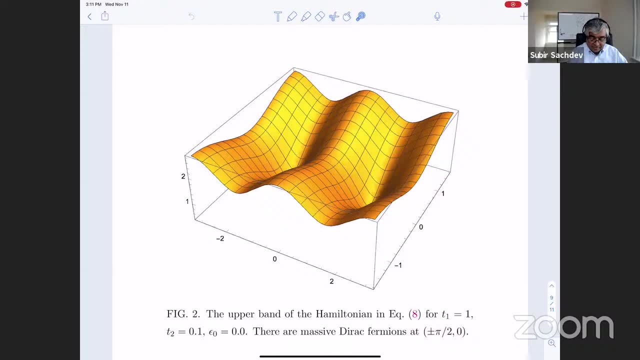 So what you notice here is that, at least for the parameters chosen, uh, there are these, uh minima here and near the minimum, the dispersion- uh, you can work out- looks like the dispersion of a relativistic direct particle. 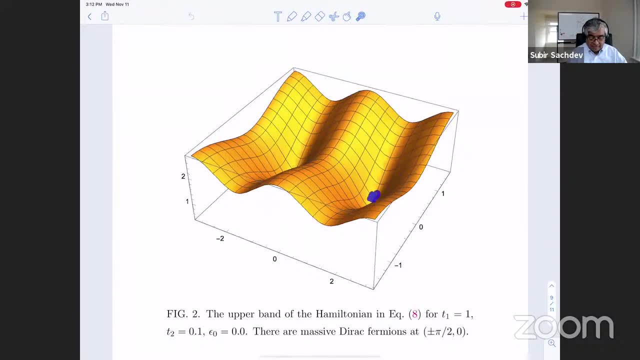 So you can think of these, Uh, these minima, uh, as representing, you know, some emergent low energy direct particles, at least near the minimum. And how many direct particles do I have? Well, I you can see two of them, one here and one there, and then there's spin up and spin down. 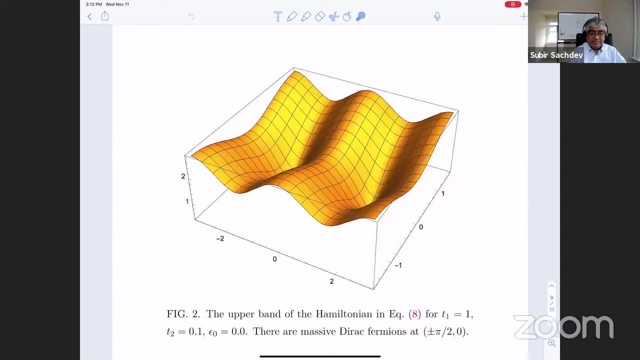 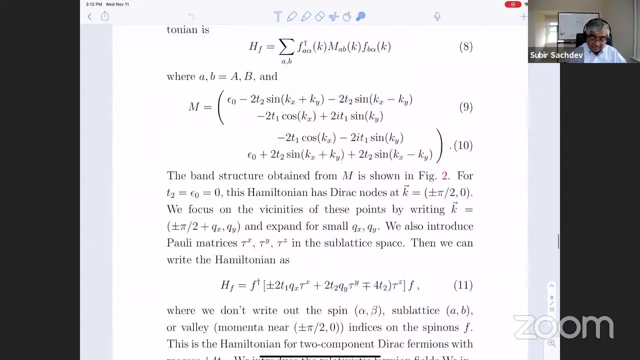 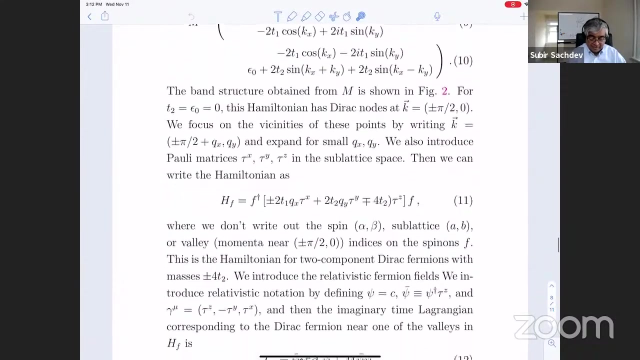 So there's a total of four, uh two, plus one dimensional massive direct fermions, And the mass has to do with the fact that this is doesn't go exactly to zero, It's it's a parabolic minimum And furthermore, you can even actually take this matrix- the Hamiltonian is this matrix, this two by two matrix, and take the continuum limit appropriately near those points, just like you do with graphene. 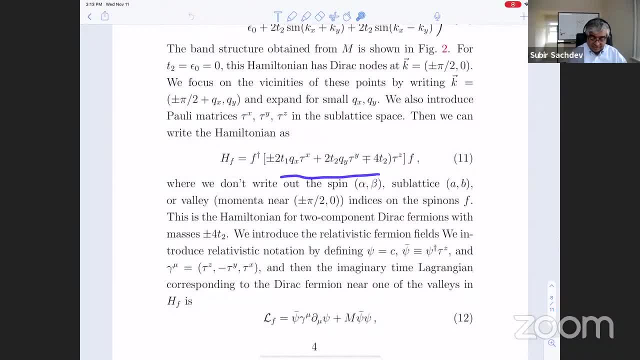 And after some, you know this is what you get. And then after some changes of notation, which are all described here, uh, that should be an F over there. Um, let me change that. So this is an F? Um. 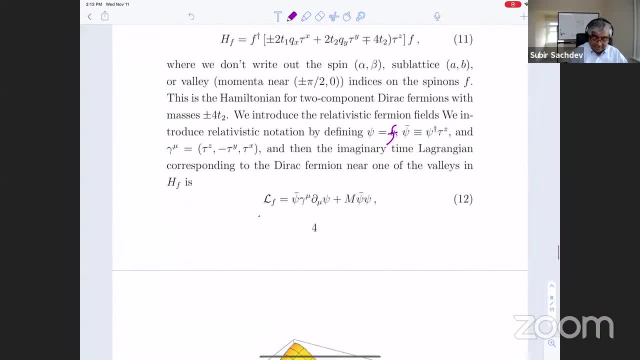 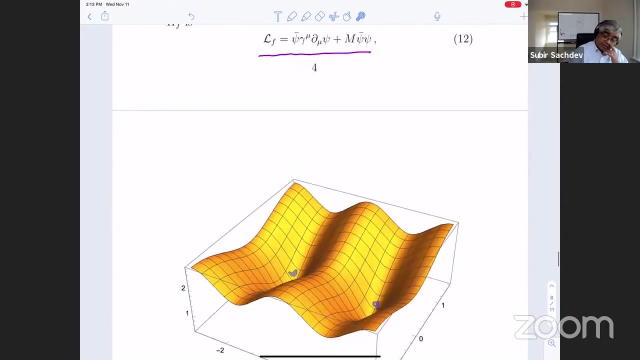 then you get in fact precisely the massive direct Hamiltonian, So you can actually derive the relativistic form with all the notations that particle physicists love. uh, for this minimum and the other minimum, and so on. Okay, All right. 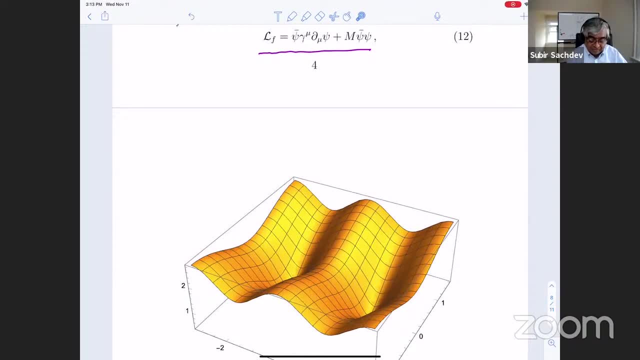 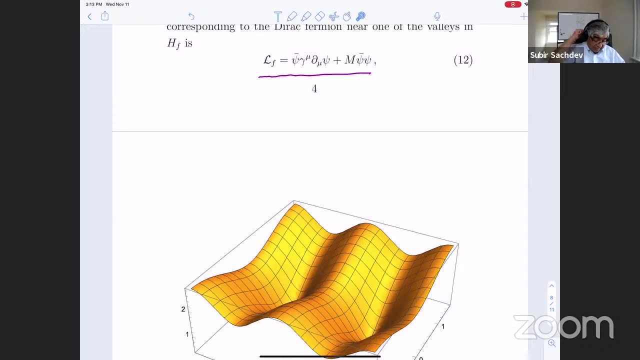 So that's great. Uh, and then from this direct part, direct dispersion, uh, you can work out the churn number. So that's easy to do in this, Uh, in this limit, And I think how you probably did that in one of the sections- uh, and basically for every direct particle M you get a churn number of a half uh for uh, for any given band. 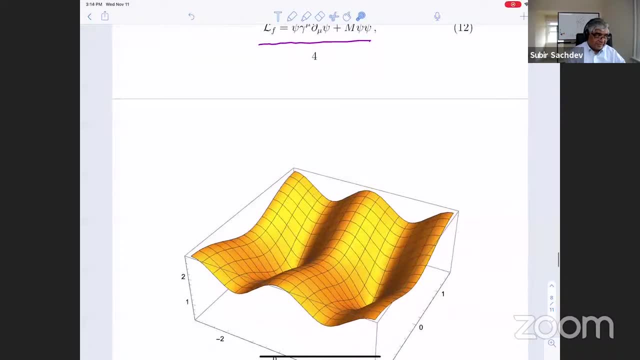 Uh, so they have to be an even number of direct particles, Otherwise you'd get half interest on turntown number, which you know is not correct. So you get a churn number of a half And the key question is: is it plus half or a minus half? 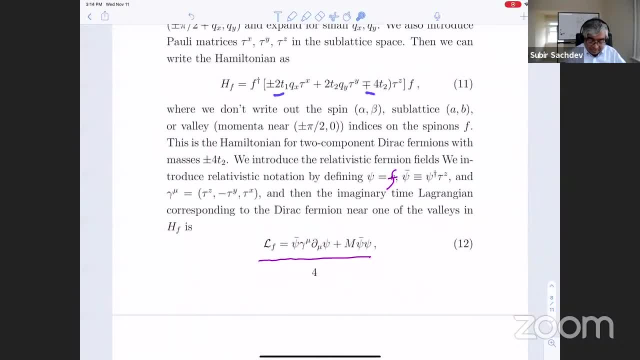 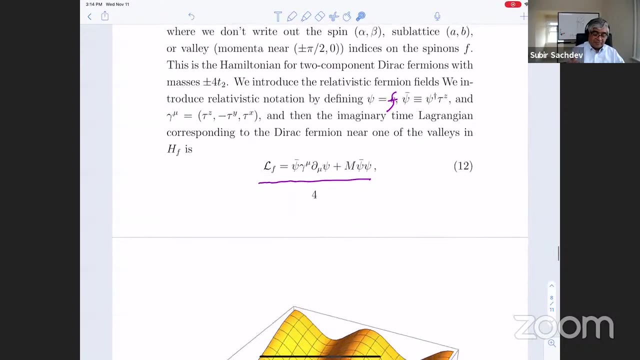 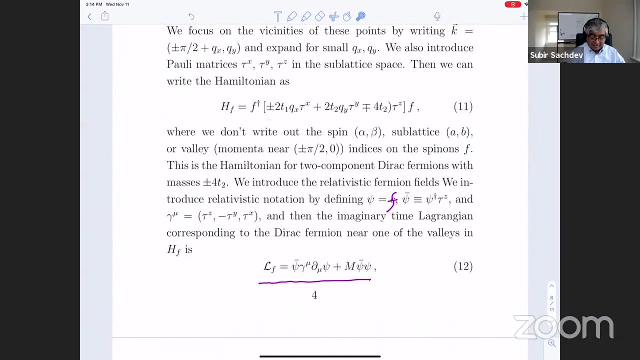 Uh, and that depends really on the details of all these plus minuses here, Uh, and if we just work out those signs you get either plus one or minus one. and that's the quickest way, without doing the full band structure, of figuring out the churn number of any band. just hope that it has some almost direct points and just compute, uh, uh, these signs near the direct point, the sign there and that sign there, uh, and the sign of the mass, and together that you can quickly figure out what the churn number is from that. 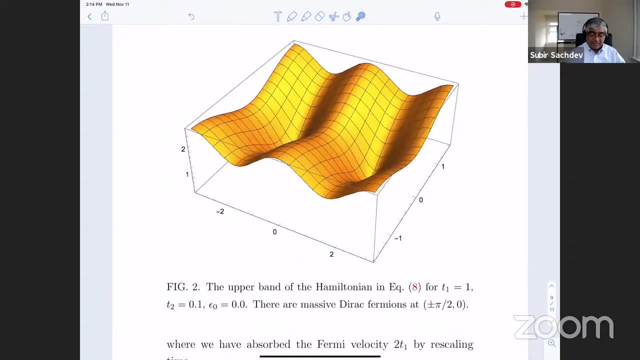 So anyway. so you do all that And you find that the upper band has churn number plus one, say, and the bottom band has churn number minus one, All right, So that's the mean field theory. You get spin ons moving in a churn in a churn band. 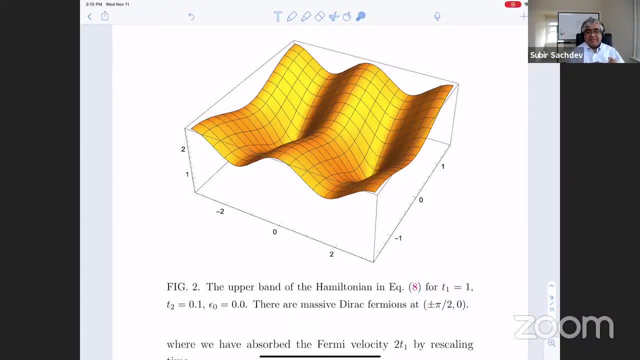 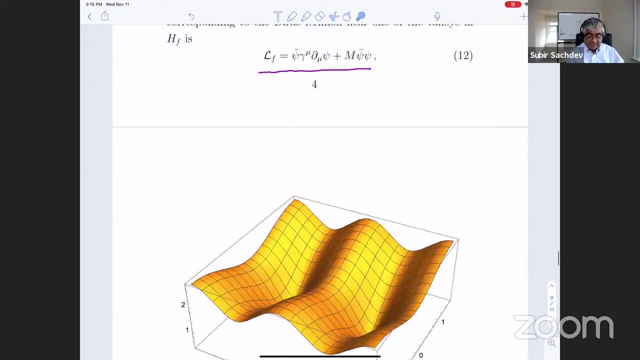 So this turns out to have a remarkable consequences to the gauge theory, because now let's take the mean field theory and do fluctuations, So the flux in the mean field theory, you just set the Q, I, J to some some, uh, some fixed value. 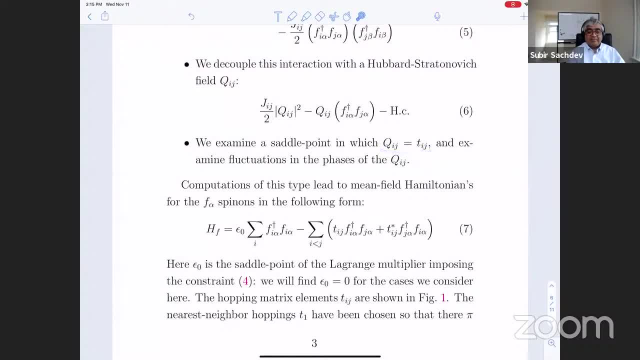 Now we're going to fluctuate them. We're going to go. you found a saddle point. Now we look at fluctuations about the saddle point. So what's the important fluctuation of Q I J? Well, just like they were for the Schrodinger boson theory, and they are the phases of the Q I J. 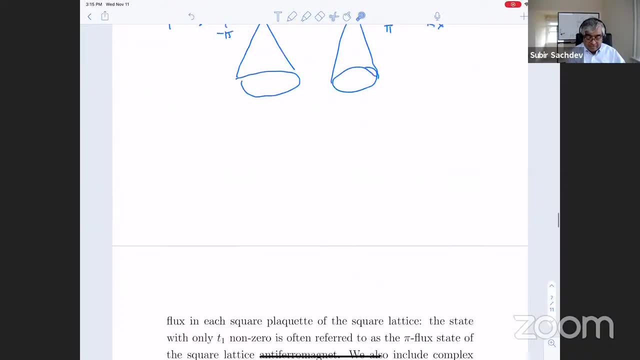 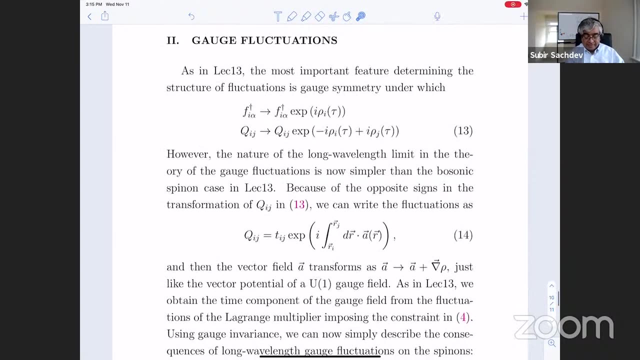 Those are the only ones that can possibly give you anything interesting, because they're constrained by gauge invariance. Okay, So what is the gauge invariance of the theory? Well, this is an exact statement of the theory. Okay, So this is an exact statement of the underlying path, integral, which you've met before, the. there's a gauge transformation, row I of tau, but row I is the arbitrary function of I, the arbitrary function of tau. 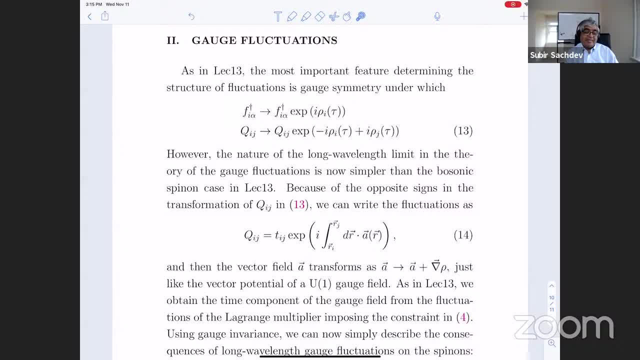 And if you make this change of variable, you will get the same action back: Uh. so so there's a gauge invariance, and this tells us that the phase of Q transforms this way as a function of uh. function of row I. 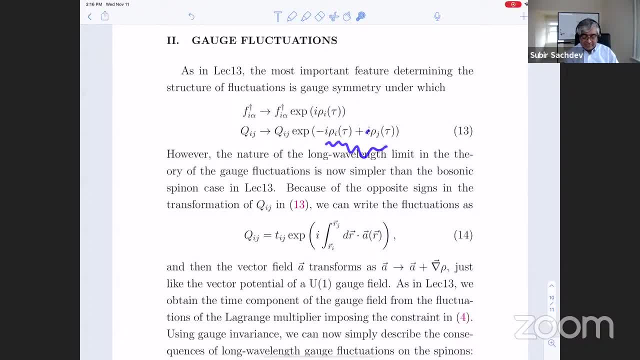 And now you, you'll see that this, this is actually a very nice form. which is the difference? So if you imagine that we're just the phase is slowly varying and we're only interested in things that are slowly varying on the scale, uh, of the lattice, then this you know so. so J is equal to I plus X. 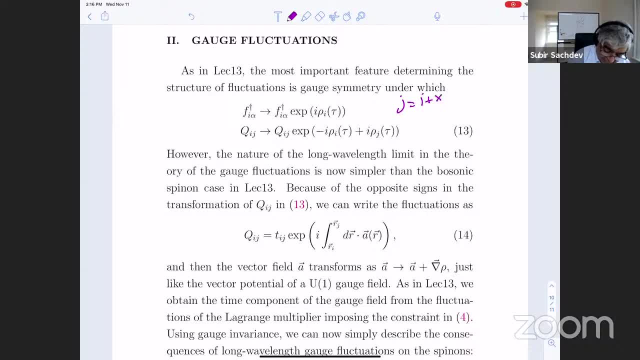 Let's say, just one distance away. and this quantity here is just equal to I, which is the number I, then D by D, X of row. So we see that the phase of Q Trans uh changes by the gradient of the gauge transformation, and that immediately tells us that the phase of Q is just like uh, a gauge field. 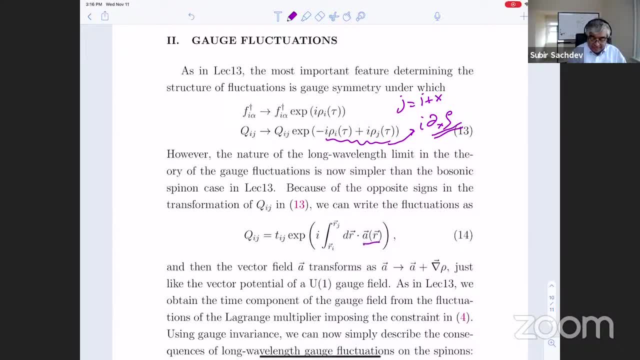 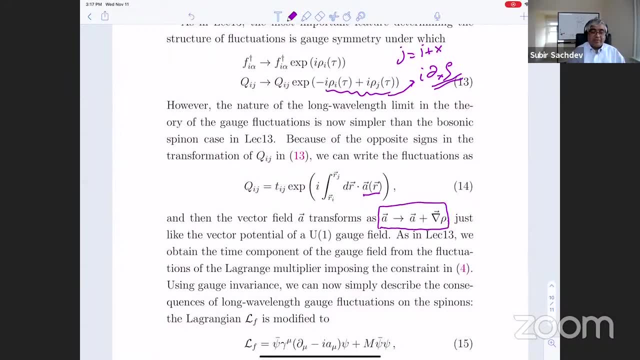 So we just call the phase of Q the gauge field little a and a will transform just like any self-respecting U on gauge field. So there it is. So now there's our emergent gauge field, the phase of Q. uh, and this is actually the ease of the fermion way of doing things. 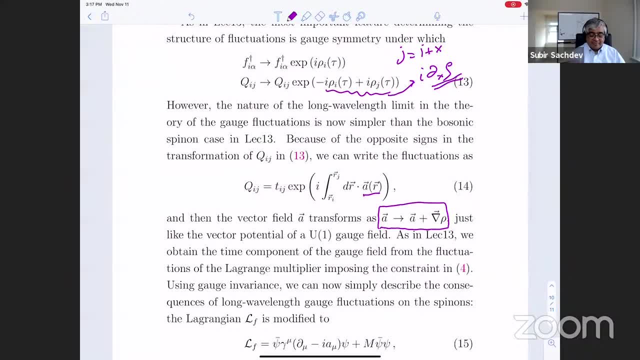 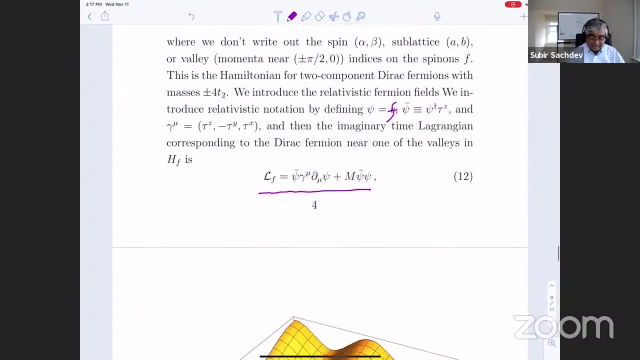 Uh, as long as you don't have pairing, the phase of Q is automatically just your, your, your one gauge field. So just knowing this, now, when we do fluctuations, we we can, without any work, we can figure out what is the correction to the Lagrangian for the spin-ons, this direct Lagrangian. 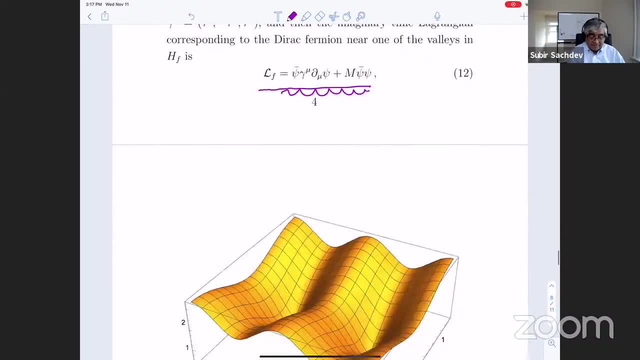 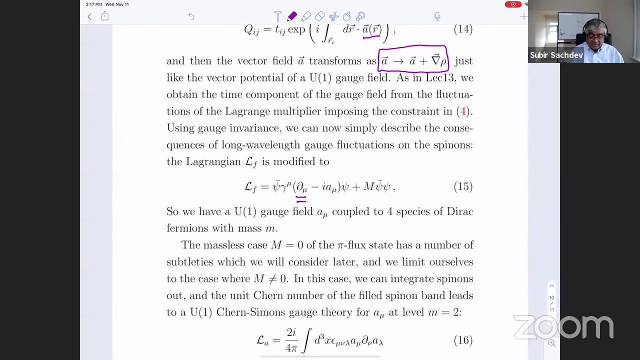 They're going to couple to the gauge field and how are they going to couple where they're going to couple? in the only way it's possible, Because from gauge Variance, uh, and all you have to do is make that gradient of covariant gradient. 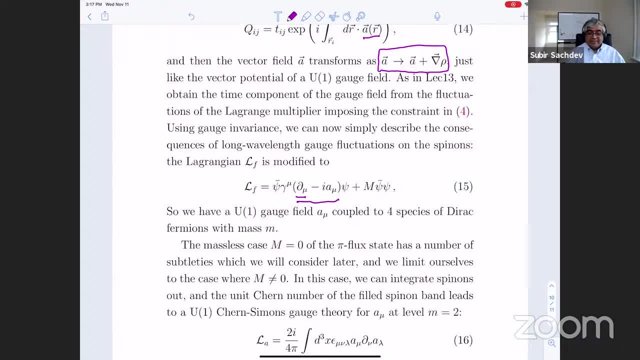 So extremely simple. You just work out the theory of the spin-ons and then you'll gauge everything and you have an emergent gauge field which is strongly fluctuating. Okay, So there's our theory. Now our theory really is quantum electrodynamics, a couple to four species of massive direct. for me on that, that, at least at low energies, that's the complete theory of fluctuations. 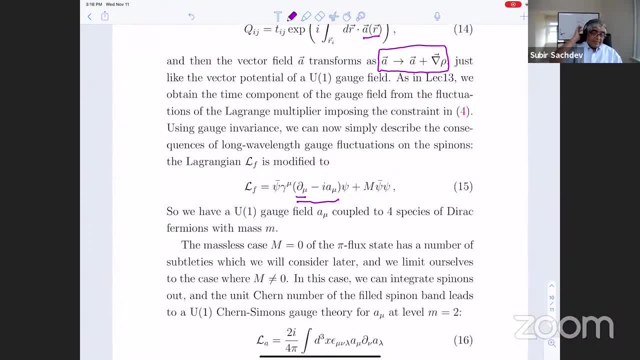 About The state. Okay, So now what's unusual about this theory? there was unusual about this theory, of course, is the churn number of the fermions, which is partly hidden in this notation, because in this notation you've made kind of different choices for the continuum, for me, on the different valleys, 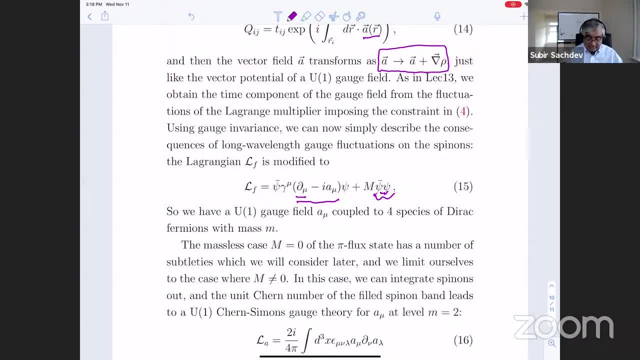 So you really have to go back and make sure you did that correctly on the microscopic scale? Um, but we don't have to Worry about any of that. We know exactly what happens when you couple a gauge field to a band in the churn number. 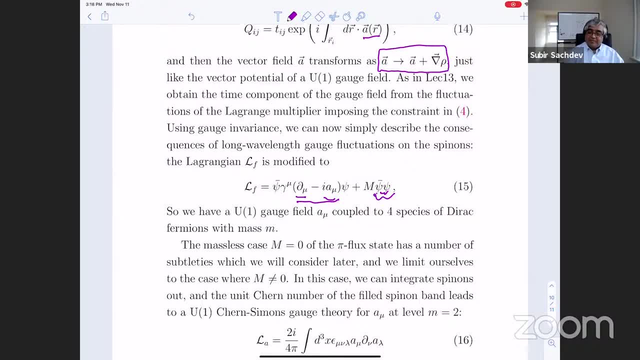 That's exactly what we worked out, uh, for the integer quantum Hall effect, And then later on, when we talked about churn numbers. when you couple it, a couple of the external electromagnetic field, to the electrons, you know a bad end of the churn number of what we got was the Chen Simon's term was coefficient. 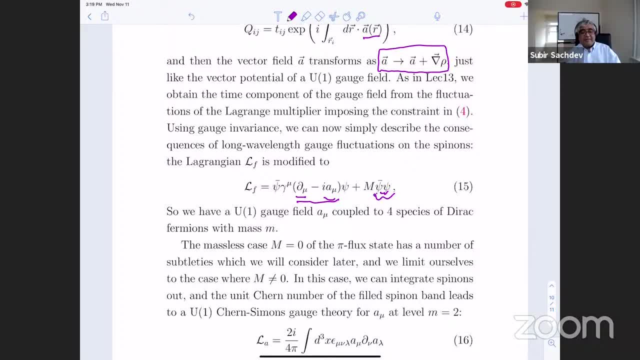 What's the churn number of the band. So exactly the same thing should happen here. Uh, so I integrate out when I get rid of, when I, since the fermions have a gap, I can remove them and get an effective theory for the the gauge boson. 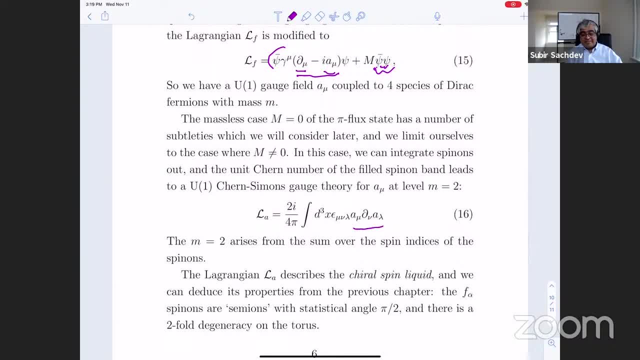 Now, it's a strongly fluctuating grade boson, It's an emergent gauge field, not an internal gauge field. Uh, and for each occupied churn band I will get uh, coefficient one, Okay, But now comes the key difference: um the coefficient, this is not one but two, and that's uh. and from our chapter on Chen Simon's gauge theory we already know that's going to make a huge difference. that's M, So this, so this whole thing is: M equals two. 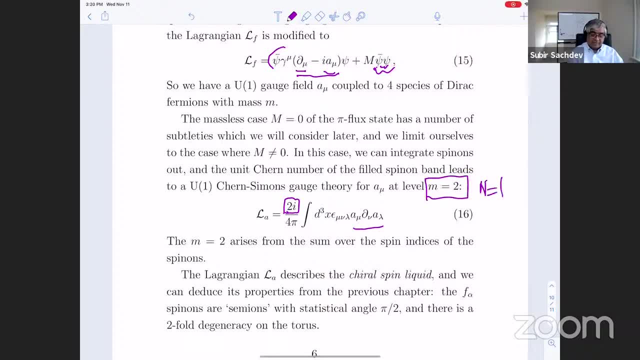 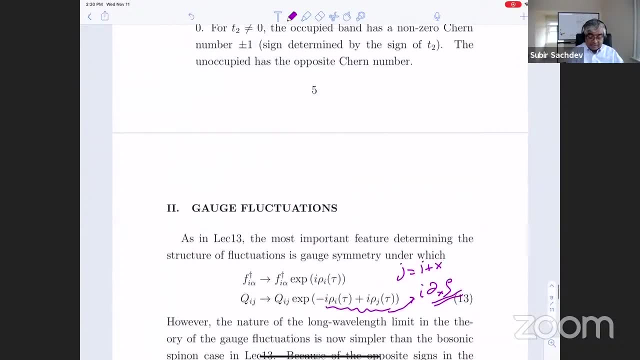 And, of course, N equals one is it's one one Chen Simon's gauge field. Where's the two come from? The two comes from the fact that there are two spins: You have spin up and spin down. You have spin up and spin down fermions occupying the lower uh band. 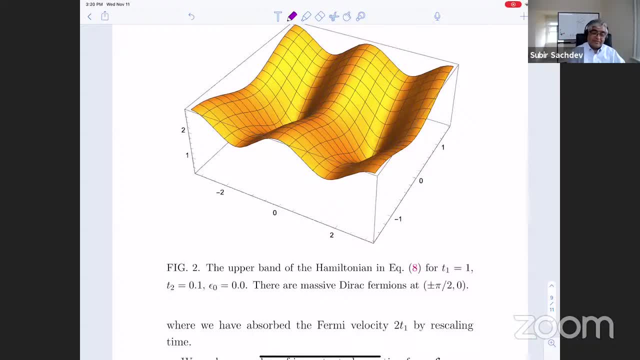 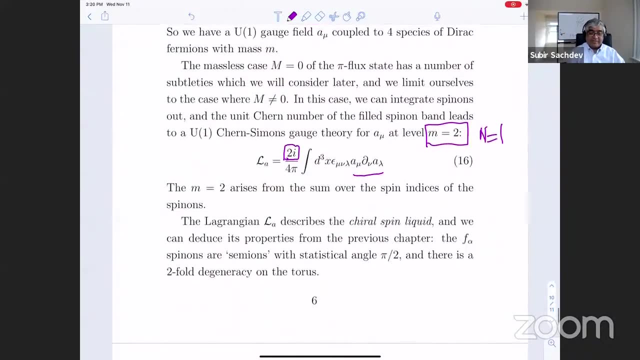 So each one of them gives you one Chen Simon's term with a unit coefficient, and they together give you uh a factor of two. Okay, So there we have it. There's our uh first microscopic derivation of a Chen Simon's gauge theory with a non-trivial coefficient: uh M equals two. 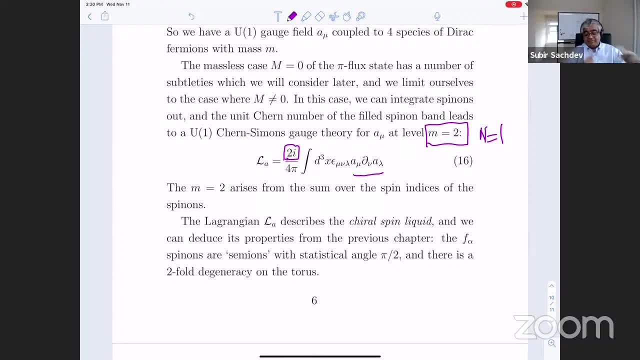 Uh and so this. so now? So when we look at the exchange of this, the spin ons- uh, initially we started out in mean field theory. the spin ons, we said, were fermions. but now this theory is telling us, no, they're not actually fermions. 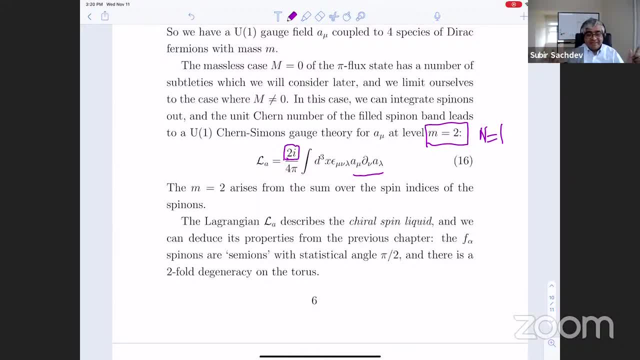 If you take two spin ons above the gap and you move them slowly around each other, in addition to the Fermi factor that you already have because they're fermions, you're going to get an additional Assistive tigal angle, which is pi by two. 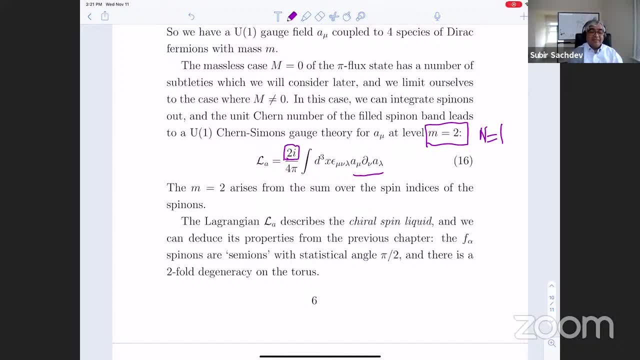 If you go back and look at our expression for the angle. Okay, These are called semi ons because they're halfway between a boson and a Fermi. on the statistical angle of a boson is zero for a Fermi on it's pi. 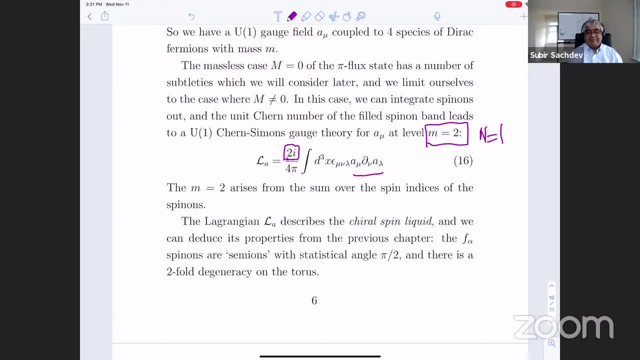 Uh, and so let's just think so. therefore, this is pi by two, or minus pi by two, depending on which way you go. Uh, so these are semi ons, and they all have the same specific angle: the particles. uh, and that's what the spin ons are. 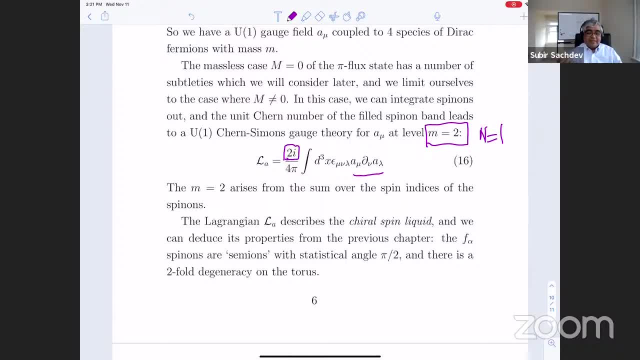 Now, if you take two semi ons and put them together, you get a boson Uh. so that's the only non-trivial uh, uh excitation. here It's the uh, not these semi ons. Yeah. 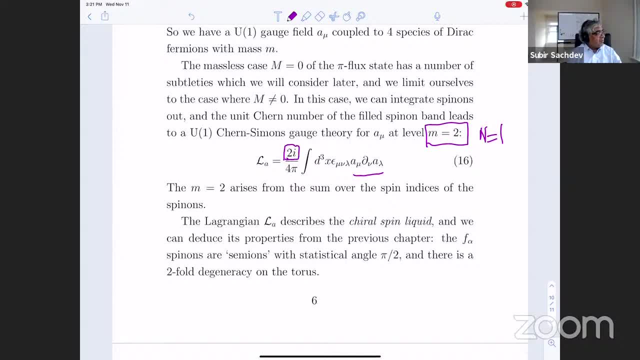 Okay, Sorry, Two semi ons should give you back a Fermi on. Uh, no, I know they do, but the fact, but. but the actual quasi particles here themselves are Fermi ons, Right. So how do you get back an actual? 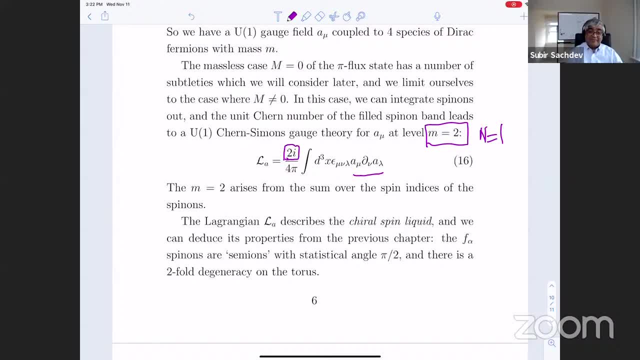 Right, No, this is a right, Sorry. This is a model of. This is a theory of spins. It's a theory of bosons, because the spin is just a Bose operator. Yeah, So this is a topological phase which can only appear in a theory of bosons. 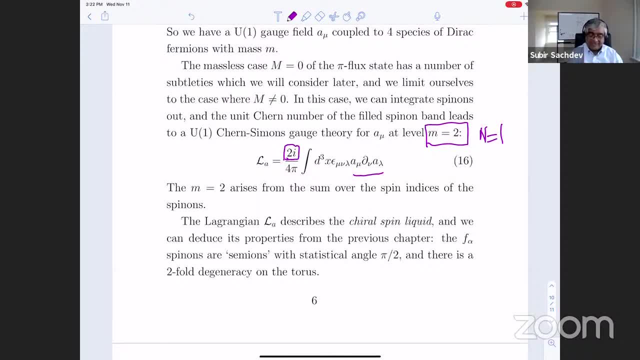 And here the boson of the spins offers their physical spin operator. Right, That's right, Thank you. You want to have both. the pool which I'm in, It's a boson TQ of T, but if you want to add a Fermi on you can times you one level one, but you should know you want to have a one. 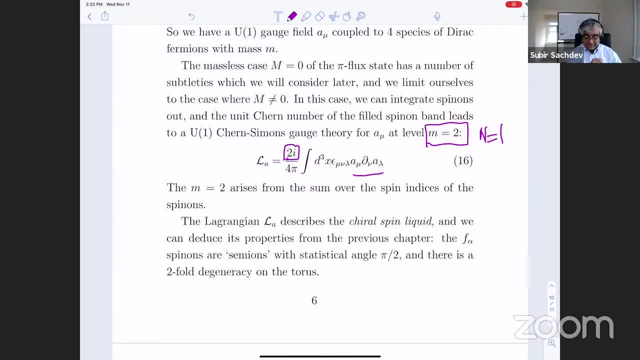 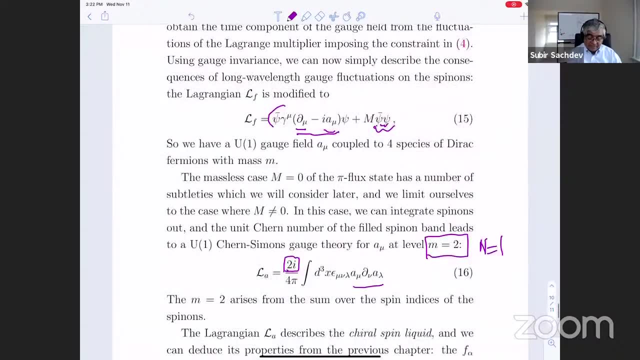 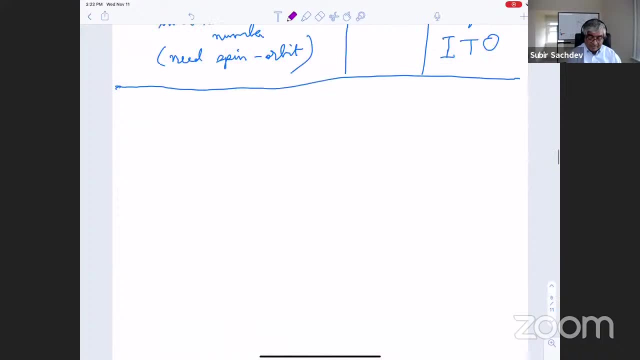 I hear you. Yeah, Thank you, That's right. So so two semi is make a boson, make a spin flip operator, because two F's make a spin flip operator. that we see already from you know from this decomposition from here. 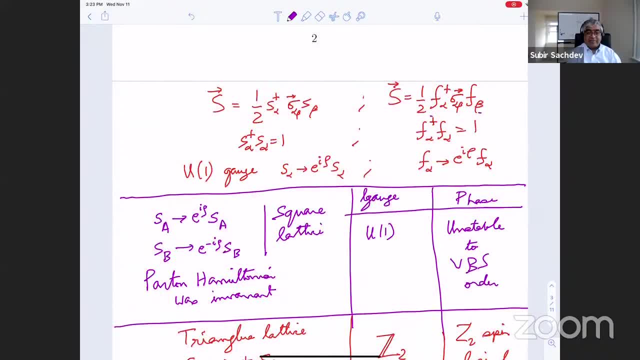 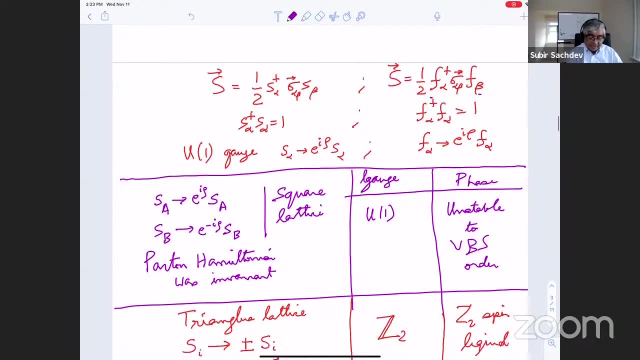 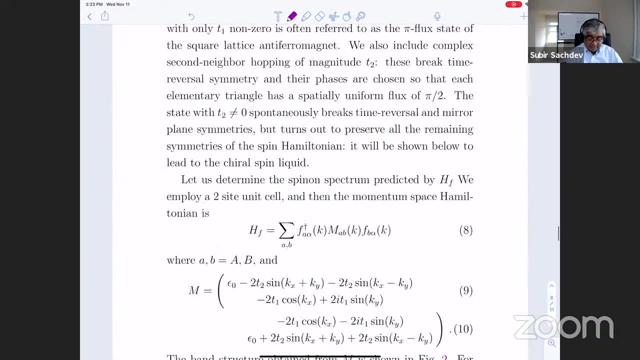 If you have two F's, then you get a spin operator. The spin operator is a boson, It's this capital B boson. So this is a theory of a bosonic, fractional, Fractalized state where the quasi particles are semi-ons. 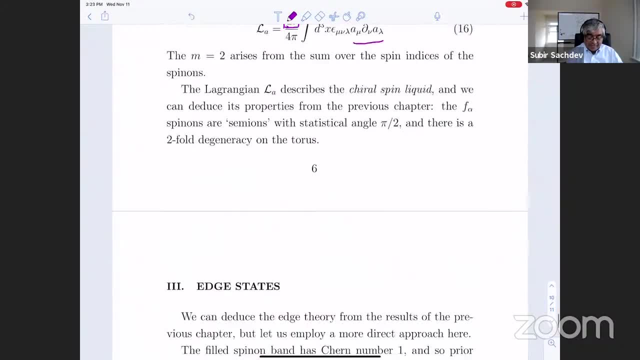 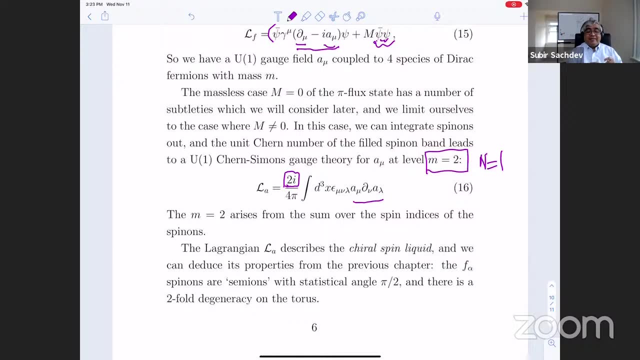 So the semi-ons, semi-ons, the spin-ons are neither neither bosons nor fermions, but the semi-ons, Okay. This is never. I mean this particular state I don't think has ever been seen in any experiment, but there have been a number of numerical studies of spin model which now show it. 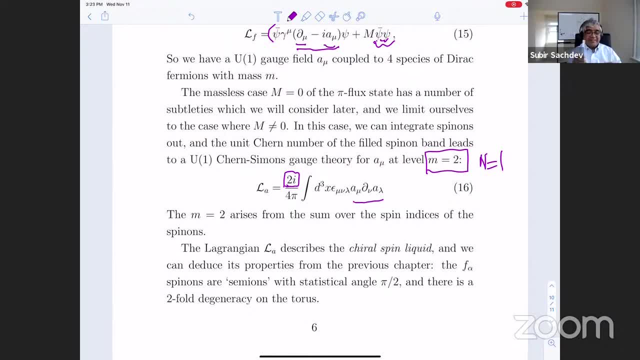 And let's see, you know what the future brings. I think the prospects are pretty good in the next, well, maybe in my lifetime. Okay Questions, All right. So now you know once I could just say, okay, I'm done. 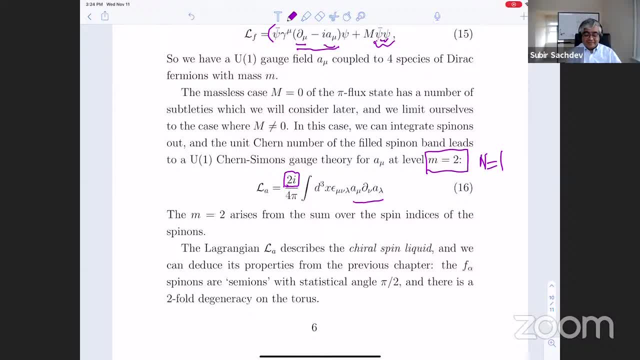 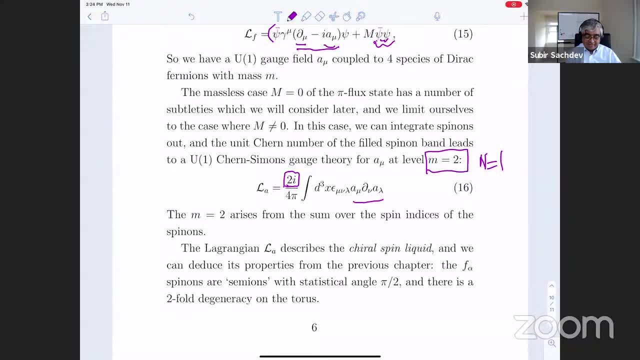 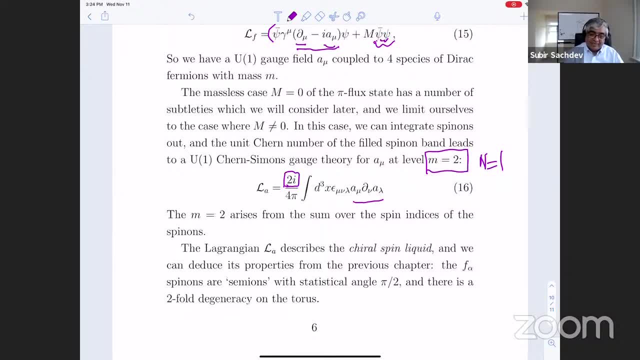 clarity. I'm going to try to proceed a bit further, not knowing all the things we learned about edge states. So let's try to do this, Try to understand the edge states of this theory on a microscopic basis. okay, so you remember, when we did the edge state theory, we had to make some postulate. we 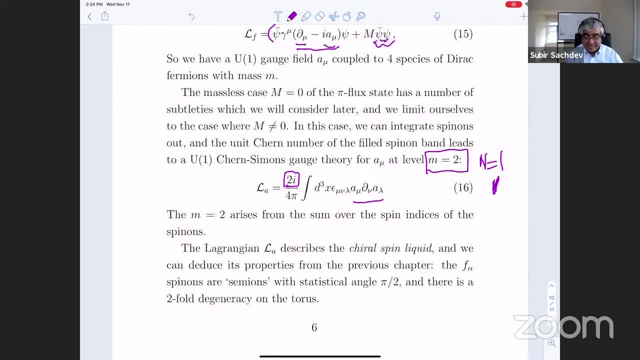 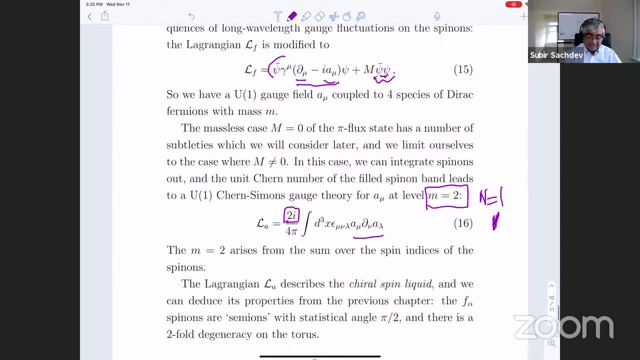 pulled out of our hat saying this is the only way to make the thing gauge invariant and therefore that must be the answer. we don't want to. we don't like such arguments. we want to actually just work out what happens on the edge of the sample. so suppose i had a sample with this band structure. 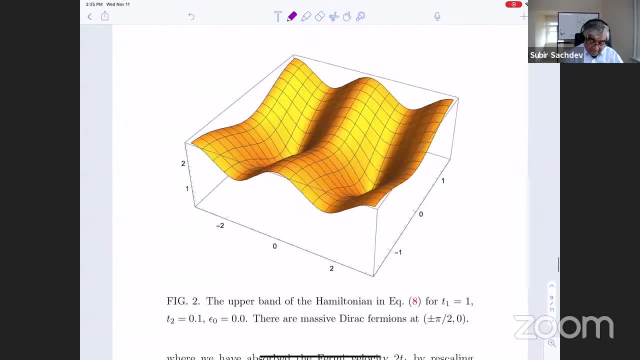 what's going on at the edge, okay, so let's just take a very naive point of view and try to figure this out. so you have a band, occupied band- i'm only showing the unoccupied band, but there's an occupied band with a churn number and for now let's even ignore the gauge. 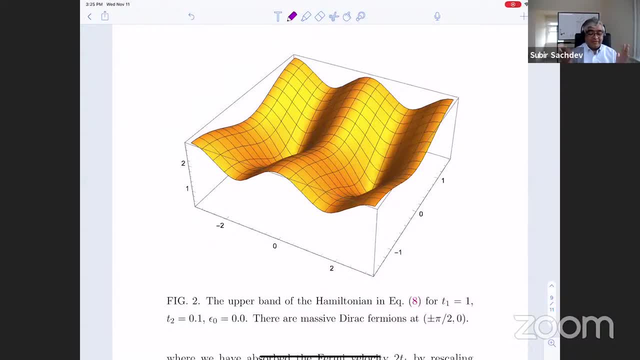 fluctuations. so what we know from the chapter integer, quantum hall effect, where we explicitly showed that every band with the churn number had an edge state. so, so there must be. and that edge state was just an ordinary freemium. okay, so so there must be an. 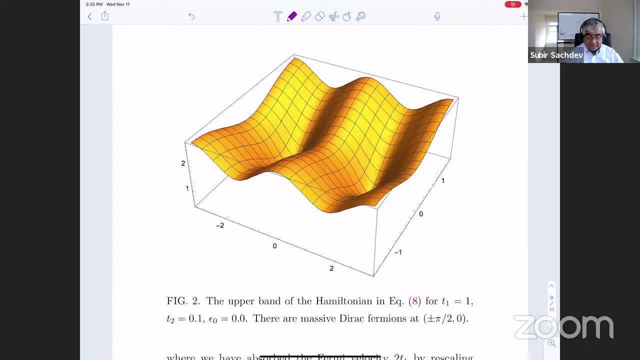 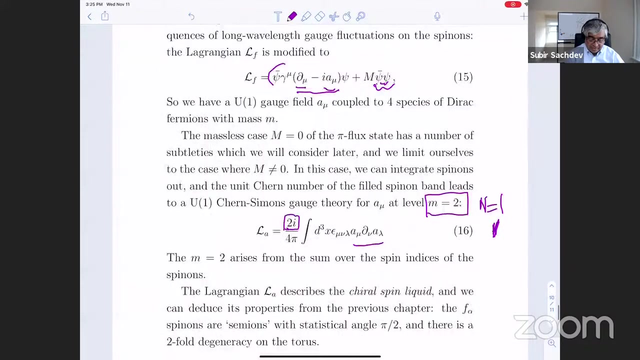 edge state here for the unoccupied, for the occupied churn band. but the important point is that there are two occupied churn bands- one would spin up and one would spin down, so each of them will give their own edge state. so that's what's going to happen. then i have these churn bands, okay, so i 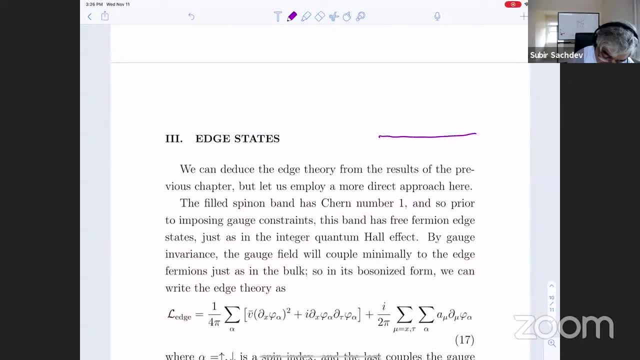 have a. this is the sample, this is the direction y, if i call it, and this is the energy, and i just have some occupied band in the center. well, it's so. these are the occupied states, and then i have a free. i have an edge state there. 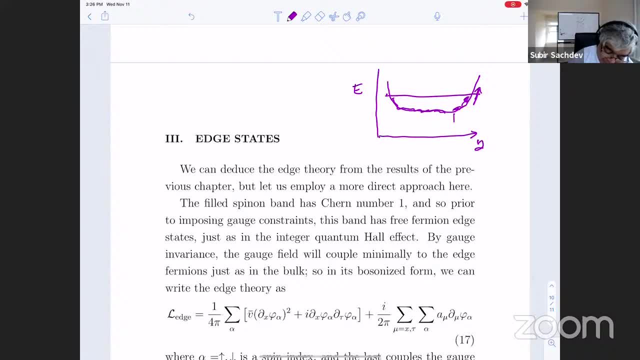 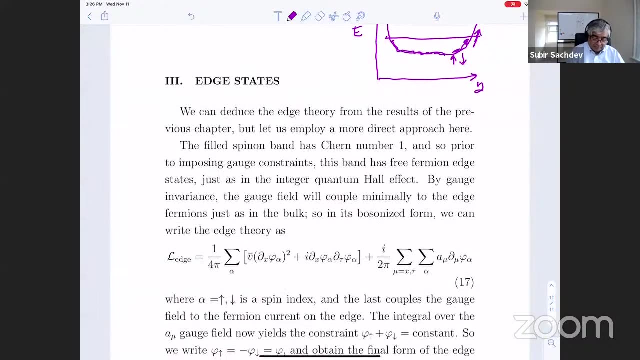 on this edge and that edge, and this happens for both spin up and spin down. so these are just free from your edge states. right now i'm just doing the mean field theory. so what is the theory of the edge? well, i already know that it's exactly this chiral boson with. 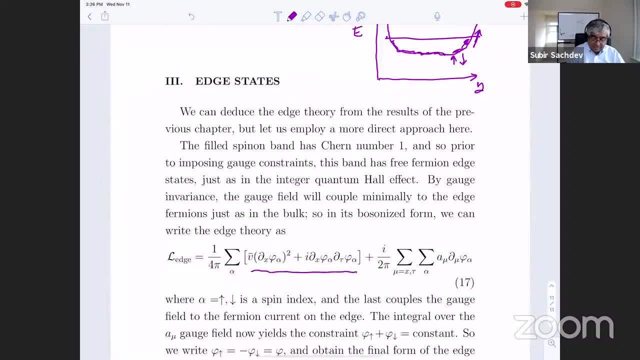 m equals one. so i have a upspin chiral boson and i have a downspin chiral boson. okay, all right, uh, but now how about the gauge fluctuations? so you know, this can't be the full theory, because we know in the bulk- uh, that wasn't the theory- what. 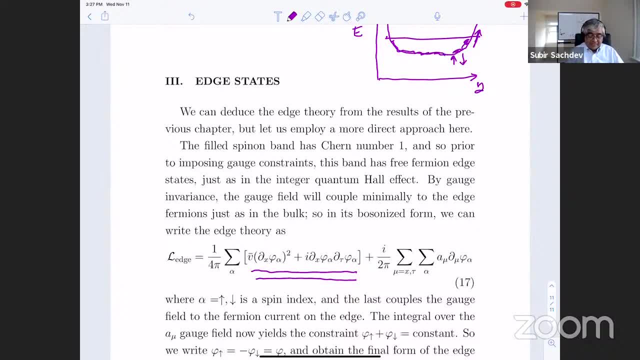 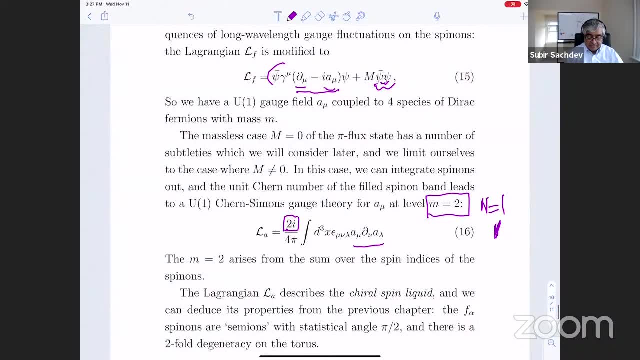 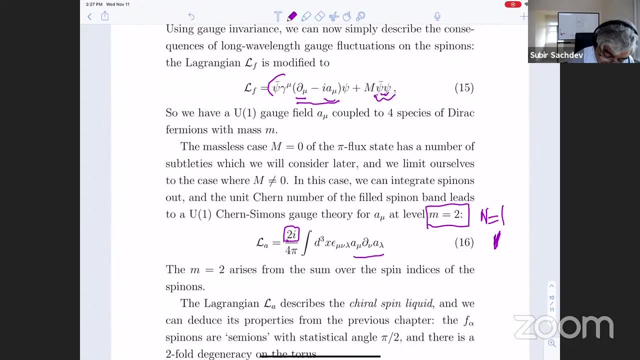 about gauge fluctuations. well, what do the gauge feel? so we have this internal gauge field which couples uh in the bulk to the fermion, uh to the, to the fermion current right. so the gauge field is coupling as you can see here. oh, but this is really much more general. this coupling here is: 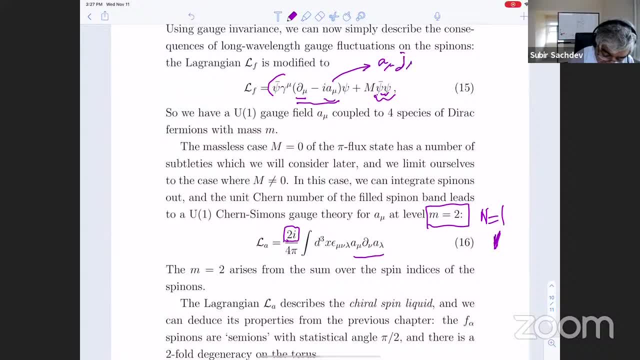 just a mu, j mu, and it just kind of follows from gauge invariance. that should be the coupling. uh, it's a mu times j mu, so therefore there should be a coupling even on the edge: uh, which couple? which couples a mu to the current of the fermions? 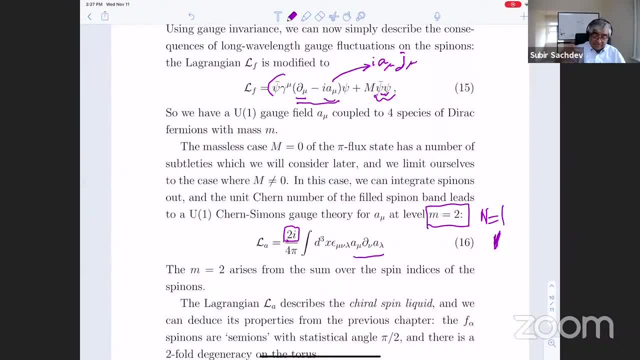 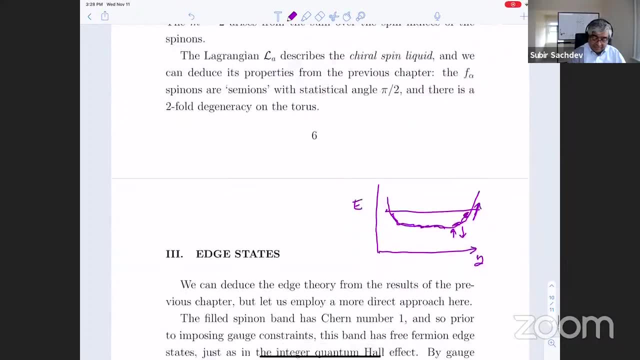 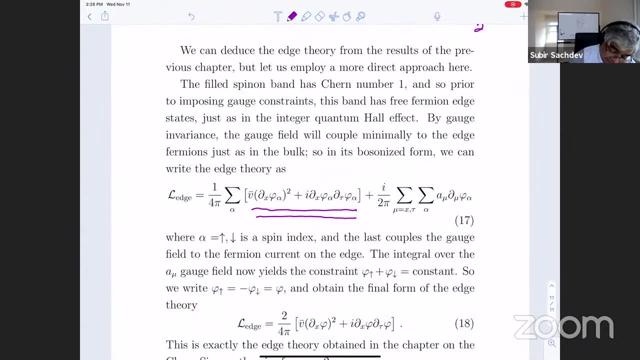 right, okay, so that's just again by gauge, invariance. so we had fermions on the edge. uh, you must have a coupling, uh, mu j mu. but what is the, the current on the edge? well, the current on the edge, uh, what we had learned was that the uh, uh, the epsilon union missing here. i'm not, i maybe miss. 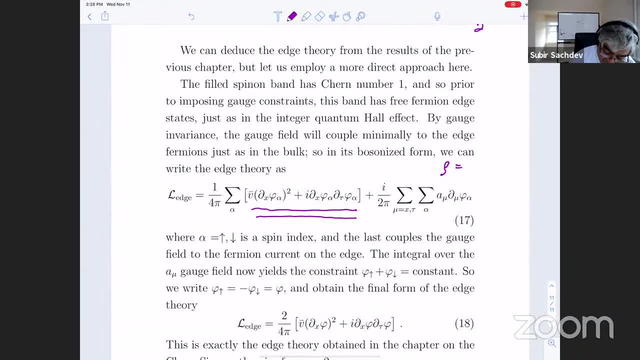 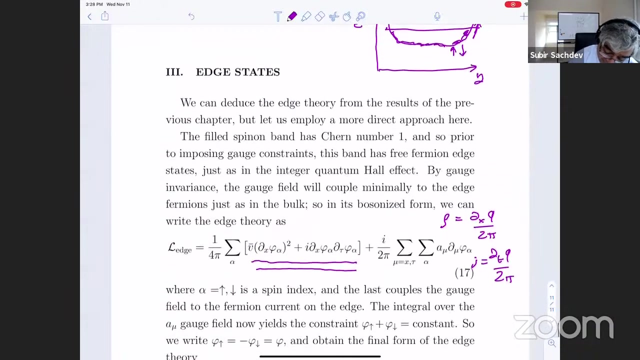 yeah, we learned that the density uh was um dx phi, yeah, dx phi, over two pi, and the current up to a sine was d tau d tau phi over two pi. so, therefore, and this, so the, the, the lawrence invariant current then is uh, so j mu, i should. i should make it write it out clearly one second. 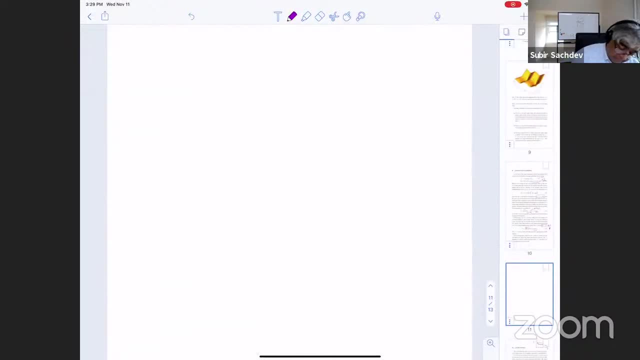 there all right. so on the boundary, we've learned from the postization formula. so the density of a carboson is del x phi over two pi. the current is g tau phi- i'm sloppy about factors- of i and minus one, two pi and therefore the current j mu. 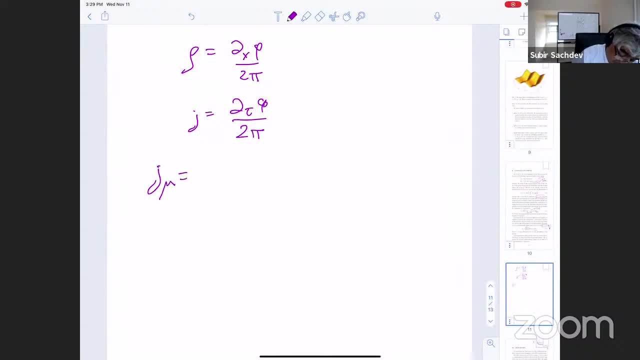 uh is okay. maybe there's a minus sign here. it's on the other side, the current, the epsilon mu nu del nu phi over two pi, that's the current of the boundary and that couples to a mu times j mu, that's the lagrangian, is a mu times j mu by gauge. 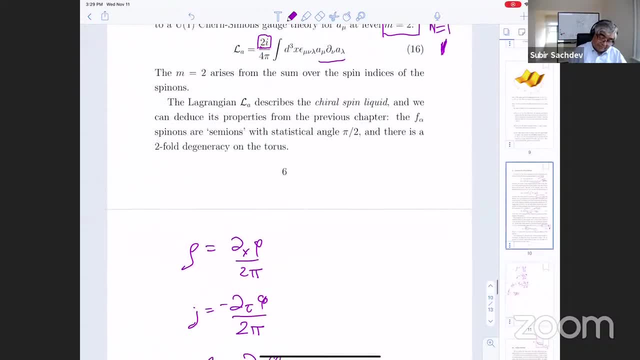 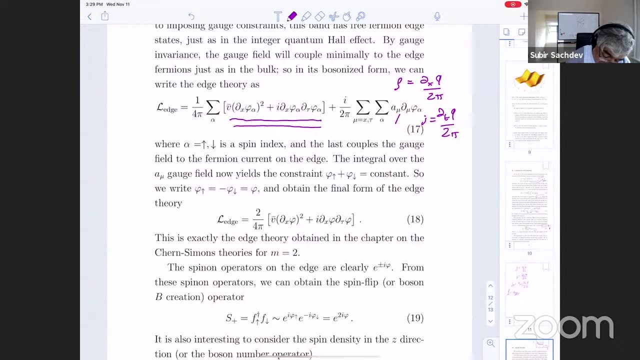 invariance. so therefore, oh yeah, i didn't write this correctly. here there's a typo. this should be a epsilon union factor here. i will fix that in the online. let me see, but it doesn't make much of a difference. all right, so now, and i have this gauge field that's fluctuating. 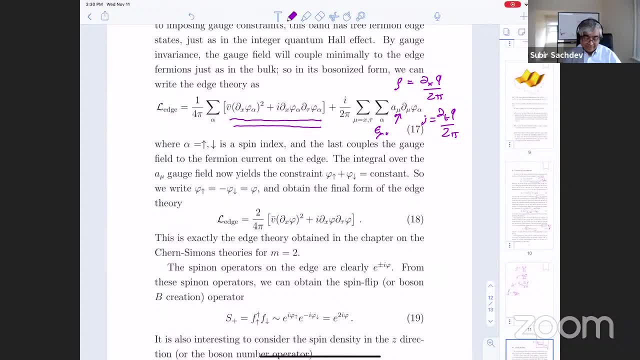 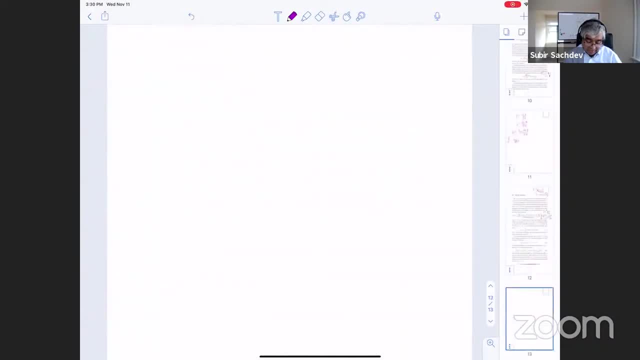 so what is? and it couples to the total current right. so, uh, the constraint. so this, you know the origin of this term is just the basic constraint on the microscopically. where did it go? yeah, microscopically, we have the constraint. we have the constraint that f dagger alpha, f alpha equals one. it's not the total density. 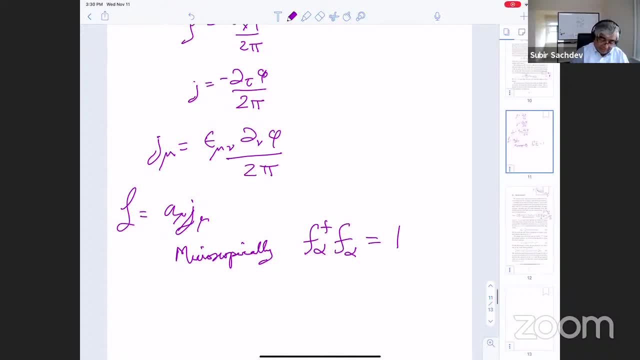 of fermions is not allowed to fluctuate. it's the sum on somewhat. alpha on every site is is one. so what this tells us on the edge when we integrate over the gauge fields, so when we integrate d a times e to the i, a, mu, j, mu over 2 pi, that's just a delta function that's going to give us a. 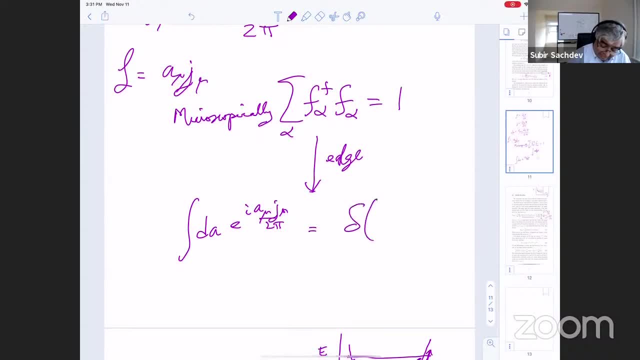 delta function and the function uh tells us that t mu, sum on alpha. again, someone spins sum on alpha, d mu is zero, meaning that there's no fluctuation in in in the total charge density. and that's exactly what it should be, because that's the constraint: the total number of firm. 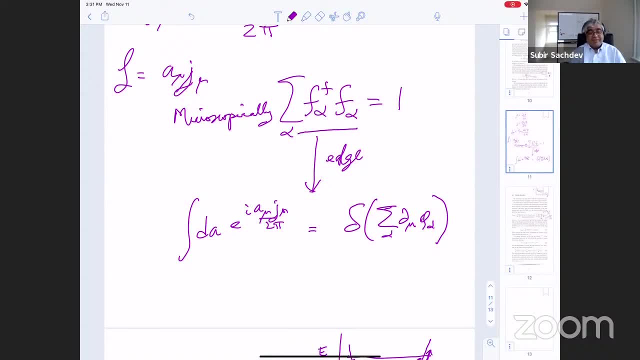 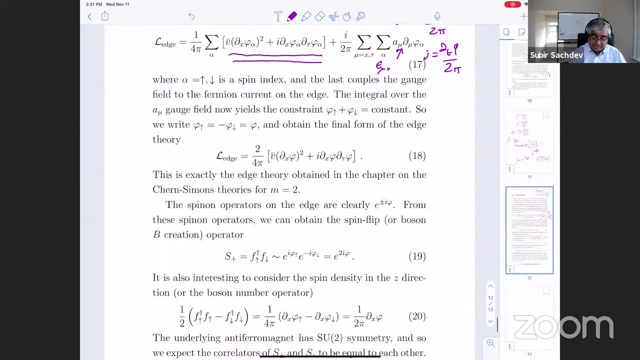 is not allowed to fluctuate, you're only allowed to make fermions from up to down and, quite remarkably, on this edge theory, this constraint is very easy to impose. exactly, you just put this delta function, so this tells us that you just have a delta function and say phi up plus phi down is a constant. 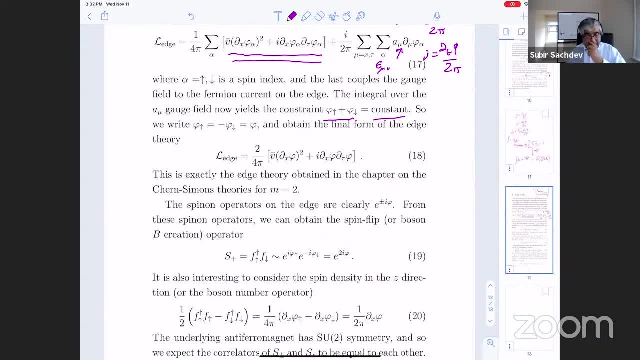 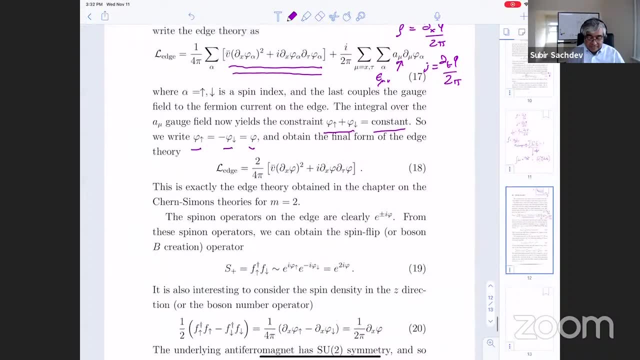 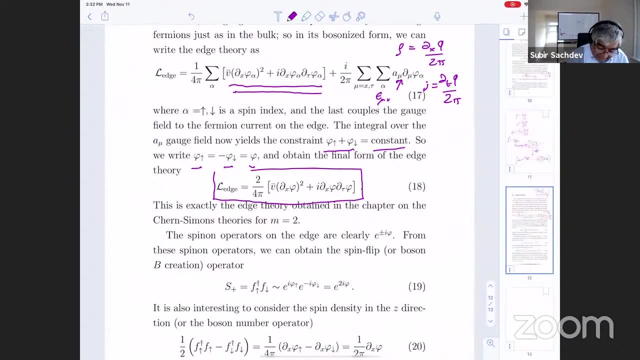 so constant doesn't matter. so you make that equal to zero, and so that means phi up is minus, phi down, which is phi. and now you plug this in here and you get your edge theory and you get the x theory with the famous factor of two. so now this was you know. hopefully it makes you happier about all the the tricks that we 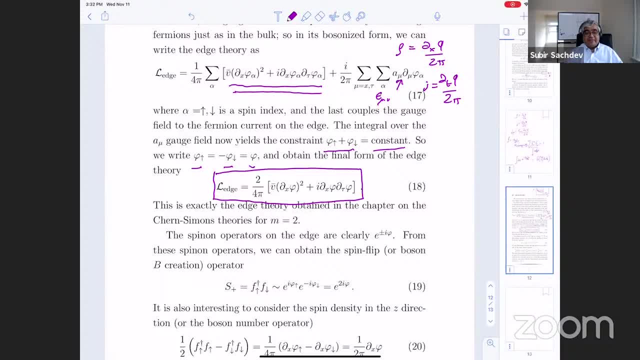 introduced in the chen simons gauge chapter where we just used gauge invariance to fix the edge. but now here we're, you know, just just doing the pad integral of the fermions in the bulk including the gauge field, and we go to the boundary and you integrate or put in the 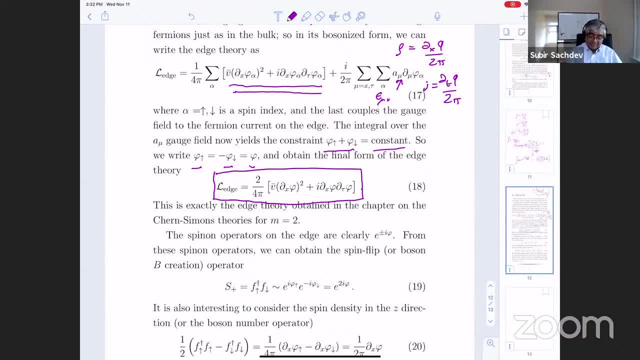 constraint on the gauge field. that gives you then the factor of two. so there it is. uh, so that's of course. we could have just got this answer from the previous chapter, but now i have a different derivation where i don't make any assumptions on some strange boundary conditions, like a tau equals zero that we used last time. 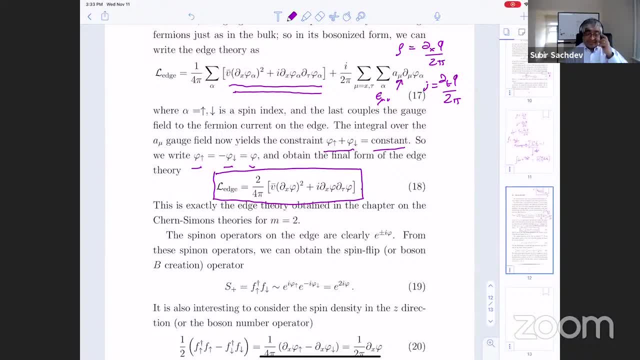 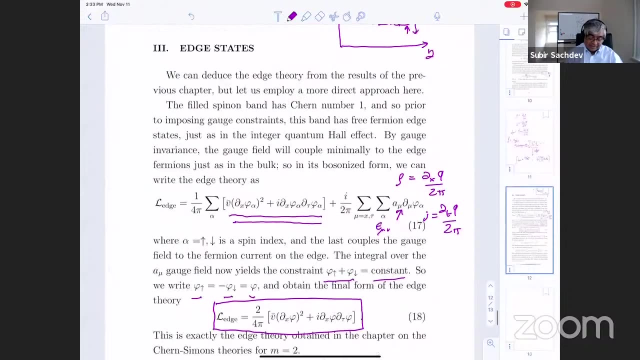 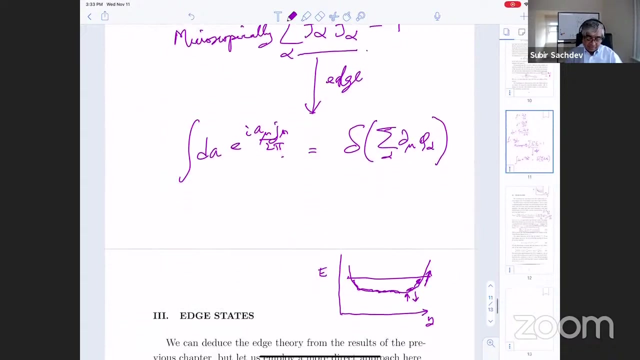 okay, um, yeah. so i i kind of really like this argument because it's one of the few cases where you know this complicated constraint, which we only treat approximately in all of these theories, we're able to treat exactly and it gives you a very in a very simple manner: just ties the two chiral bosons to each other. 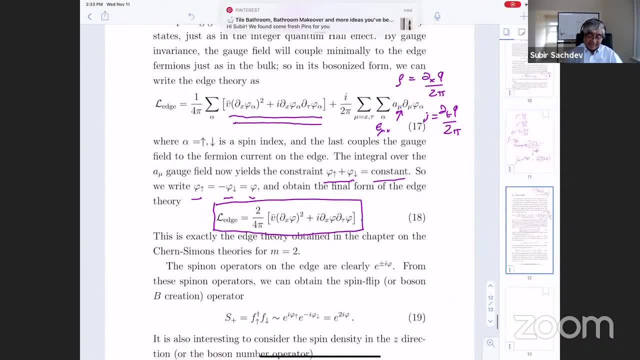 and it's, you know, it's this very strong interaction that's ultimately responsible, then, for this factor of two, and that's why this theory is completely different. it's, you know, but it's still gaussian, but it gives you rather more remarkable properties, including, uh, the semionic statistics. 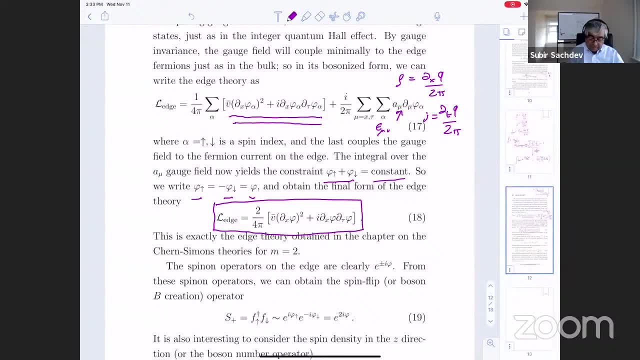 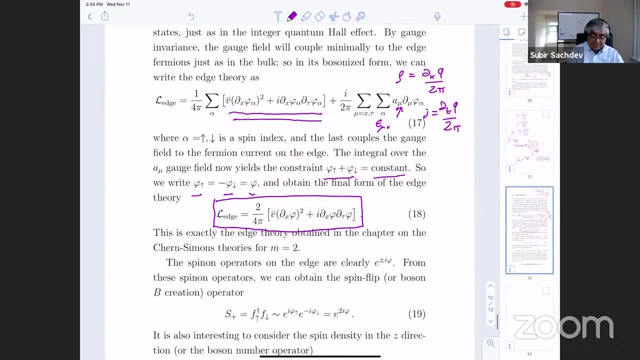 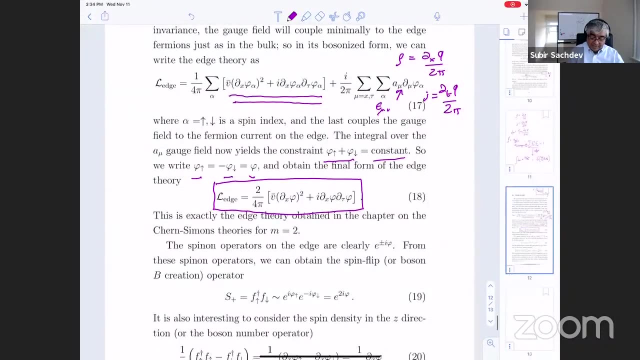 um, okay. so now of course we know the, the quasi-particle operators. in the bulk they were just fermions, and we already know that the fermions are just e to the i phi, uh, in the bosonization language, and therefore the spin on becomes plus or minus i phi on the boundary. 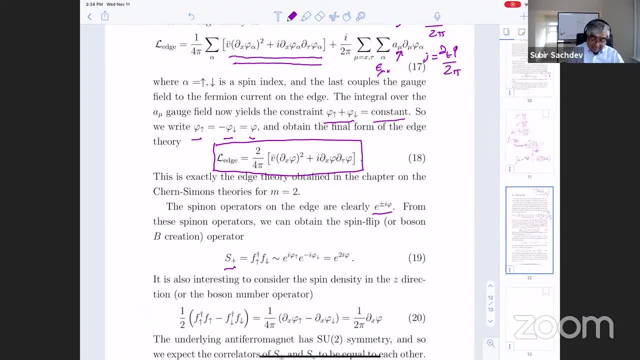 and the spin flip operator, like i said, gives you e to the two i phi, because if one is phi up and the other is phi down, they have opposite signs and you get two i phi. another interesting operator to consider is the spin density, not the total density, but 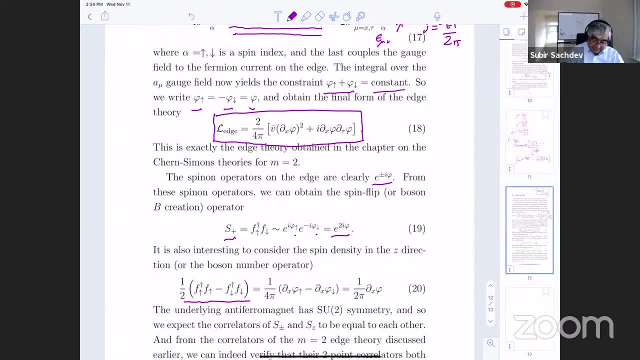 the difference in density of the fermions. well, that's this difference, including that factor of one half, and that gives you a one over two pi gradient of phi. okay, so now there might be one thing that's kind of bothering you: perhaps the underlying system we started with had an su2 symmetry. 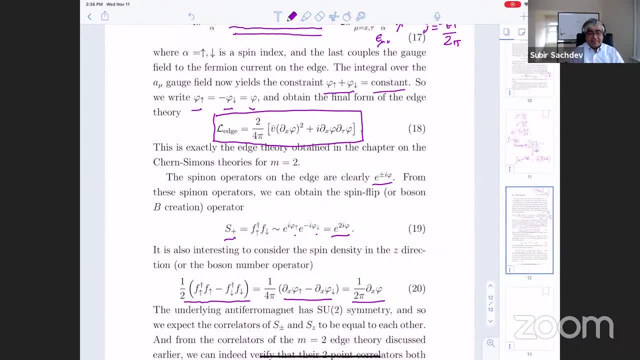 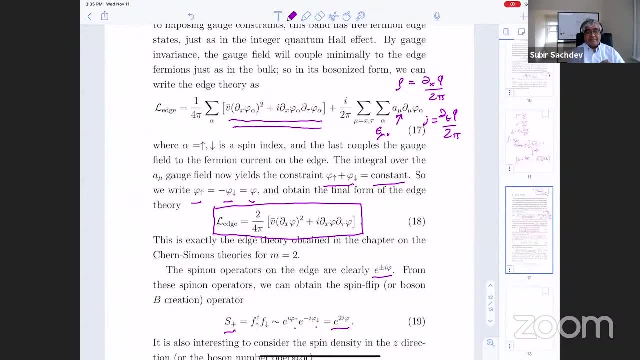 and of spin rotations. but when we did the bosonization of the boundary theory we broke that su2 symmetry. we treated spin up and spin down with two separate chiral bosons. so in fact we no longer have the su2 symmetry in this theory. but if things were right, 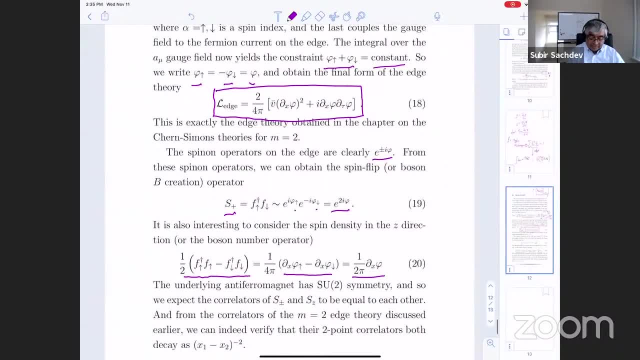 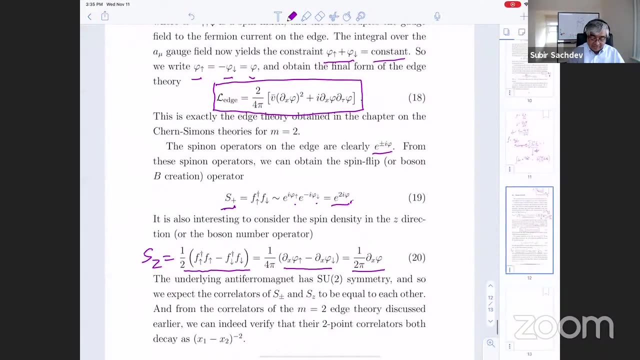 you should find, uh, that the physical operators like s plus and s, my s plus and s z- so this is s z- should have the same correlation functions, but they look very different. one is e to the two i phi and one is one over two pi grad x phi. 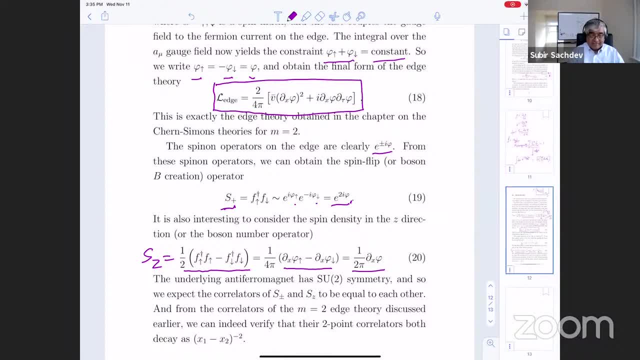 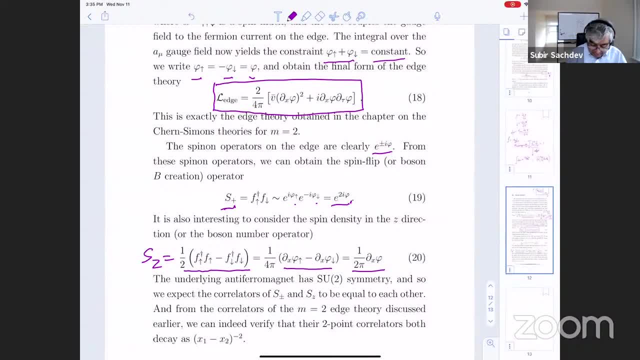 they both give you exactly the same answer. so this, this theory here, this chiral boson theory, which looks like a u1, it has a u1 global symmetry. so this is the u1 cosmology algebra at level two. secretly, it has an su2 symmetry. 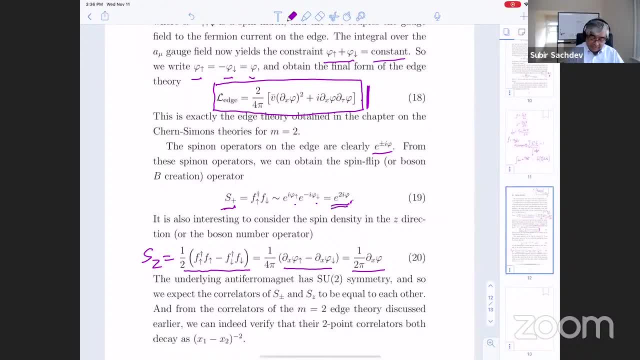 and that su2 symmetry is associated with these operators, e to the two i, phi and one over two pi, grad x, phi having the same correlation function. so, in fact, even though you broke the su2 symmetry, uh in the bosonizing the theory, in the end you can recover. 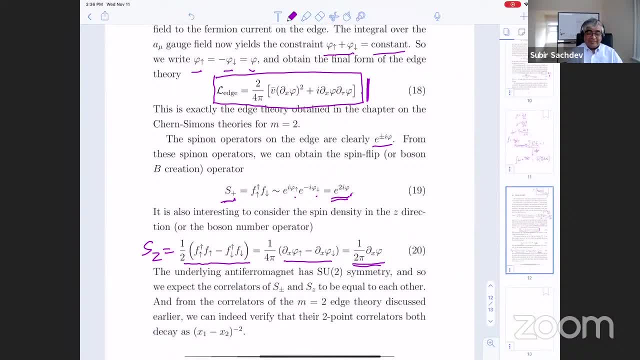 now there's another way to do all of this, using an approach that maintains su2 symmetry at all times. that involves an su2 gauge field in the bulk and non-obelian bosonization on the boundary. uh so, and that's also a very powerful technique, which is useful in other cases. 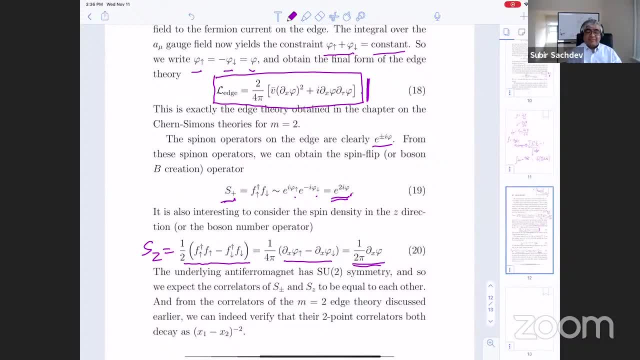 but here we can actually get all the answers we need just by using abelian bosonization. is this related to the, to the, to the level ranked? equality, level ranked only? no, i don't think so. this is just if you take the c equals one, uh theory at certain points, at certain. 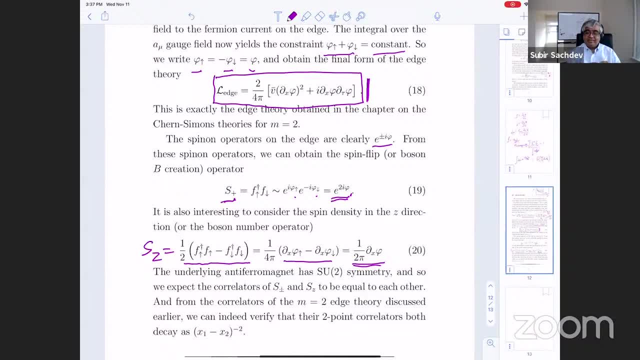 radii of the c equals one theory. there's extra symmetries. if you just you know, if you look at the lookup- kid sparks lectures on conformal field theory- then you find that central charge c equals one, has many different, uh, many different cfts and at some points there, even though the 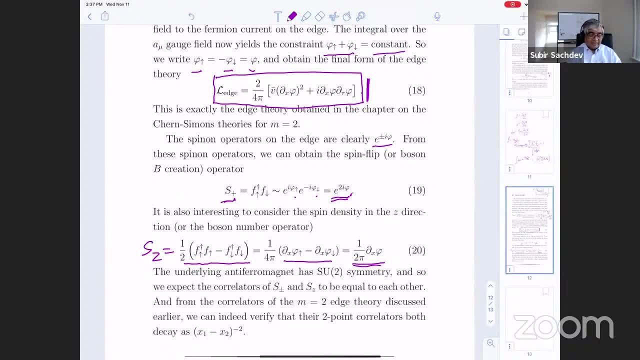 explicit symmetry is only u1. the correlators all have and all the operator spectrum has an su2 symmetry. yeah, i don't think. level rank duality is a more complicated thing for non-obby engaged theories. maybe it's connected, i don't know. maybe it's connected, i don't know. 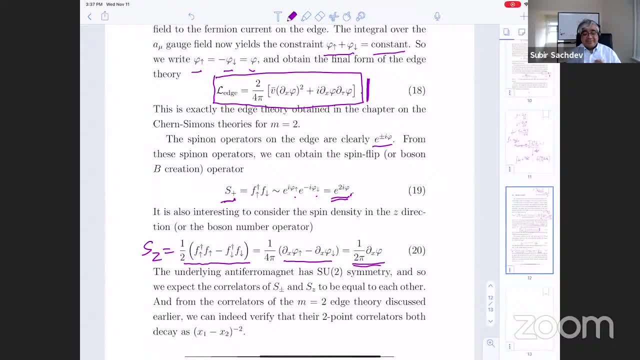 maybe it's connected, i don't know. maybe you can derive it in some way, but maybe you can derive it in some way. but maybe you can derive it in some way, but not that i know of okay, other questions, okay. so now you know, let's move on, we can. 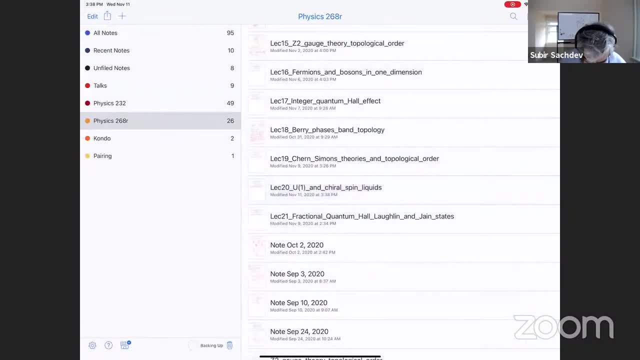 okay, so now you know, let's move on. we can. okay, so now you know, let's move on. we can do the next chapter, do the next chapter, do the next chapter. we have all this powerful technology. let's, we have all this powerful technology. let's, we have all this powerful technology, let's apply. finally, then, 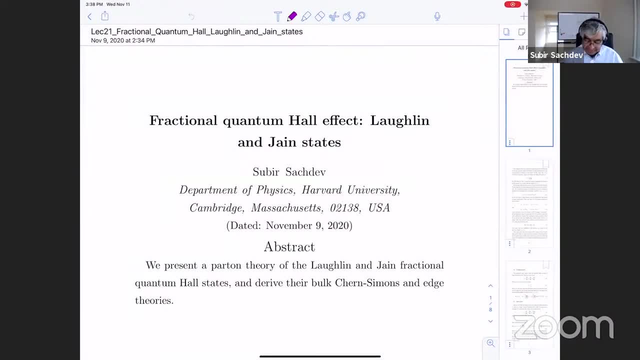 apply, finally then apply, finally then, uh, the famous corner fractional quantum, uh, the famous corner fractional quantum, uh, the famous corner fractional quantum hall states. let's apply this hall states. let's apply this hall states, let's apply this, let's use this approach, uh, to get, and some understanding of the fractional 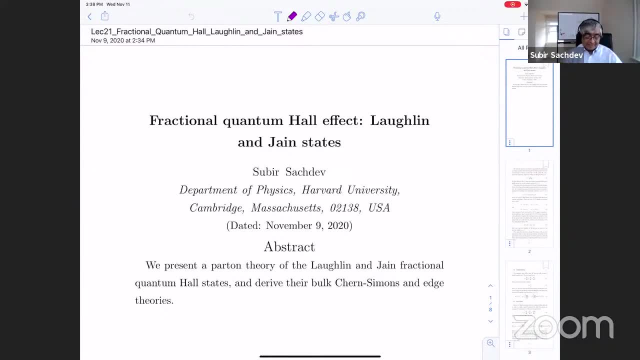 and some understanding of the fractional and some understanding of the fractional quantum hall states. quantum hall states, quantum hall states, which are of course the one, the topological, which are of course the one, the topological, which are of course the one, the topological states that are best studied. 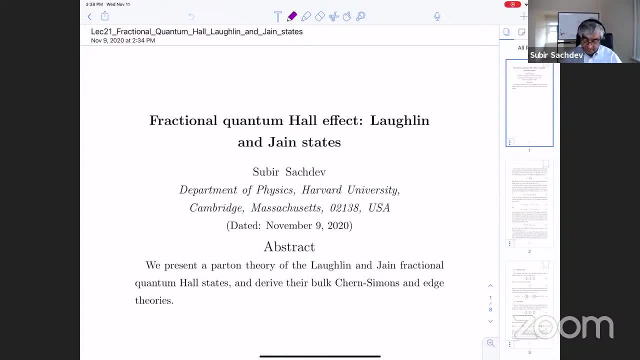 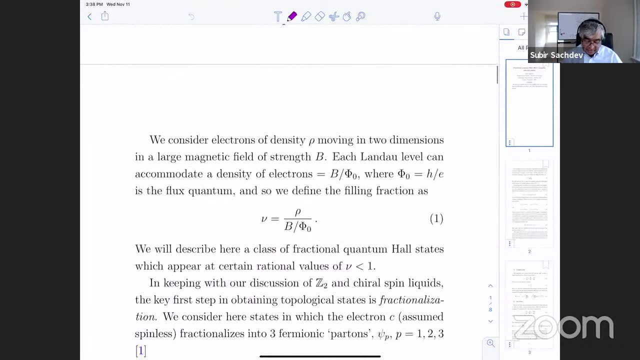 states that are best studied, states that are best studied experimentally. okay, okay, so, um just to review, you get the. so um, just to review, you get the. so um just to review, you get the fractional quantum hall effect. fractional quantum hall effect. fractional quantum hall effect. uh, here, let's just take the end all. 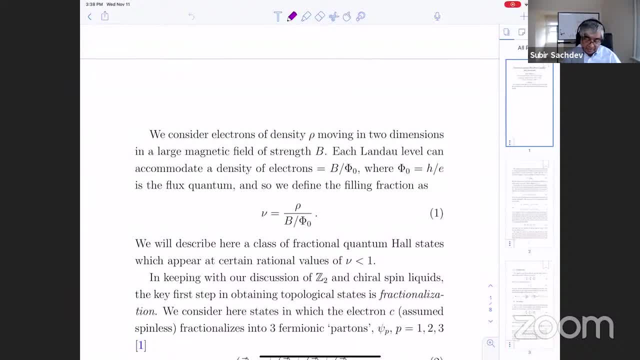 uh here, let's just take the end. all uh here, let's just take the end. all levels, levels, levels. so we consider electrons are some. so we consider electrons are some. so we consider electrons are some density: rho in two dimensions in a very density. rho in two dimensions in a very 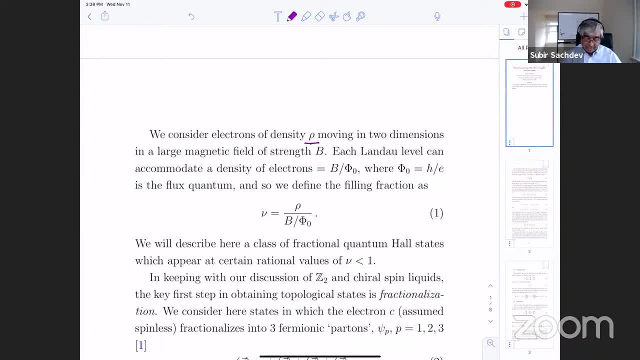 density, rho in two dimensions in a very large magnetic field. large magnetic field, large magnetic field. so you get a bunch of landau level in. so you get a bunch of landau level in. so you get a bunch of landau level in the magnetic field b. 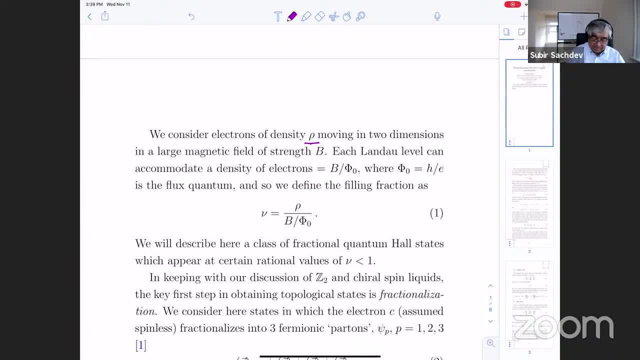 the magnetic field b. the magnetic field b, uh and each landau levels. the density of uh and each landau levels. the density of uh and each landau levels. the density of electrons: you can electrons, you can. electrons, you can, you can accommodate, you can accommodate, you can accommodate. is b over phi naught. so that's the. 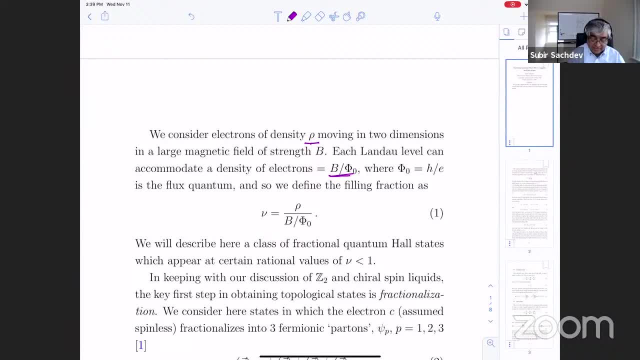 is b over phi naught, so that's the is b over phi naught. so that's the fully filled landau level, but the density fully filled landau level, but the density fully filled landau level, but the density equals b over phi naught. equals b over phi naught. 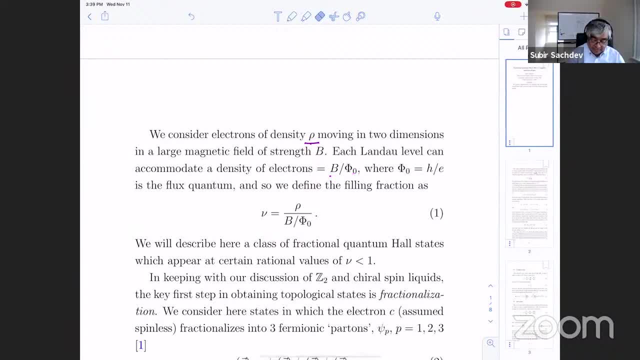 equals b over phi naught, where phi naught is the filling fraction. where phi naught is the filling fraction. where phi naught is the filling fraction um, um, um. phi naught is the flux quantum, excuse me. phi naught is the flux quantum, excuse me. 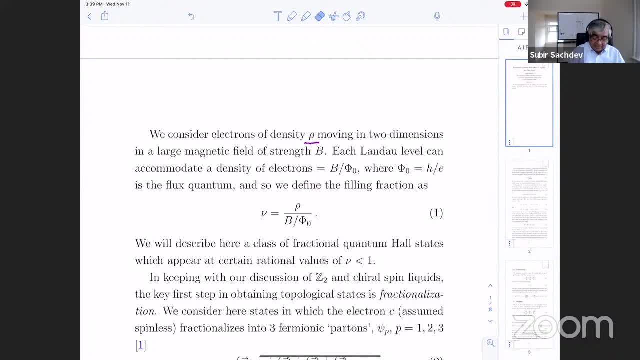 phi naught is the flux quantum, excuse me. so if the landau level is partially so, if the landau level is partially so, if the landau level is partially filled, filled, filled, then you get, then you get, then you get a filling fraction which is defined by the. 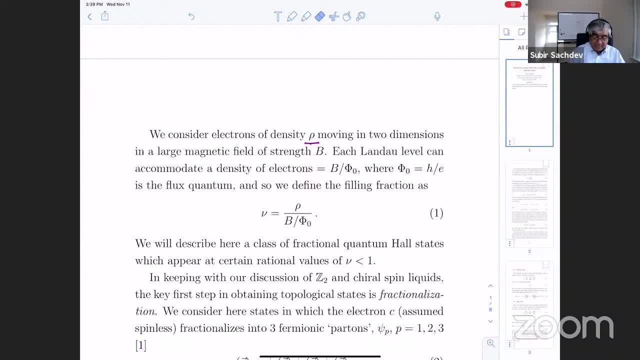 a filling fraction which is defined by the. a filling fraction which is defined by the ratio of the density ratio of the density ratio of the density of the electrons to the magnetic field, of the electrons to the magnetic field of the electrons to the magnetic field, and the remarkable experimental 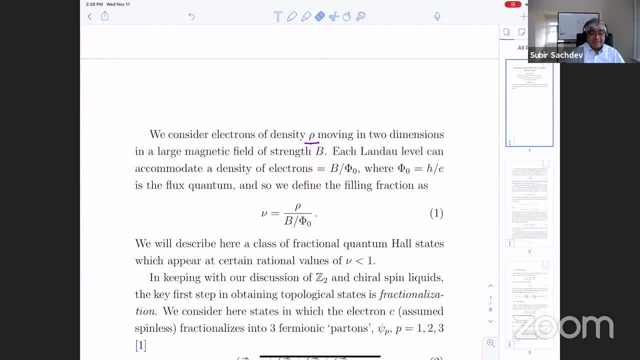 and the remarkable experimental. and the remarkable experimental observation which was experimentally observation, which was experimentally observation, which was experimentally in theoretically complete surprise, in theoretically complete surprise, in theoretically complete surprise, was that at certain all was that at certain all was that at certain all, what was first observed, for example at 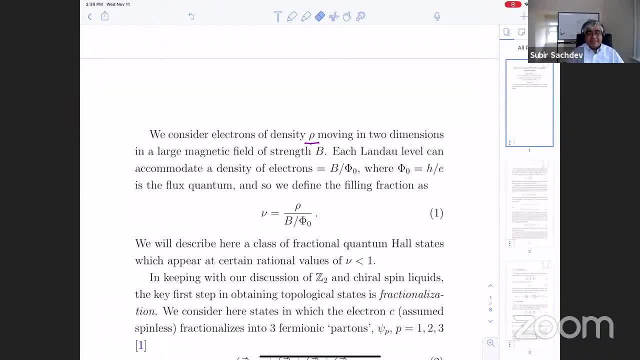 what was first observed, for example, at. what was first observed, for example, at: nu equals one-third. nu equals one-third, nu equals one-third. you had a gap state. you had a gap state. you had a gap state with the whole conductivity there was. with the whole conductivity there was. 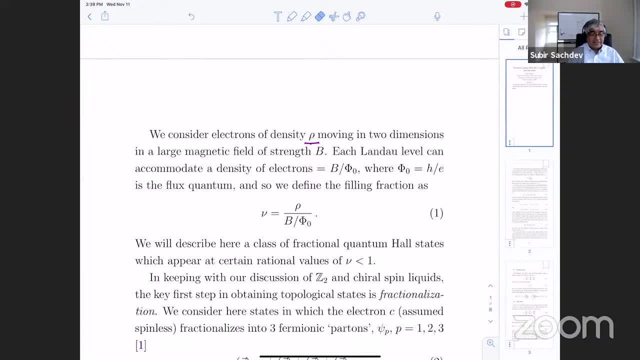 with the whole conductivity, there was one third of uh e squared over h. one third of uh e squared over h. one third of uh e squared over h. um. so sigma x y was one new times e? um. so sigma x? y was one new times e. um. so sigma x y was one new times e squared over h when new is the filling. 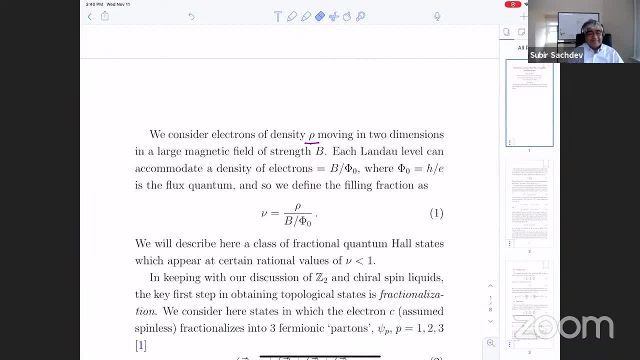 squared over h when new is the filling: squared over h when new is the filling fraction of one third, and this was a fraction of one third, and this was a fraction of one third, and this was a plateau and uh, plateau and uh, plateau and uh, and you know, and that too, so a lot of. 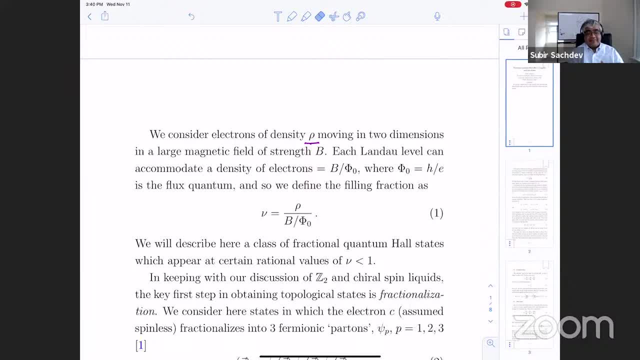 and you know, and that too so a lot of, and you know, and that too so a lot of remarkable developments, remarkable developments, remarkable developments. so the first theory of this uh came from. so the first theory of this uh came from. so the first theory of this uh came from laughlin. 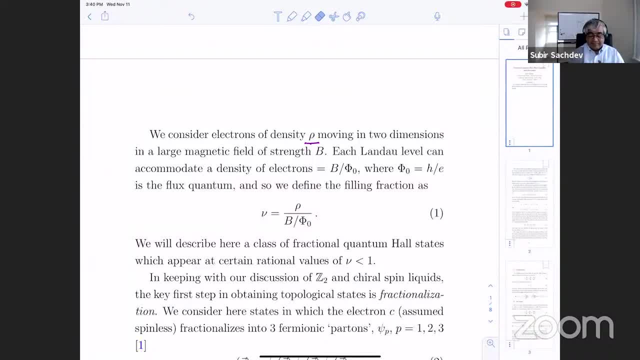 laughlin, laughlin, uh, where he proposed a uh, where he proposed a uh, where he proposed a of trial wave function, which explained of trial wave function, which explained of trial wave function, which explained a lot of things, a lot of things, a lot of things. and from that trial wave function, people 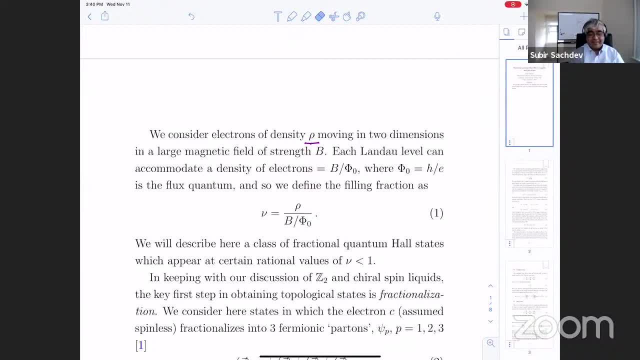 and from that trial wave function people and from that trial wave function people you know, understood the connection to you know, understood the connection to you know, understood the connection to john simon's gauge theories and many john simon's gauge theories and many john simon's gauge theories and many, many other things. 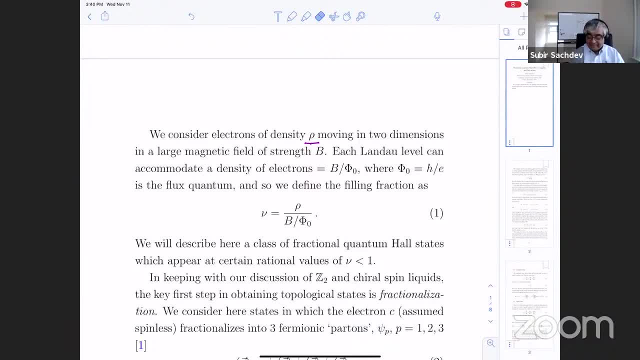 many other things, many other things, uh, and you can, starting from that wave, uh, and you can, starting from that wave, uh, and you can, starting from that wave, function, you can derive a lot function. you can derive a lot function. you can derive a lot now. that's, you know, described in so many. 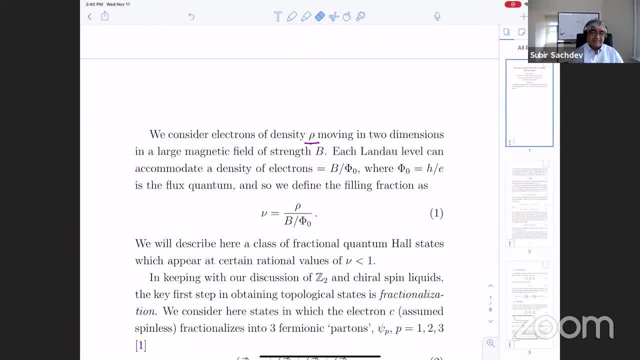 now that's you know described in so many, now that's you know described in so many books and review articles that uh, i'm books and review articles. that uh, i'm books and review articles. that uh i'm which i imagine you can read, which i imagine you can read. 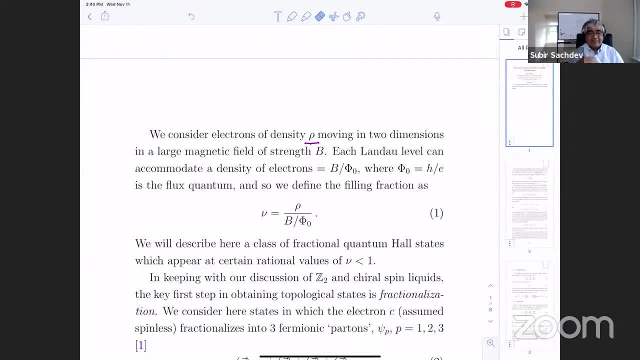 which i imagine you can read. so i'm not going to take the historical. so i'm not going to take the historical, so i'm not going to take the historical development. i'm just going to describe development. i'm just going to describe development. i'm just going to describe this. 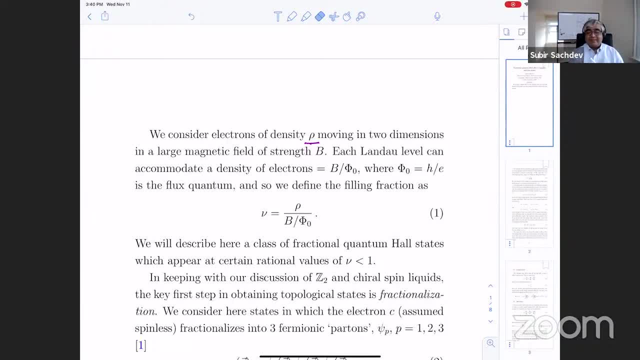 this, this by the approach we've been using, which is by the approach we've been using, which is by the approach we've been using, which is the part on construction, the part on construction, the part on construction, and from the part on construction you can, and from the part on construction you can. 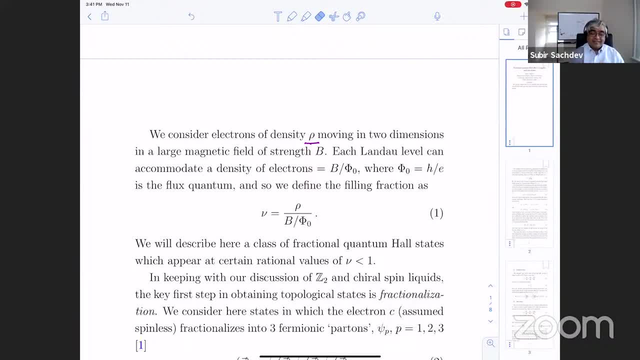 and from the part on construction, you can even write down and deduce laughlin's, even write down and deduce laughlin's, even write down and deduce laughlin's wave function, wave function, wave function. but more powerfully you can deduce the. but more powerfully you can deduce the. 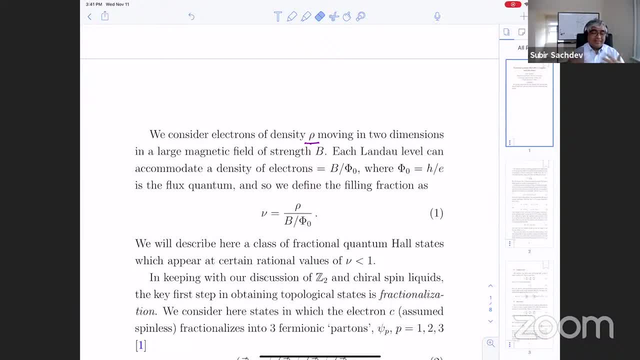 but more powerfully you can deduce the edge state theory, the bulk theory, the edge state theory, the bulk theory, the edge state theory, the bulk theory, the fractional statistics. everything comes fractional statistics, everything comes fractional statistics. everything comes out very naturally, out very naturally, out very naturally, in a way. 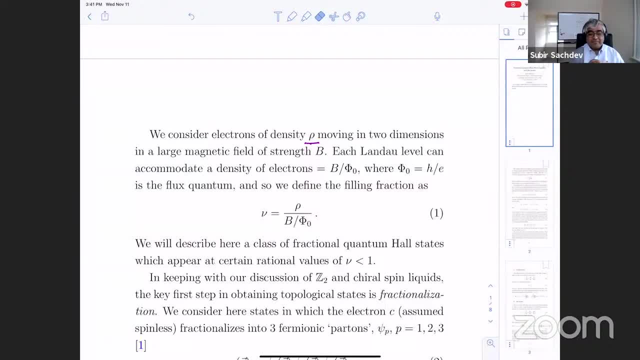 in a way, in a way very similar to what we just did for the, very similar to what we just did for the, very similar to what we just did for the chiral spin liquid. so what's the basic idea? so the basic. so what's the basic idea? so the basic. 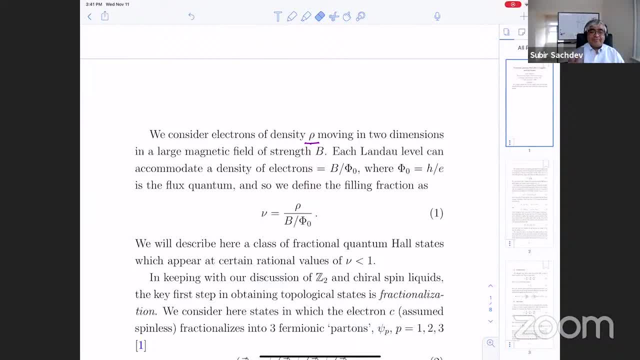 so what's the basic idea? so the basic idea, idea, idea of the partons, is to split the particle of the partons is to split the particle of the partons is to split the particle up, in this case the electron which is the up, in this case, the electron which is the. 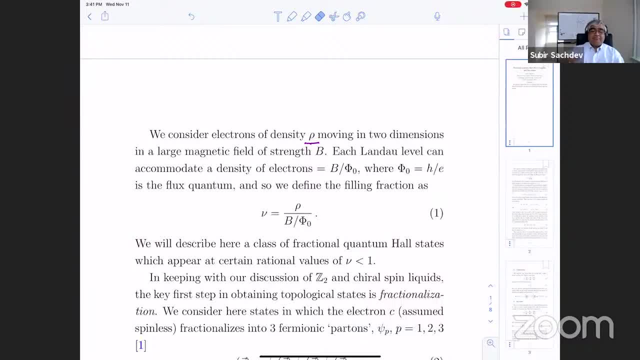 up, in this case the electron, which is the physical particle, physical particle, physical particle into parts, into parts, into parts, and it turns out that for the laughlin, and it turns out that for the laughlin, and it turns out that for the laughlin state and also for 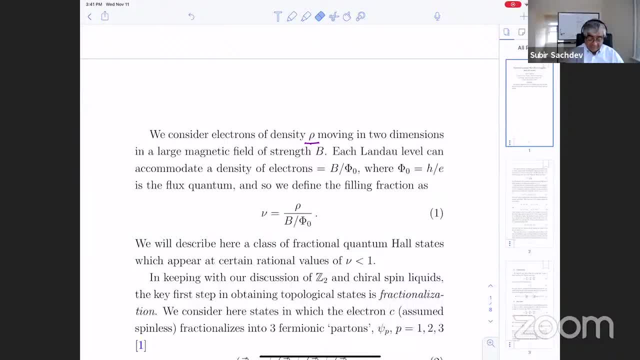 state, and also for state and also for the jane states. as we'll see, it is the, the jane states. as we'll see it is the, the jane states. as we'll see, it is the main sequence of jane states, main sequence of jane states, main sequence of jane states. the division we're going to make is not 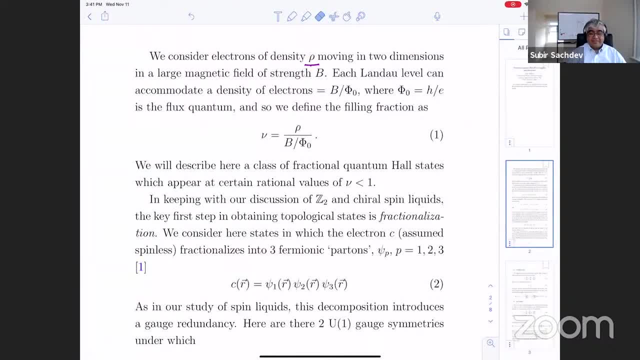 the division we're going to make is not. the division we're going to make is not split it into two. split it into two. split it into two, which is what we've done so far, but into which is what we've done so far, but into which is what we've done so far, but into three. 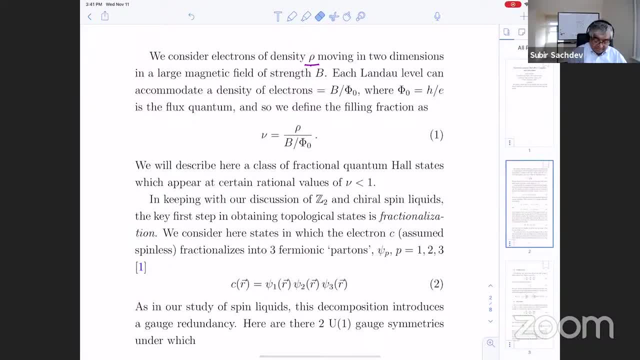 three, three. we take our electron and split it into. we take our electron and split it into. we take our electron and split it into three patterns. okay, so if i draw a picture, okay, so if i draw a picture, okay, so if i draw a picture, um, just to make this pictorial, 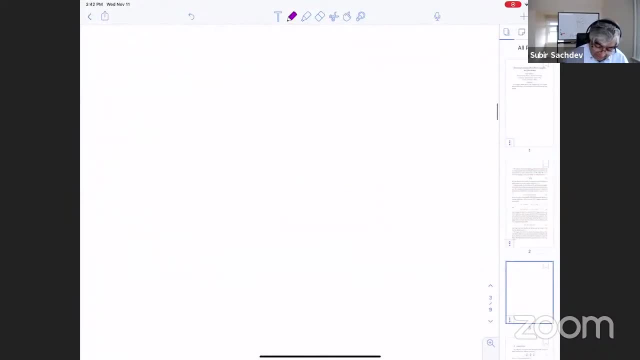 yeah, yeah, yeah. so you have your sample and in the sample. so you have your sample and in the sample. so you have your sample and in the sample, um, um, um, you have some particles here. are you have some particles here? are you have some particles? here are particles sitting in your sample. 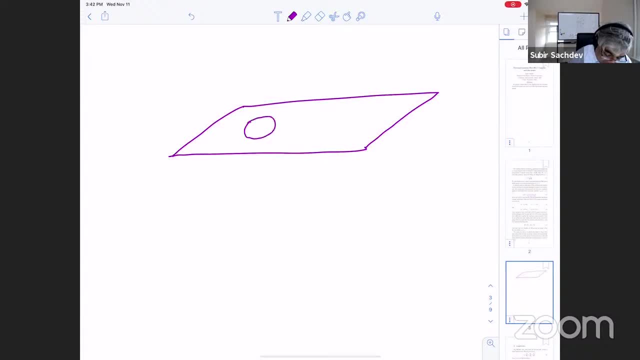 so here's your electron and you are filling one third. so there, and you are filling one third. so there, and you are filling one third. so there are three flux quanta, are three flux quanta are three flux quanta for each particle. so i'm going to clump. 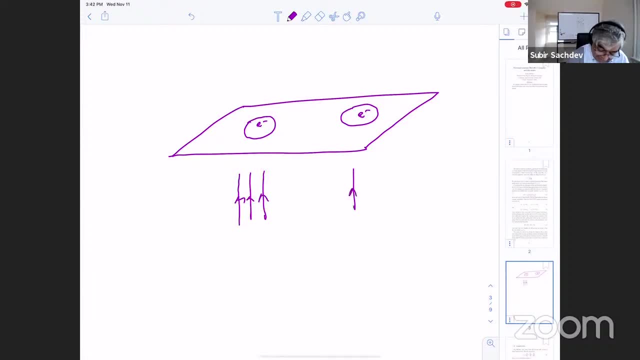 for each particle. so i'm going to clump for each particle. so i'm going to clump them up, just them up, just them up, just to make a picture. this is the physical to make a picture. this is the physical to make a picture. this is the physical magnetic field. 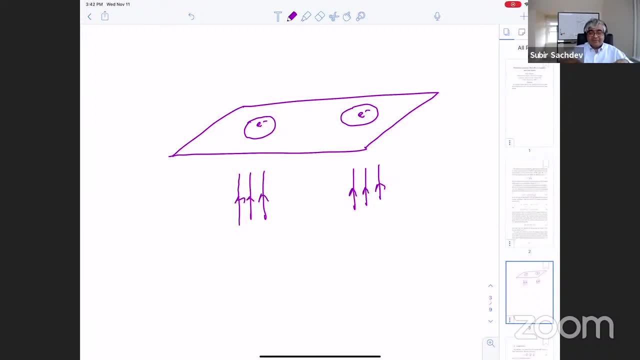 magnetic field. magnetic field. so for each electron there are three flux. so for each electron there are three flux. so for each electron there are three flux: quanta coming in. quanta coming in. quanta coming in, because you have nu equals one third. because you have nu equals one third. 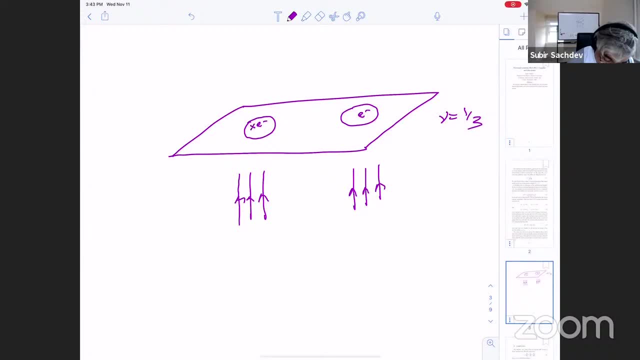 because you have nu equals one third. so what i'm going to say is that the so what i'm going to say is that the so what i'm going to say is that the electron, electron, electron is actually made up of three particles, is actually made up of three particles. 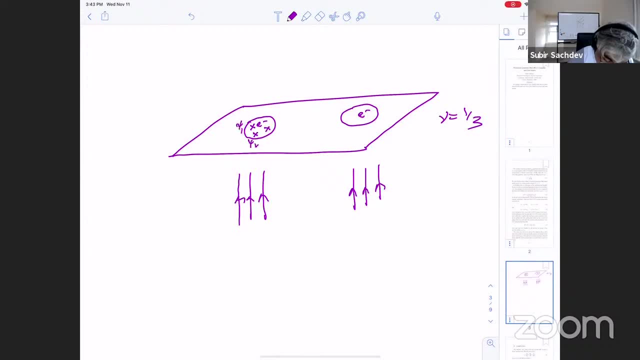 is actually made up of three particles: psi one side, two side, three, uh uh, and we're going to imagine that these, and we're going to imagine that these, and we're going to imagine that these flux, quanta, flux, quanta, flux, quanta, each act on one of the protons. 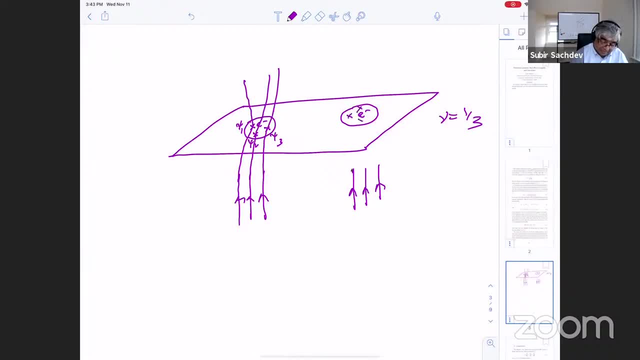 so you have one flux quantum for each. so you have one flux quantum for each. so you have one flux quantum for each proton. so that's, you know very crudely the. so that's, you know very crudely the. so that's you know very crudely the picture. 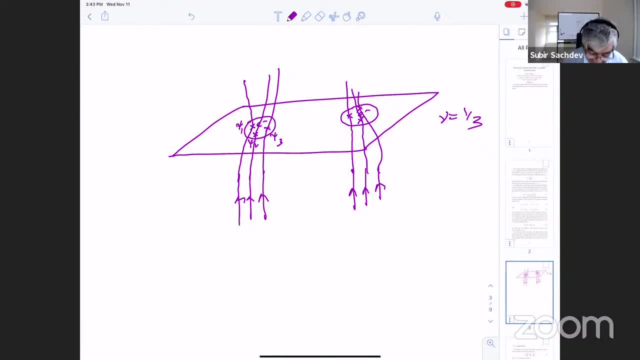 picture, picture. uh, of course we're going to do an. uh, of course we're going to do an. uh, of course we're going to do an actual calculation. so don't be actual calculation. so don't be actual calculation. so don't be alarmed by this very simplistic. 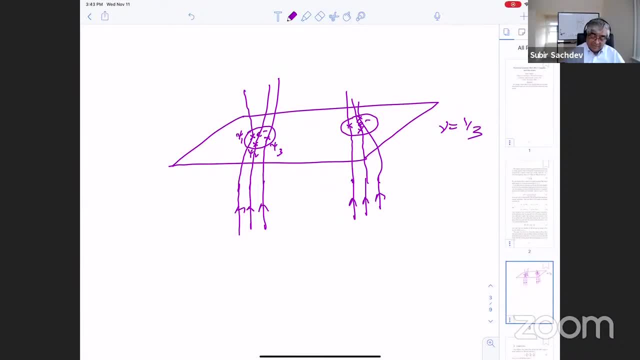 you know kindergarten type drawings. so, roughly speaking, you have one flux. so, roughly speaking, you have one flux. so, roughly speaking, you have one flux line for each electron, each part on now. line for each electron, each part on now. line for each electron, each part on now. and if you have 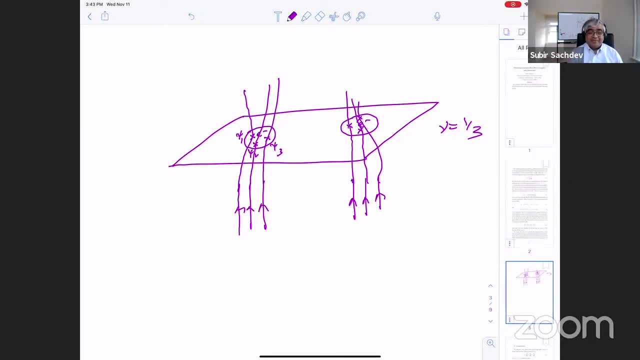 and if you have, and if you have a part on which is also fermion here, a part on which is also fermion here, a part on which is also fermion here to begin with, to begin with, to begin with, which has uh, which has uh, which has uh, one flux quantum per parton, but it's 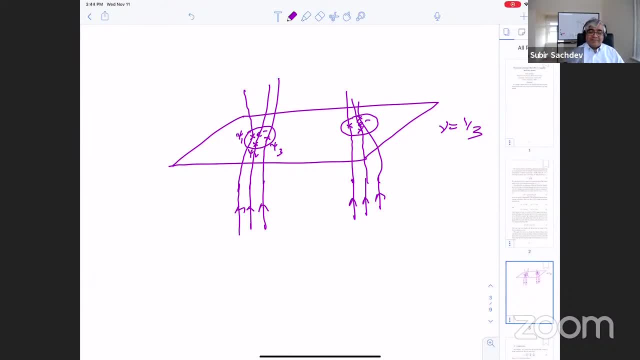 one flux quantum per parton. but it's one flux quantum per parton. but it's going to fully fill its land level, going to fully fill its land level, going to fully fill its land level. so the protons will fully occupy. so the protons will fully occupy. 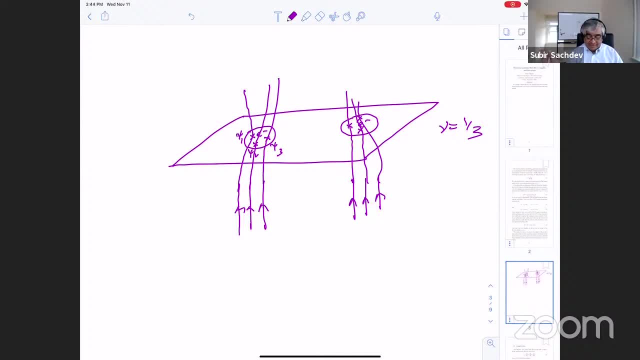 so the protons will fully occupy one single land level. one single land level. one single land level. okay, okay, okay, so that's the idea. so you have. so that's the idea, so you have. so that's the idea. so you have the electron of c, of r. 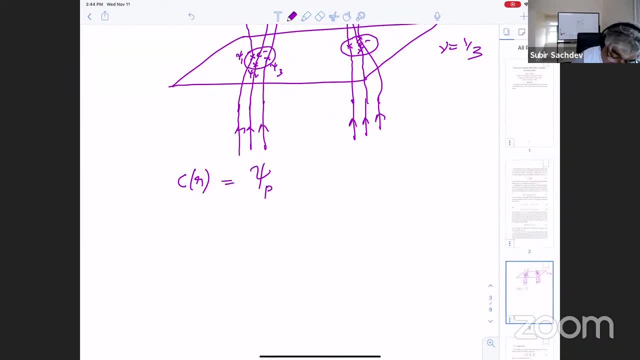 of c of r of c of r. the operator splits into the operator splits into the operator splits into electrons: psi 1 of r. psi. 1 of r. psi 1 of r. psi 2 of r. psi 2 of r. psi. 2 of r. psi. 3 of r. 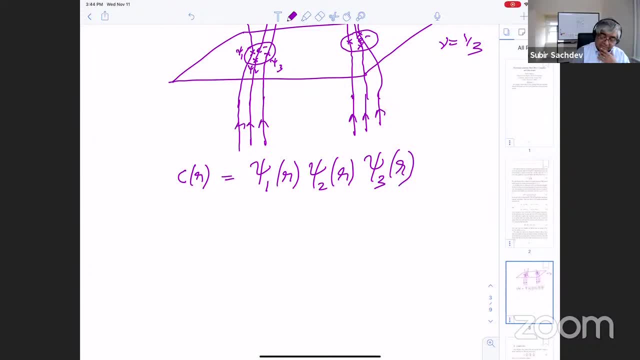 psi 3 of r, psi 3 of r um, um, um. okay, okay, okay, so they are. these protons have their own. so they are. these protons have their own. so they are. these protons have their own wave function and they all occupy a wave function and they all occupy a. 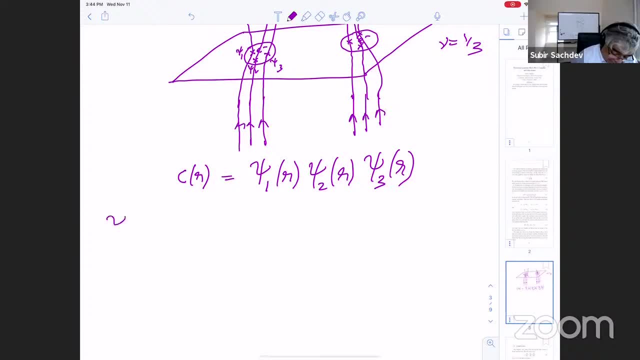 wave function and they all occupy a landau level, landau level, landau level. so what is the wave function of the? so what is the wave function of the? so what is the wave function of the electrons r1, r1, r1 to rn to rn. 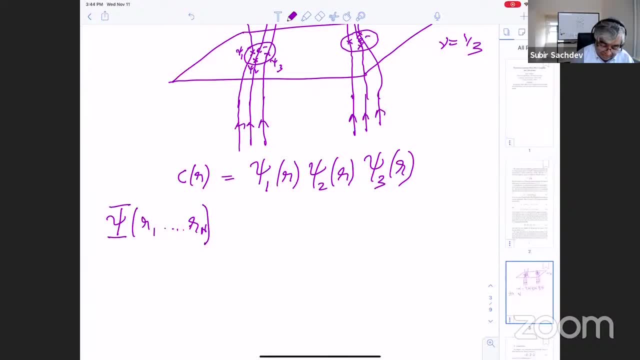 to rn this, this, this too many size. let's make this capital too many size. let's make this capital too many size. let's make this capital psi. this is the actual wave function. psi. this is the actual wave function. psi. this is the actual wave function. well, that's going to be a product of the. 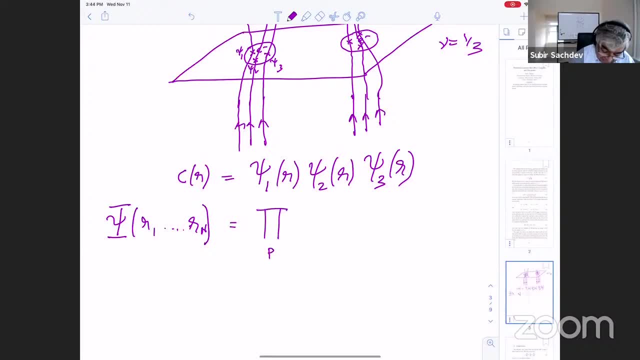 well, that's going to be a product of the. well, that's going to be a product of the wave function of each of the protons. so so, so part on wave function are called psi p, part on wave function are called psi p, part on wave function are called psi p. and we want the coordinates of the. 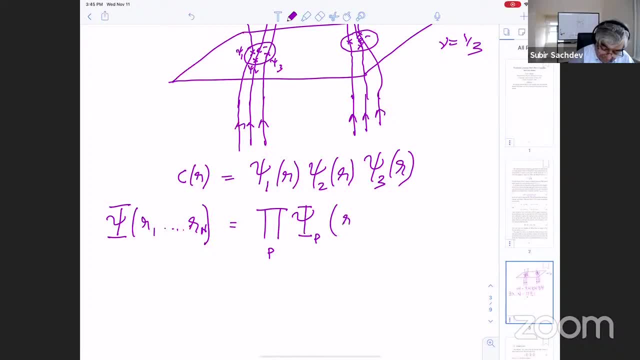 and we want the coordinates of the and we want the coordinates of the electron and the part on to be the same electron and the part on to be the same electron and the part on to be the same. so there'll be coordinates, uh. so there'll be coordinates, uh. 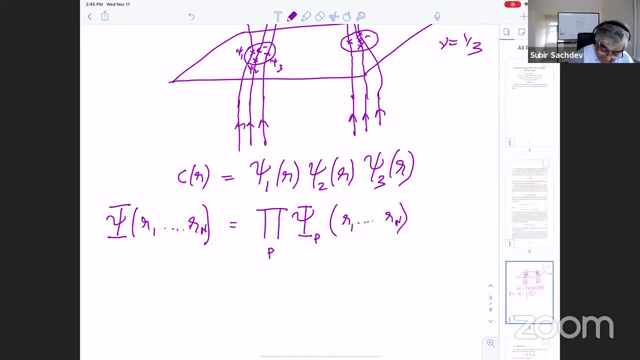 so there'll be coordinates. uh, you know, r1 through rn. now, what is so? each one of these now, what is so each one of these? now, what is so each one of these? is the part on wave function for a. is the part on wave function for a. 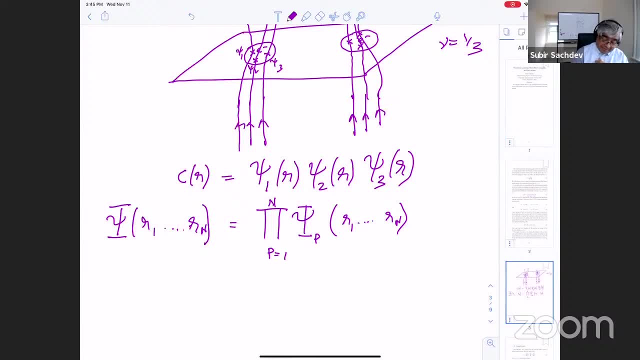 is the part on wave function for a part on in a fully failed landlord level, part on in a fully failed landlord level, part on in a fully failed landlord level. now you may remember i told you what the now you may remember. i told you what the now you may remember. i told you what the wave function of a fully filled and our 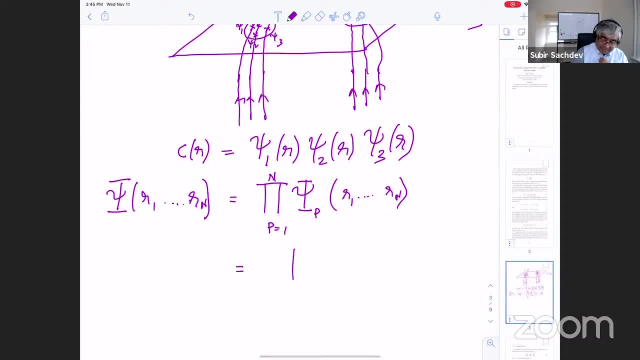 wave function of a fully filled and our wave function of a fully filled and our level was, level was, level was uh, it was uh, it was uh, it was product on product on product on i less than j, i less than j, i less than j, and i'll ignore the exponential factors. 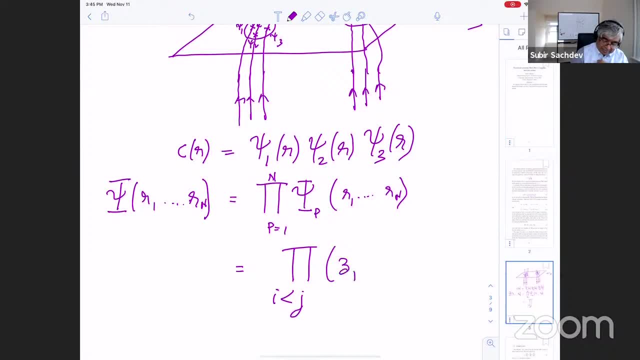 and i'll ignore the exponential factors, and i'll ignore the exponential factors, which all work out correctly, which all work out correctly, which all work out correctly: times zi minus zj. this was the times zi minus zj. this was the times zi minus zj. this was the wave function. 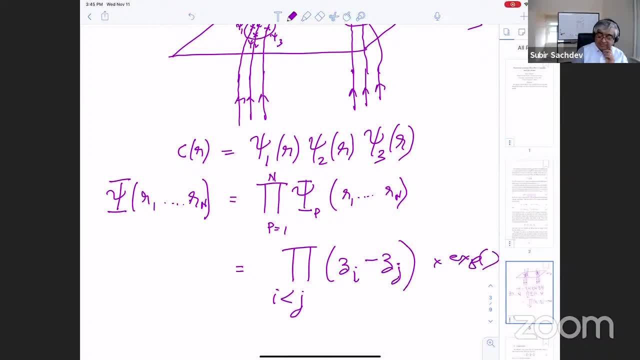 wave function. wave function times some exponential which i won't times, some exponential which i won't times, some exponential which i won't worry about, worry about. worry about uh wave function of a fully filled uh wave function of a fully filled uh. wave function of a fully filled lander level: the vanderbond determinant. 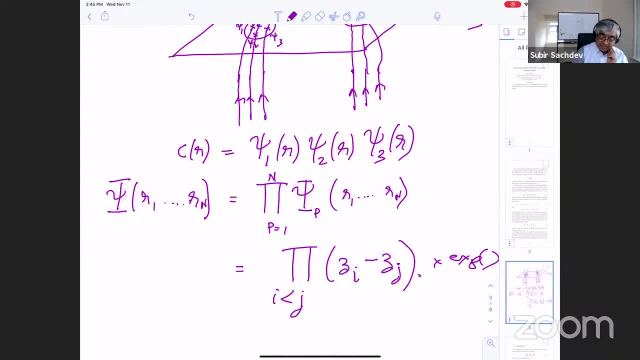 lander level: the vanderbond determinant. lander level: the vanderbond determinant. but i have three partons with the same. but i have three partons with the same. but i have three partons with the same. wave function: a fully lander level. wave function: a fully lander level. 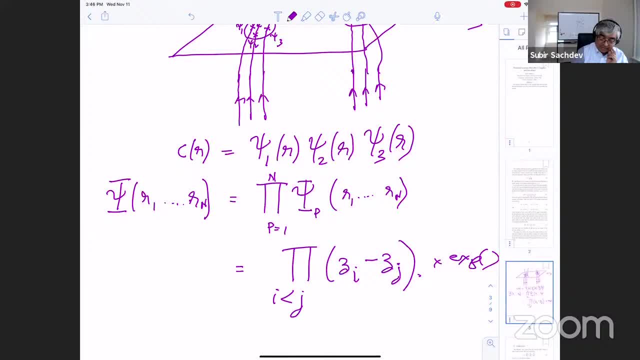 wave function, a fully lander level, and all of them, and all of them, and all of them have the same coordinate. so i'll just get have the same coordinate, so i'll just get have the same coordinate. so i'll just get this cube, this cube, this cube, and that's the famous laughlin wave. 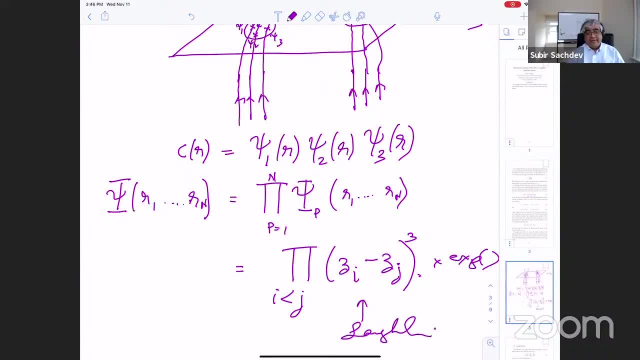 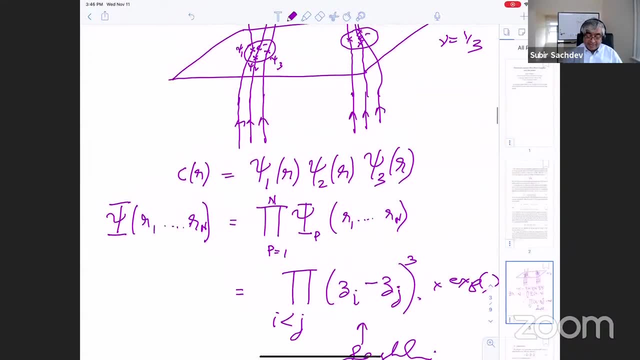 and that's the famous laughlin wave, and that's the famous laughlin wave function. now, amazingly, you can also do this: uh for, uh for, uh for for other states, in fact, almost all the for other states, in fact, almost all the for other states, in fact almost all the states that are observed. 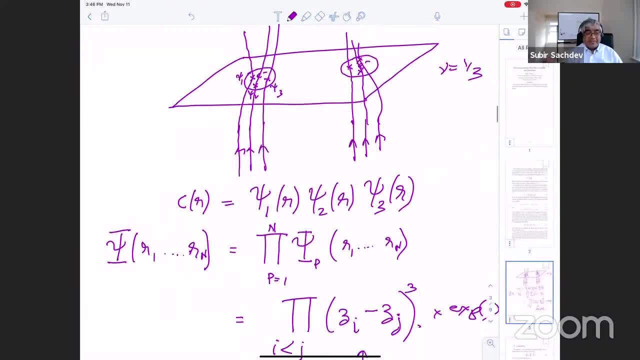 states that are observed, states that are observed- uh, that's so-called jane states. uh, that's so-called jane states. uh, that's so-called jane states. and the way you do it is by taking one, and the way you do it is by taking one, and the way you do it is by taking one of the partons. 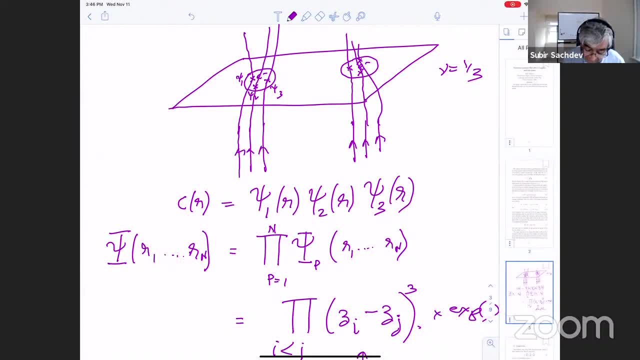 of the partons of the partons, but the third parton, there's only half. but the third parton, there's only half, but the third parton, there's only half. a flux quantum coming in a flux quantum coming in a flux quantum coming in for the third parton. well, if it has. 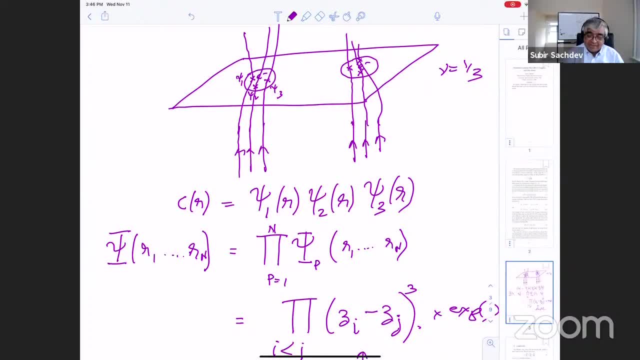 for the third parton? well, if it has for the third parton, well, if it has only half a flux quantum, that means it only half a flux quantum, that means it only half a flux quantum, that means it can occupy, can occupy, can occupy fully occupied two landau levels. and if 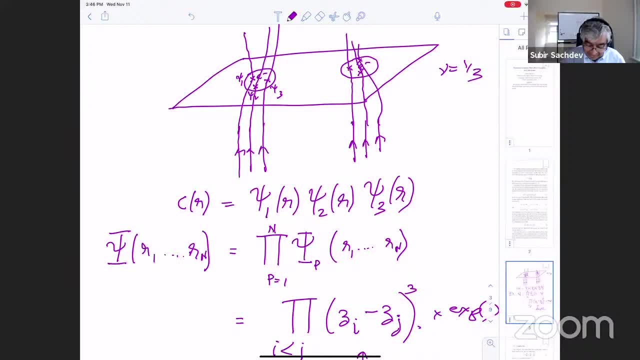 fully occupied two landau levels. and if fully occupied, two landau levels. and if you do that, you do that, you do that. uh, you end up getting the two-fifths. uh, you end up getting the two-fifths. uh, you end up getting the two-fifths state. 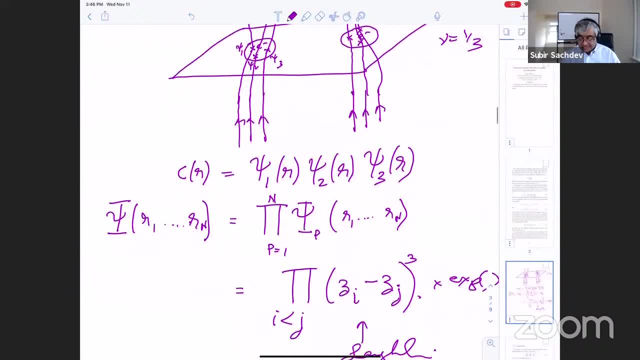 state state and in fact, that works very beautifully and in fact that works very beautifully and in fact that works very beautifully. so, so ridiculous as this construction, so so ridiculous as this construction, so so ridiculous as this construction- sounds, sounds, sounds. it's the one that works in practice you. 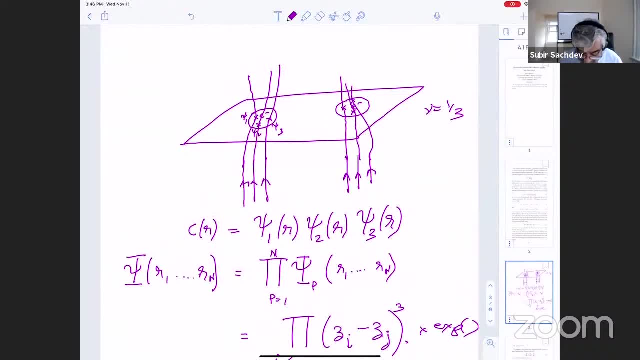 it's the one that works in practice. you, it's the one that works in practice. you know remarkably well in so many. know remarkably well in so many. know remarkably well in so many different, different, different experiments. okay, so that's all we're experiments. okay, so that's all we're. 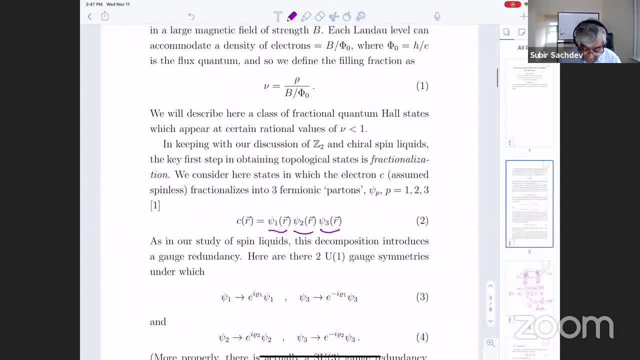 experiments. okay, so that's all we're going to do. going to do, going to do- uh and uh. here's a little bit more now. uh and uh. here's a little bit more now. uh and uh. here's a little bit more now. let's do this more formally. 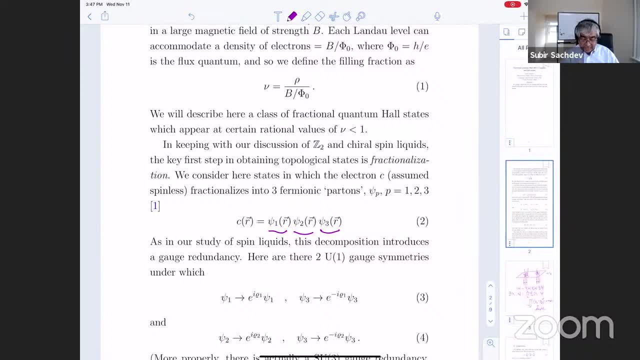 so we take our electron and we split it. so we take our electron and we split it. so we take our electron and we split it into three protons, into three protons, into three protons. okay, now we are. now we are gauge. okay, now we are. now we are gauge. 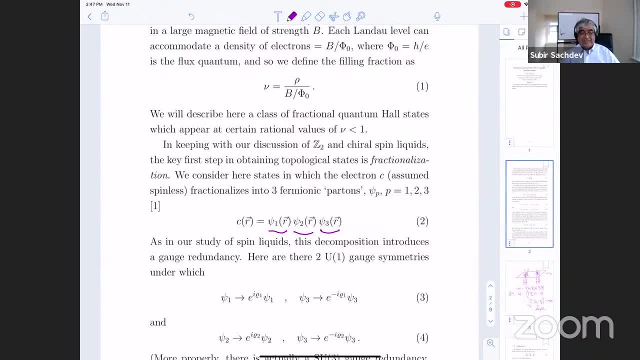 okay, now we are. now we are gauge theorists, so we want to derive. you know theorists, so we want to derive. you know theorists, so we want to derive. you know, every time we do a decomposition, every time we do a decomposition, every time we do a decomposition and there's a gauge field that got to. 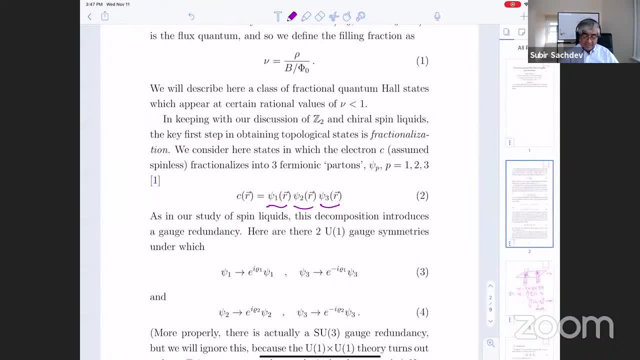 and there's a gauge field that got to, and there's a gauge field that got to come about. so now this one side, the come about. so now this one side, the come about. so now this one side, the moment i do this, i have now, moment i do this, i have now. 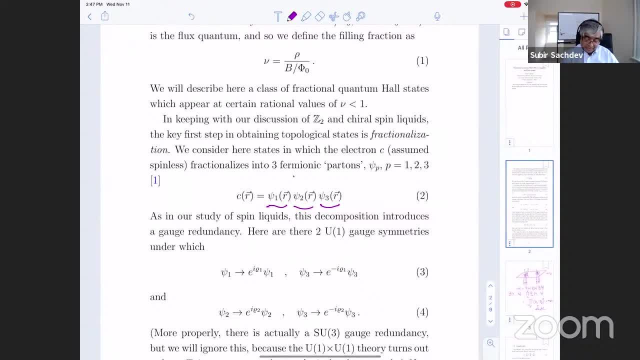 moment i do this, i have now a redundancy, a redundancy, a redundancy, and i have two redundancies, one, one, and i have two redundancies, one, one, and i have two redundancies, one, one redundancy here and one redundancy here, redundancy here and one redundancy here, redundancy here and one redundancy here. in fact, if you're really being strict, 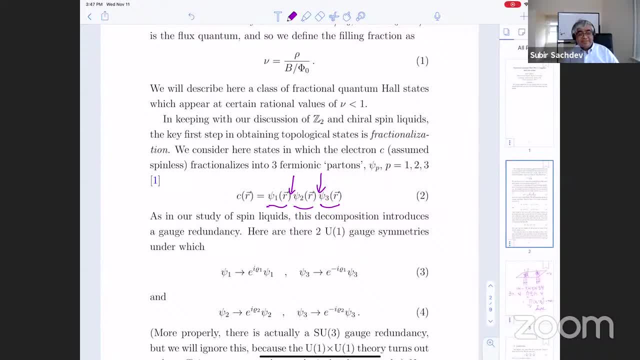 in fact, if you're really being strict, in fact, if you're really being strict, there's really an su3 redundancy and there's really an su3 redundancy, and there's really an su3 redundancy and it's an su3 gauge field. it's an su3 gauge field. 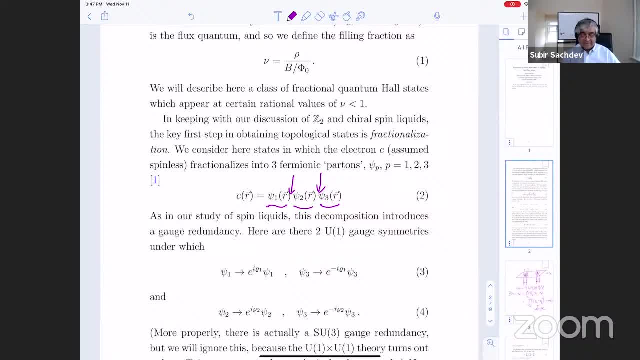 it's an su3 gauge field, but uh, it turns out you don't need it. so, but uh, it turns out you don't need it. so, but uh, it turns out you don't need it. so we'll just talk about the u1 gauge. we'll just talk about the u1 gauge. 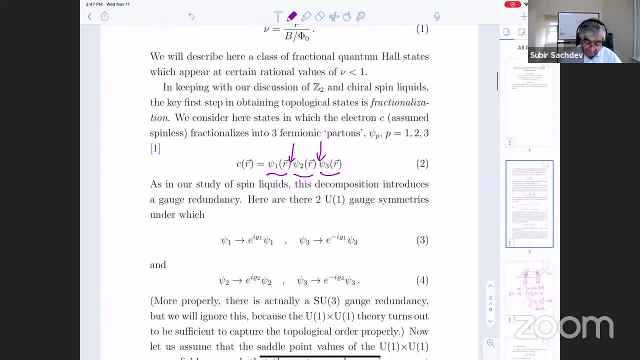 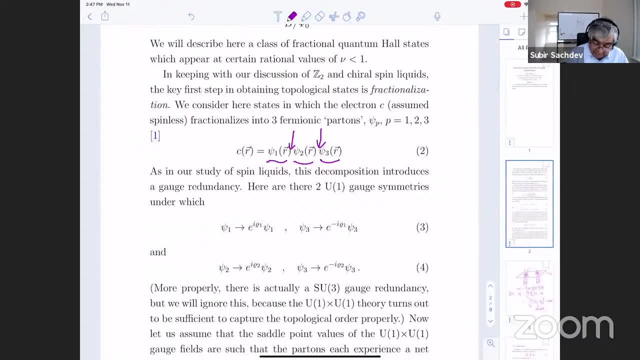 we'll just talk about the u1 gauge. redundancy here, redundancy here, redundancy here, uh, just to make our life simple, uh, just to make our life simple, uh, okay, so so, therefore, uh, okay, so so, therefore, uh, okay. so so, therefore, uh, there's one, there's a u1 grades. 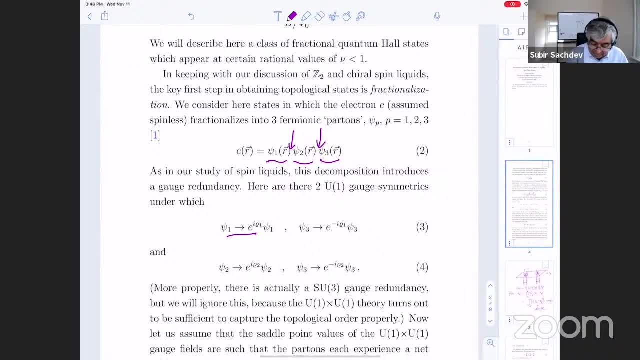 uh, there's one. there's a. u1 grades. uh, there's one. there's a u1 grades. transformation which generated by row one. transformation which generated by row one. transformation which generated by row one where psi one, where psi one, where psi one and side three have opposite signs, and. 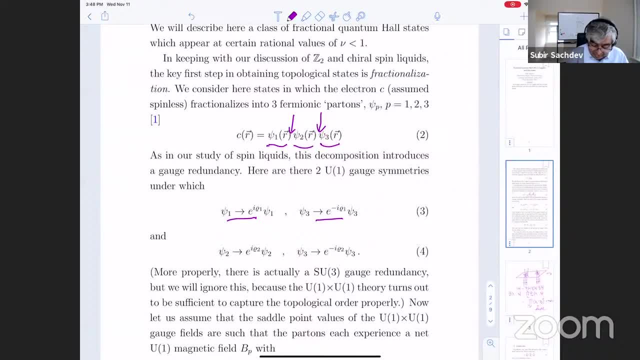 and side three have opposite signs and and side three have opposite signs and another one. does i choose to make side? another one does i choose to make side? another one does i choose to make side three special, three, special, three, special, uh, where side two and side three have. 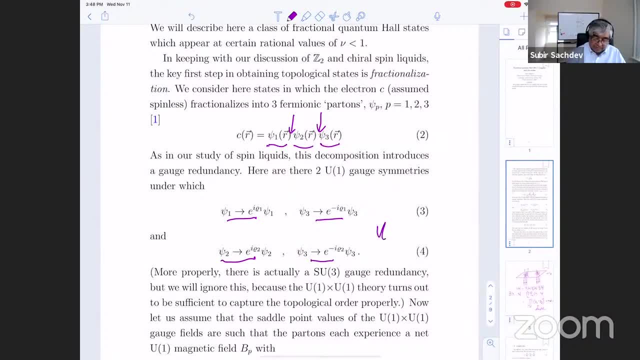 uh, where side two and side three have. uh, where side two and side three have opposite sides, opposite sides, opposite sides. so it's a u1 cross u1. there are two u1, so it's a u1 cross u1. there are two u1, so it's a u1 cross u1. there are two u1 gauge fields. 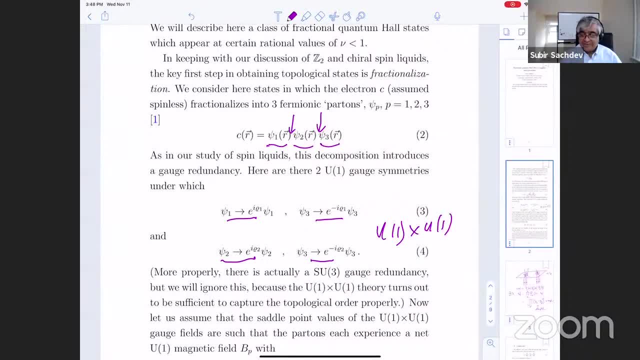 gauge fields. gauge fields- well, that's sounding promising. we we well, that's sounding promising. we, we well, that's sounding promising. we we know we already had chance. i'm in theory know we already had chance. i'm in theory know we already had chance. i'm in theory, with n gauge fields, so maybe we're. with n gauge fields. so maybe we're with n gauge fields, so maybe we're going to get two. in fact, you don't get going to get two. in fact you don't get going to get two. in fact, you don't get two at the end, two at the end. 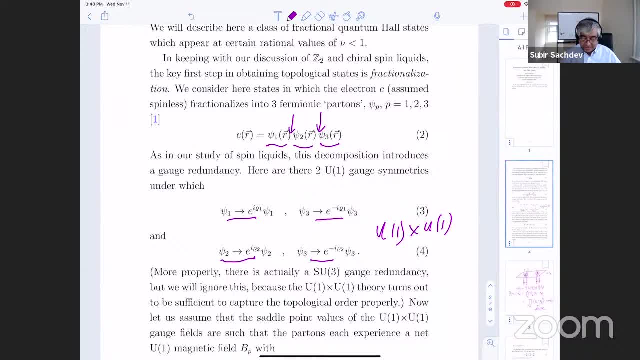 two at the end. uh, because of this the constraint, but uh, because of this the constraint, but uh, because of this the constraint, but anyway. so there seem to be two u1 gauge anyway. so there seem to be two u1 gauge anyway. so there seem to be two u1 gauge fields here, at least for now. 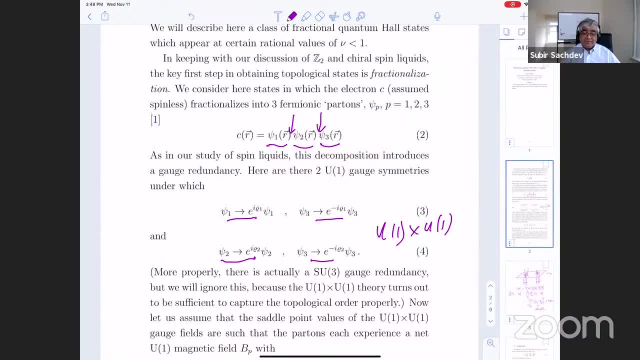 fields here, at least for now. fields here, at least for now. so if you write down any theory of the, so if you write down any theory of the, so if you write down any theory of the protons, i'm going to have to have two protons. i'm going to have to have two. 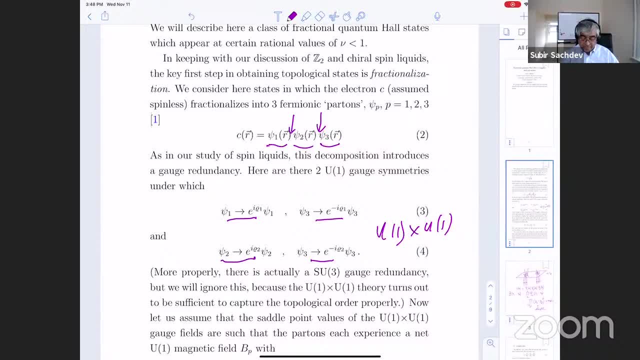 protons, i'm going to have to have two gauge fields. because there are two gauge fields, because there are two gauge fields, because there are two constraints, constraints, constraints, okay, okay, okay. so that's point number one. so that's point number one, so that's point number one. so now i take my original theory. 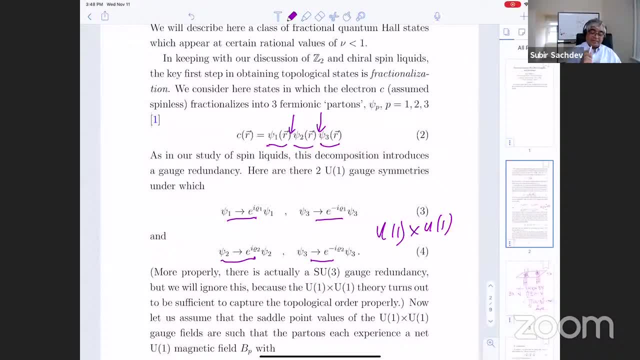 so now i take my original theory. so now i take my original theory for the electron which experiences, for the electron which experiences, for the electron which experiences a magnetic field, a magnetic field, a magnetic field due to the external gauge field, and then i write down a theory for 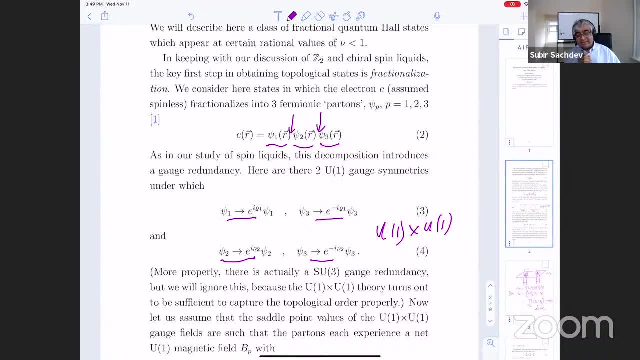 and then i write down a theory for, and then i write down a theory for: psi 1 psi 2 psi, 3 psi 1 psi 2 psi 3 psi 1 psi 2, psi 3, which experience not only the external, which experience not only the external. 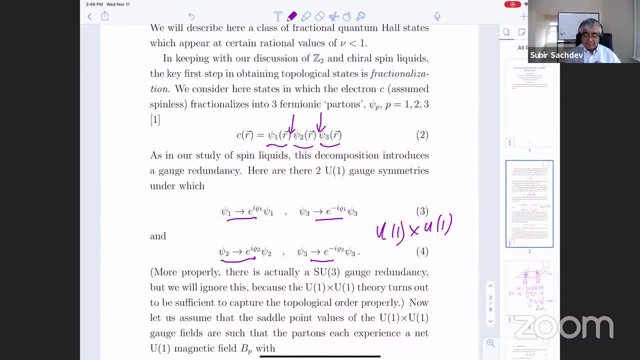 which experience not only the external gauge field but also the internal gauge gauge field, but also the internal gauge gauge field but also the internal gauge field. so now i look for a saddle point. so now i look for a saddle point. so now i look for a saddle point now because i already have a gauge. 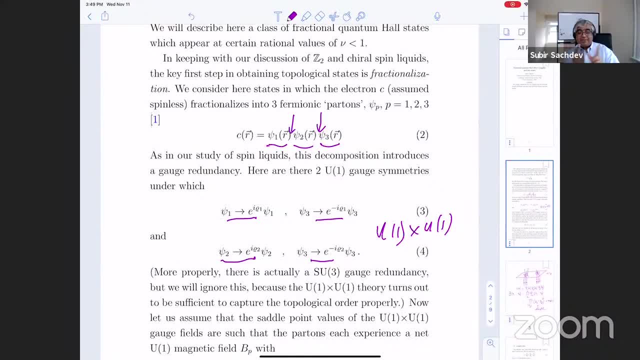 now because i already have a gauge, now because i already have a gauge magnetic field in the external gauge magnetic field, in the external gauge magnetic field, in the external gauge field, it seems reasonable that i will field. it seems reasonable that i will field, it seems reasonable that i will also have. 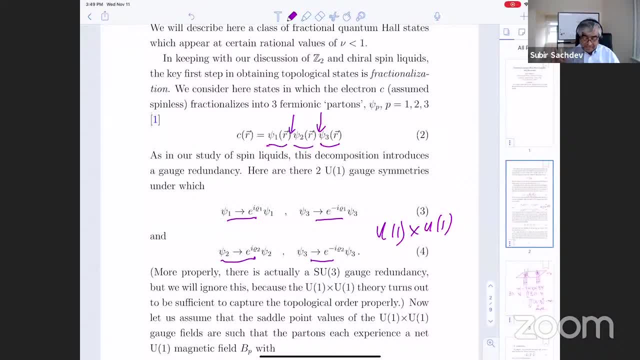 also have, also have a magnetic field due to the internal, a magnetic field due to the internal gauge fields, gauge fields, gauge fields. so really for each parton, i should be so, really for each parton, i should be so, really for each parton, i should be looking at the sum of the magnetic 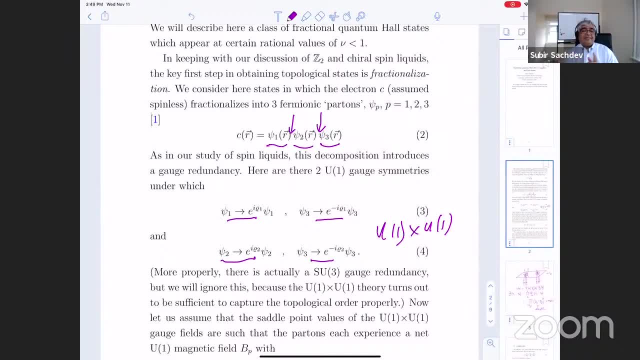 looking at the sum of the magnetic, looking at the sum of the magnetic fields, fields, fields, the one due to the external field and the one due to the external field. and the one due to the external field and the one due to the internal field, the one due to the internal field. 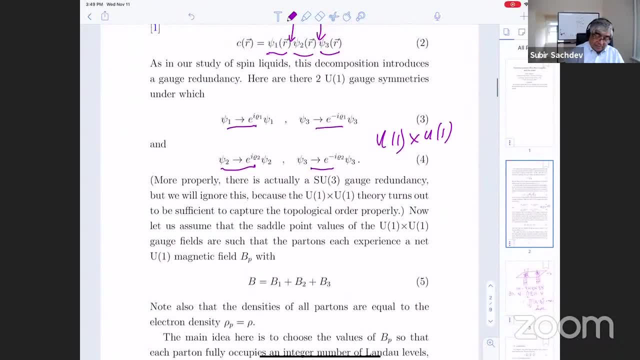 the one due to the internal field. okay, now, first of all, you can see already now, first of all, you can see already now. first of all, you can see already from here if there's an internal gauge from here, if there's an internal gauge from here, if there's an internal gauge field on psi 1. 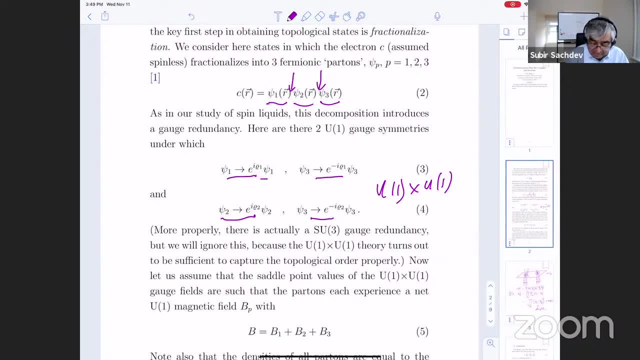 field on psi 1, field on psi 1, internal magnetic field on psi 1, the internal field on psi 3. the internal field on psi 3, the internal field on psi 3 is equal and opposite is equal, and opposite is equal and opposite. if there's an internal field on side 2. 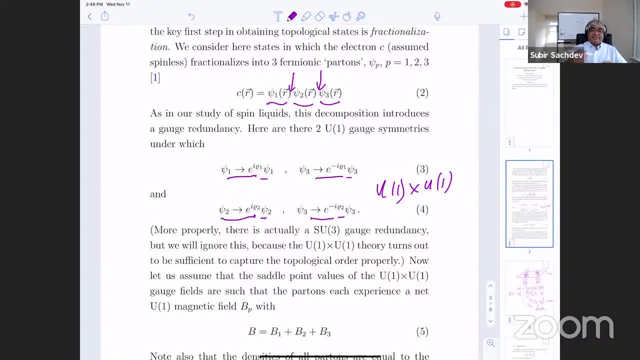 if there's an internal field on side 2. if there's an internal field on side 2, the internal field on side 3 is equal and the internal field on side 3 is equal and the internal field on side 3 is equal and opposite. so these internal gate. 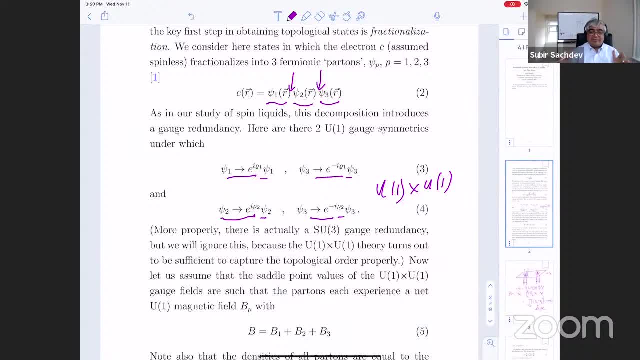 opposite. so these internal gate opposite, so these internal gate magnetic fields are not going to change. magnetic fields are not going to change. magnetic fields are not going to change the sum of the, the sum of the, the sum of the of the gauge field, of the gauge field. 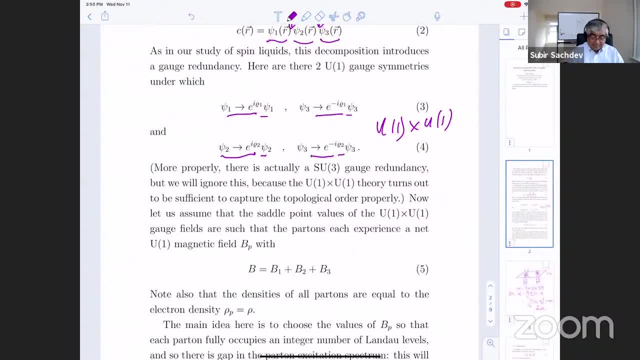 of the gauge field. so let's assume that there's some total. so let's assume that there's some total, so let's assume that there's some total. magnetic field, magnetic field, magnetic field, bp, bp that each parton experiences. this bp involves both the external field. 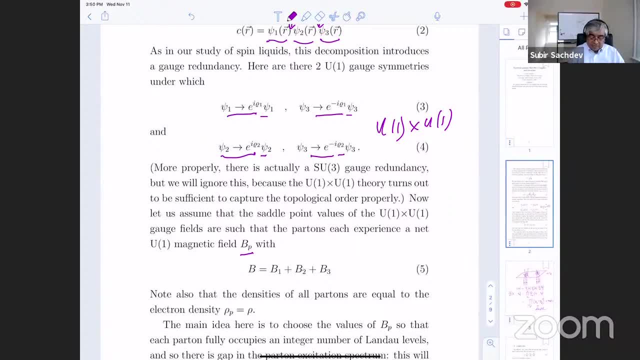 this bp involves both the external field. this bp involves both the external field and the internal field. so we have a constraint that the total. so we have a constraint that the total. so we have a constraint that the total field must be the sum of the internal field must be the sum of the internal. 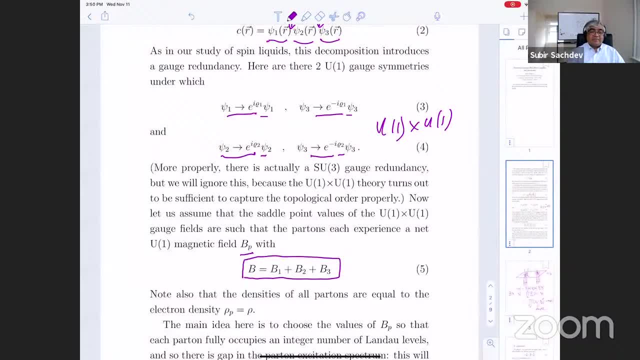 field must be the sum of the internal fields on the three partons fields on the three partons fields on the three partons, because the internal fields always act, because the internal fields always act, because the internal fields always act equally and opposite equally and opposite, equally and opposite on any pair of particles. 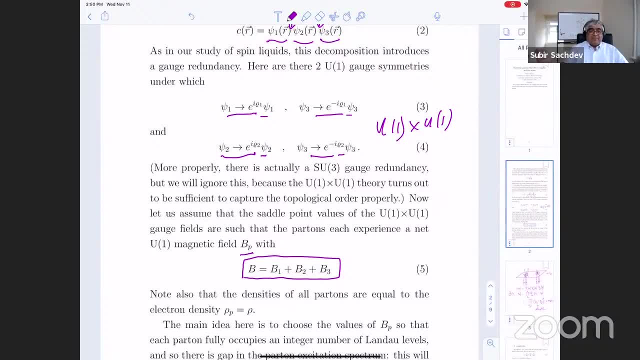 on any pair of particles, on any pair of particles. all right, all right, all right. so now we are. we have to choose b1- b2. so now we are, we have to choose b1- b2. so now we are, we have to choose b1, b2, b3. 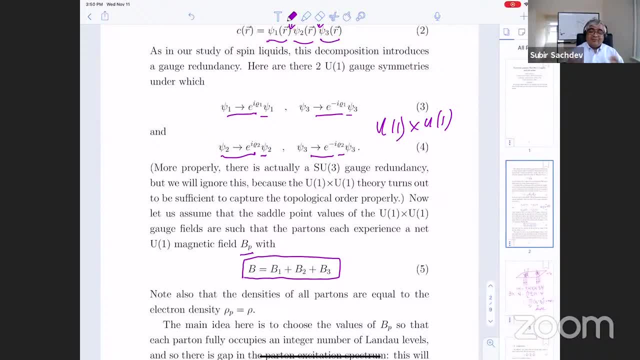 b3, b3, and it's really up to us to choose it. and it's really up to us to choose it. and it's really up to us to choose it. and how do we want to choose it, but we? and how do we want to choose it, but we? 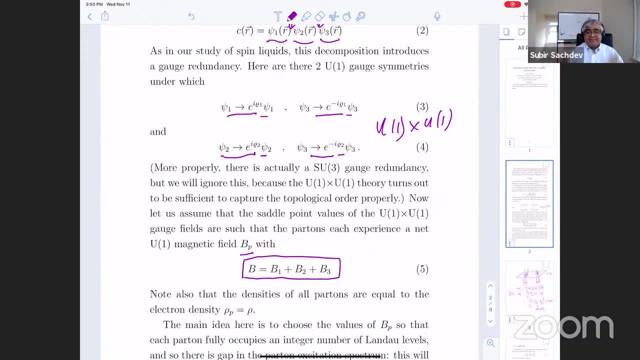 and how do we want to choose it? but we want to choose it in a way that the mean want to choose it, in a way that the mean want to choose it, in a way that the mean field has a gap field, has a gap field, has a gap. now that's a good mean field. if you do a 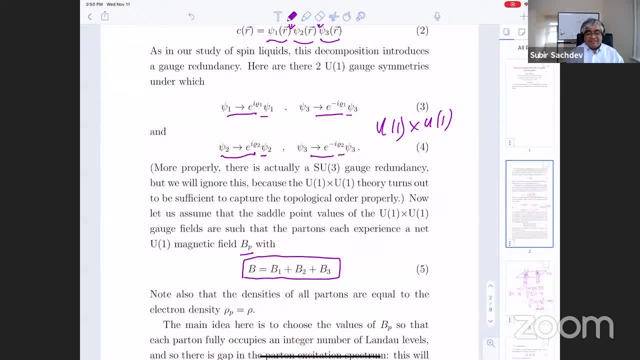 now that's a good mean field. if you do a, now that's a good mean field. if you do a mean field theory, mean field theory, mean field theory, and then you get a state that's non, and then you get a state that's non, and then you get a state that's non, degenerate and has a gap. 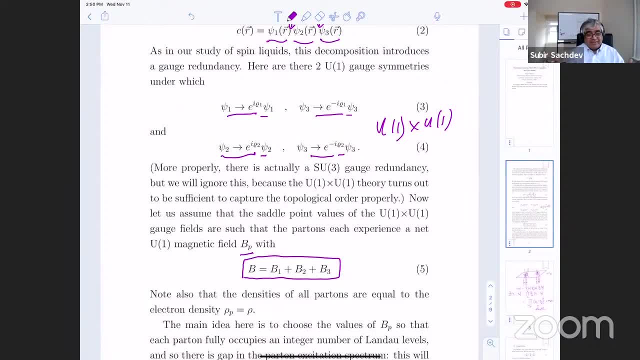 degenerate and has a gap, degenerate and has a gap. well, that means you can make progress well. that means you can make progress well. that means you can make progress from it, from it, from it. so you want to choose a field so that. so you want to choose a field so that. 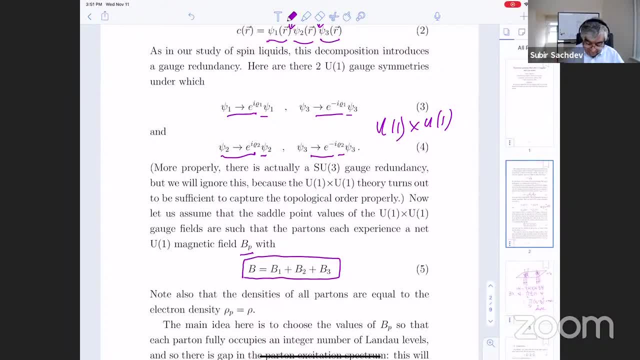 so you want to choose a field so that the mean field has a gap, the mean field has a gap, the mean field has a gap, and so and so and so. so, basically, you always want to choose, so, basically, you always want to choose. so, basically, you always want to choose b1, b2 and b3. 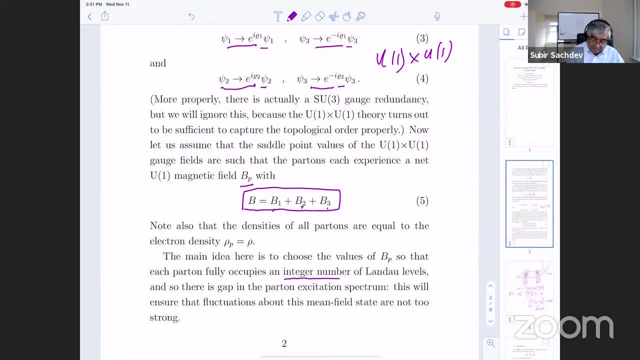 b1, b2 and b3. b1, b2 and b3, so that each parton occupies an integer. so that each parton occupies an integer. so that each parton occupies an integer number of gander levels. number of gander levels. number of gander levels, because only then the parton would have. 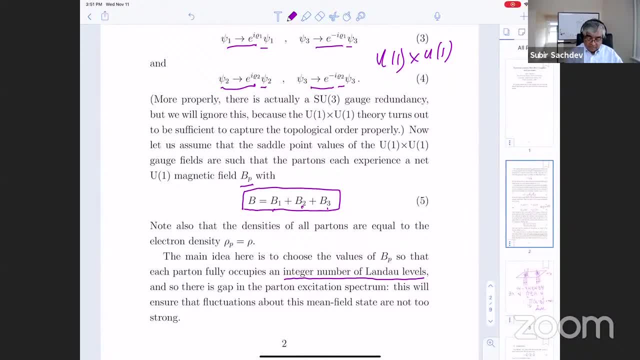 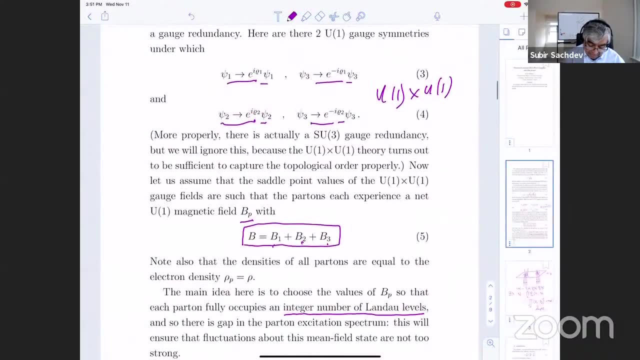 because only then the parton would have, because only then the parton would have a gap in its spectrum, a gap in its spectrum, a gap in its spectrum. okay so, okay so, okay, so, if i do this more generally, right. so what can we say? that let's do. 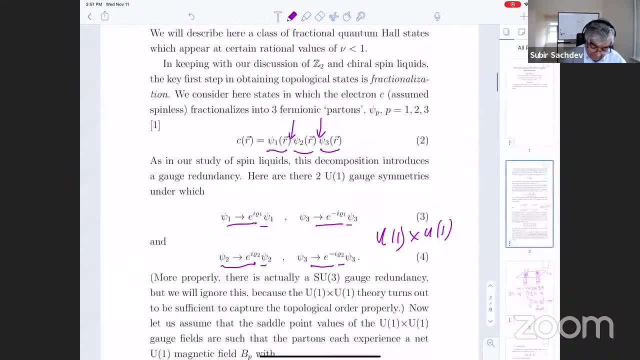 right. so what can we say that? let's do right. so what can we say that? let's do it over here, it over here, it over here. so we have. let's do it over here. no, let me make. let's do it over here. no, let me make. 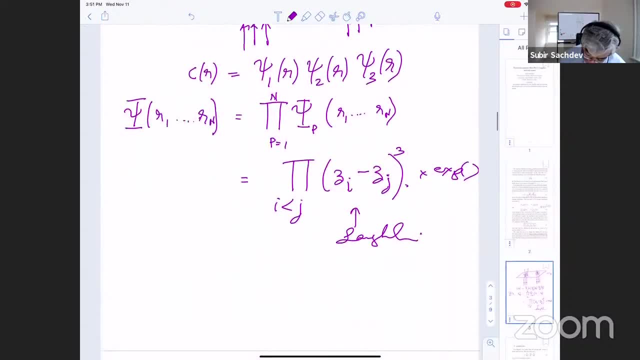 let's do it over here. no, let me make another page sorry. another page sorry. another page, sorry. let me make another page. let me make another page sorry. so we have the filling fraction. so we have the filling fraction. so we have the filling fraction of, of of the original electron. 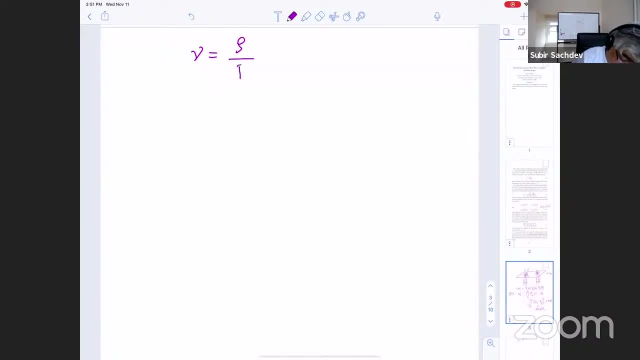 the original electron. the original electron is the density of electrons. is the density of electrons is the density of electrons divided by b. so i'll just drop the divided by b. so i'll just drop the divided by b. so i'll just drop the factors of phi naught. 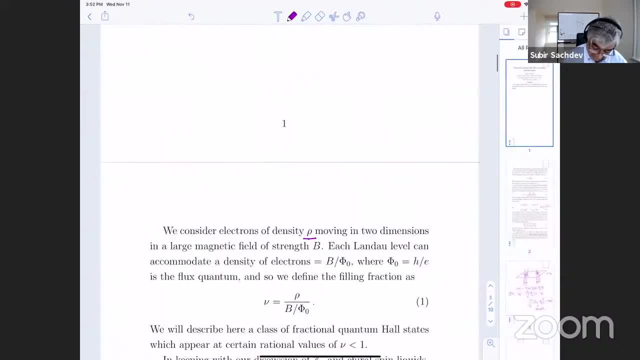 factors of phi naught. factors of phi naught, they just are very common and they just, they just are very common and they just they just are very common and they just make a life very complicated, make a life very complicated, make a life very complicated. so, filling fraction of the electrons. 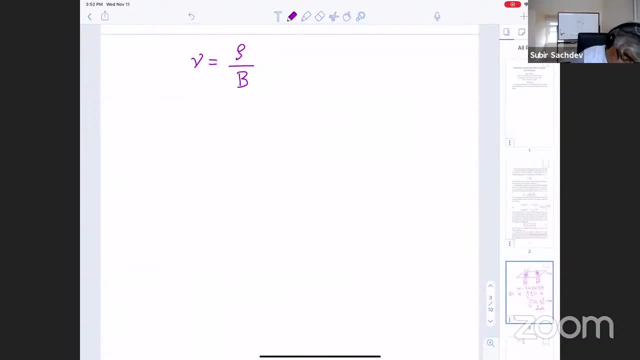 so filling fraction of the electrons. so filling fraction of the electrons is: is is is b, is b is b, then we also have b, then we also have b, then we also have b equals b1 plus b2, equals b1 plus b2, equals b1 plus b2 plus b3. 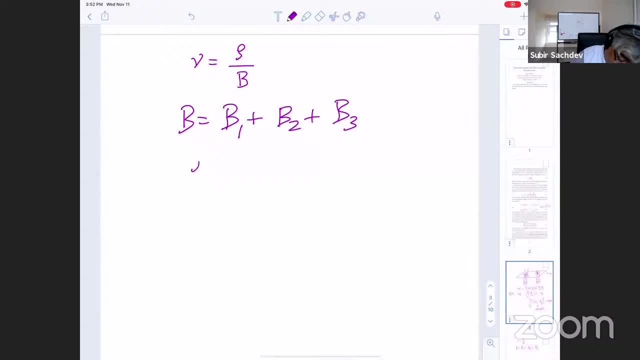 plus b3 plus b3. then what do we want, we want? then, what do we want, we want? then? what do we want, we want now? we also know that the density of the now we also know that the density of the now we also know that the density of the electrons is equal to the density of the. 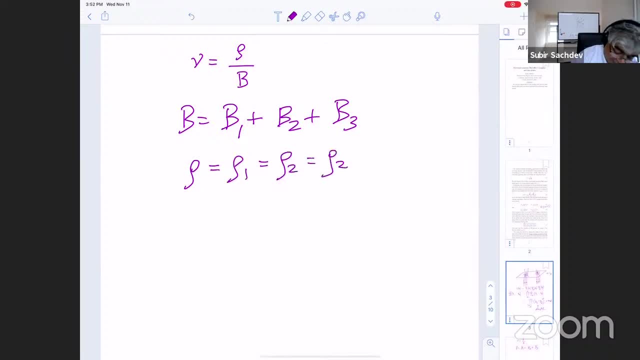 electrons is equal to the density of the electrons is equal to the density of the partons, partons, partons. they're all equal. because every time you they're all equal, because every time you they're all equal. because every time you put an electron you put one part on each. 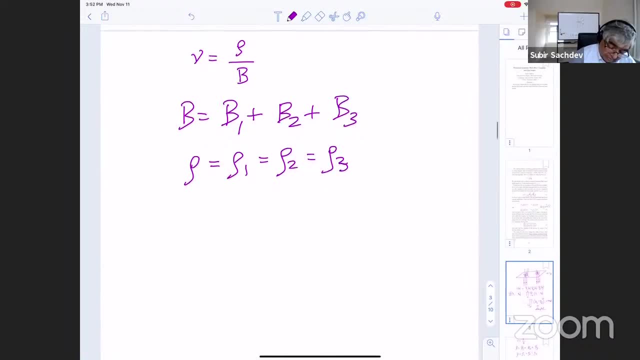 put an electron, you put one part on each. put an electron, you put one part on each type, type, type. uh, okay, so that's something else. you uh okay, so that's something else. you uh, okay, so that's something else you know. and then you want the partons to 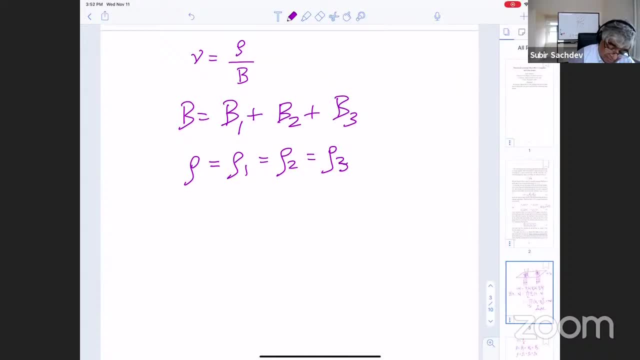 know, and then you want the partons to know, and then you want the partons to have, have, have, uh uh, uh. occupy an integer number of landau level. occupy an integer number of landau level. occupy an integer number of landau level, so that what you, what you also want, 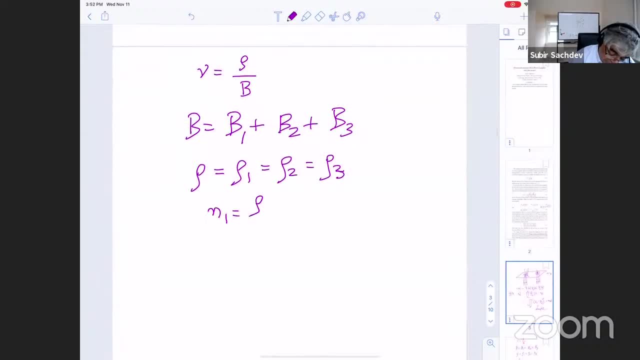 so that what you, what you also want, so that what you, what you also want is: n1 is, n1 is, n1 is is is rho, because rho and rho are over b1 rho, because rho and rho are over b1 rho, because rho and rho are over b1. you want n2. 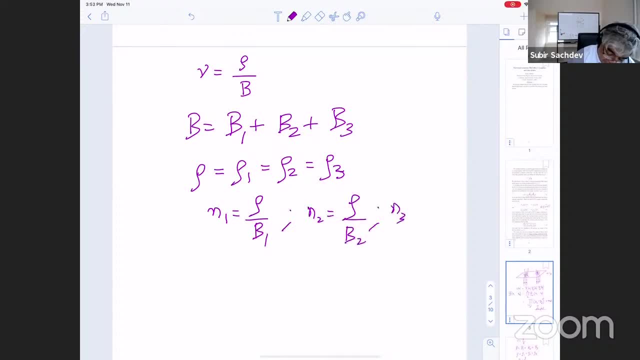 you want n2, you want n2 is rho over b2, is rho over b2, is rho over b2. and you want n3 and you want n3, and you want n3 is rho over b3, with, with, with n1, n1, n1 and two. 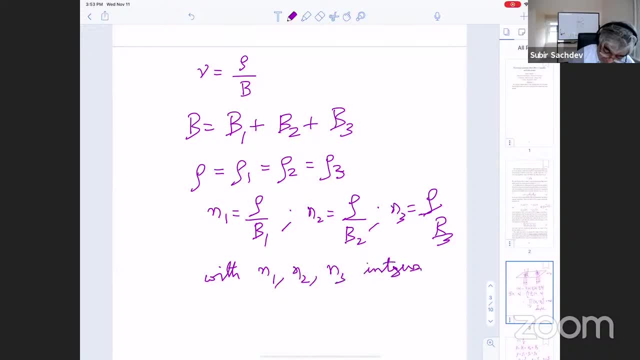 and two and two and three integers. okay, so now you have a set of relations. okay, so now you have a set of relations. okay, so now you have a set of relations. uh, you give me a new. uh, you give me a new. uh, you give me a new. and then you try to find n1, n2 and n3. 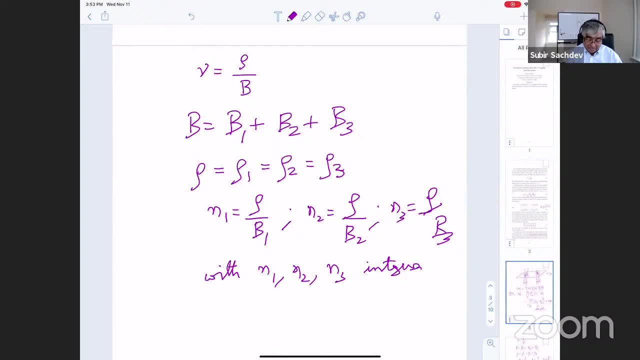 and then you try to find n1, n2 and n3, and then you try to find n1, n2 and n3, so that this, this all works. so this won't so that this this all works. so this won't so that this this all works. so this won't work for any value of new. 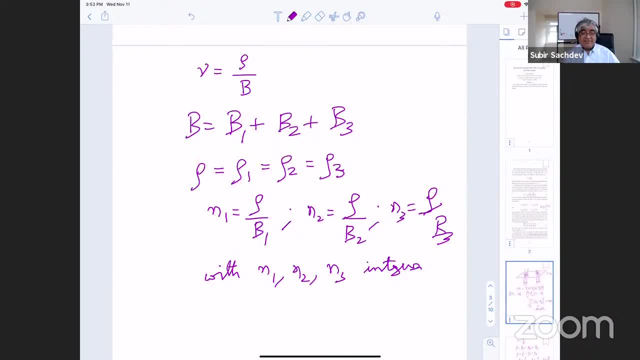 work for any value of new, work for any value of new, if you try to eliminate all the variables. if you try to eliminate all the variables, if you try to eliminate all the variables in these equations, only certain in these equations, only certain in these equations, only certain values of new. 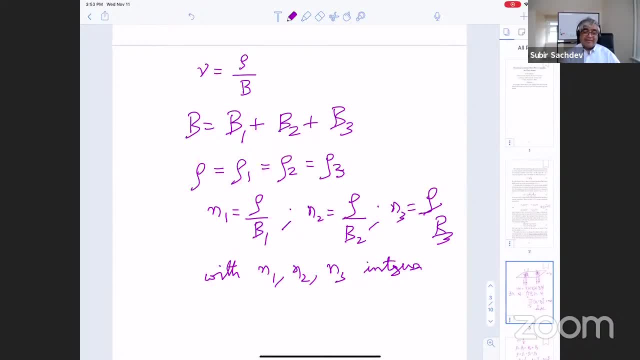 values of new, values of new. will this whole thing work? and if it, will this whole thing work? and if it, will this whole thing work? and if it works, then you're guaranteed to have a works. then you're guaranteed to have a works, then you're guaranteed to have a gap. 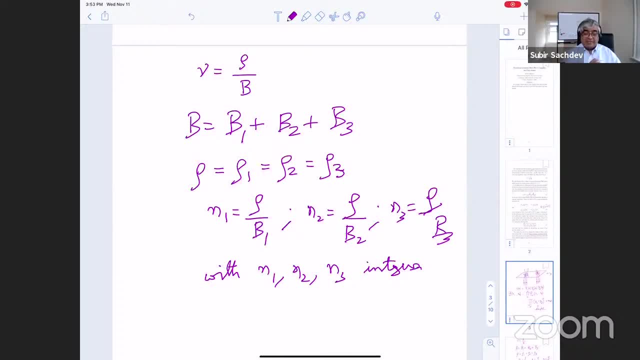 gap, gap above the uh, above the uh, above the uh, the observed states, the observed states, the observed states above the mean field theory, above the mean field theory, above the mean field theory. and the remarkable fact which is i was, and the remarkable fact which is i was, 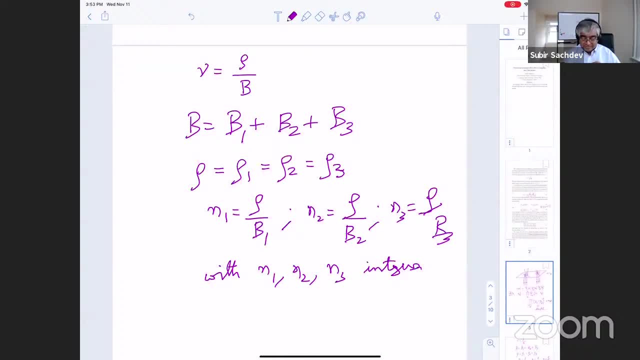 and the remarkable fact, which is i was stepping forward to that, stepping forward to that, stepping forward to that is that essentially, all observed states is that essentially all observed states is that essentially all observed states can be described by some choice of n1, can be described by some choice of n1. 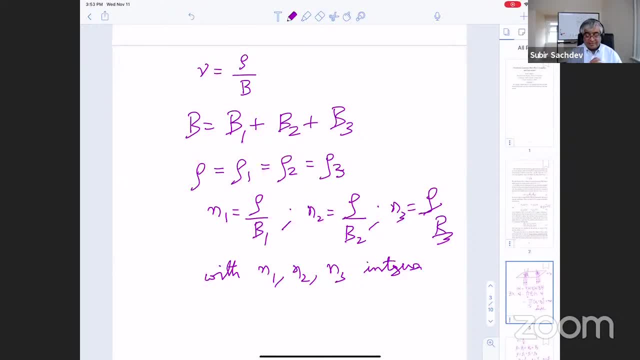 can be described by some choice of n1 and n2 and three and n2 and three and n2 and three. that's the beauty of it. in fact they can. that's the beauty of it, in fact, they can. that's the beauty of it, in fact. they can also be some of the n2 and nc can even. 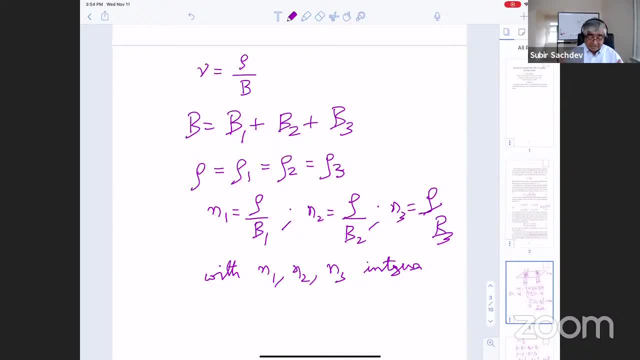 also be. some of the n2 and nc can even also be. some of the n2 and nc can even be negative, be negative, be negative, so the magnetic field can be pointing, so the magnetic field can be pointing, so the magnetic field can be pointing the other direction. for some of the 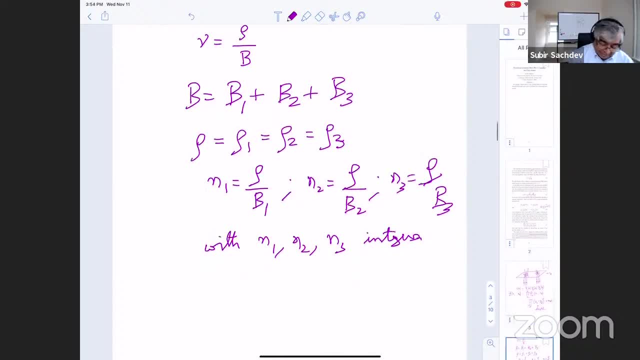 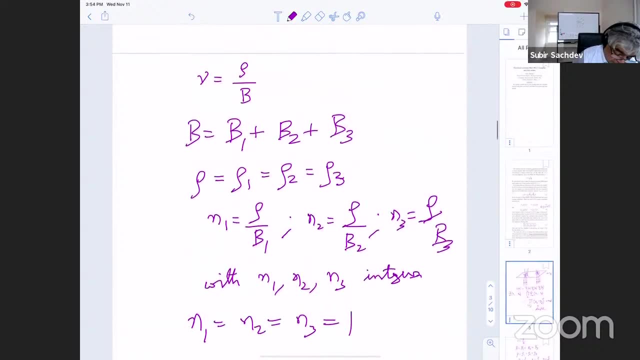 the other direction for some of the, the other direction for some of the particles. so the simplest case, so the simplest case. so the simplest case is: n1 is n1, is n1 equals two equals n3 equals one. and if equals two equals n3 equals one. and if 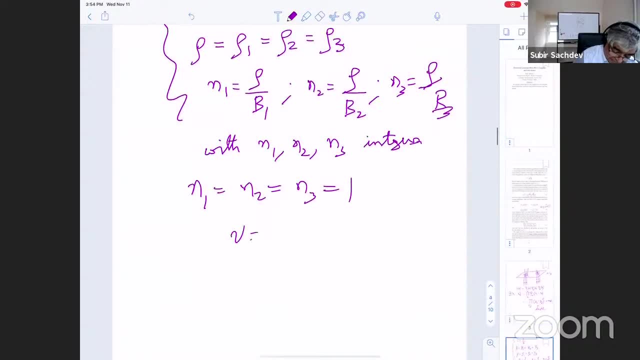 equals two, equals n3 equals one. and if you just do the numerology of these, you just do the numerology of these, you just do the numerology of these equations, you'll find that that means equations. you'll find that that means equations. you'll find that that means nu equals one third. 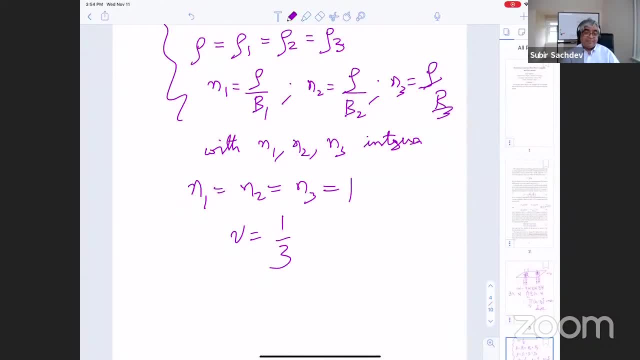 nu equals one third, nu equals one third. so that's the famous Laughlin case. so that's the famous Laughlin case. so that's the famous Laughlin case. so each parton sees, so each parton sees, so each parton sees, uh, exactly one flux quantum. and you and 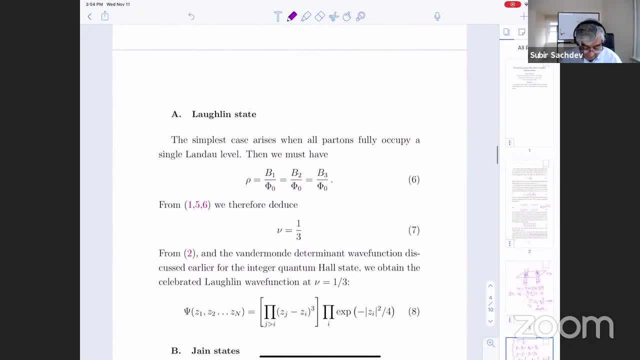 uh, exactly one flux quantum. and you and uh, exactly one flux quantum. and you, and i already showed you, i already showed you, i already showed you- that gives you the Laughlin wave function, that gives you the Laughlin wave function, that gives you the Laughlin wave function. so 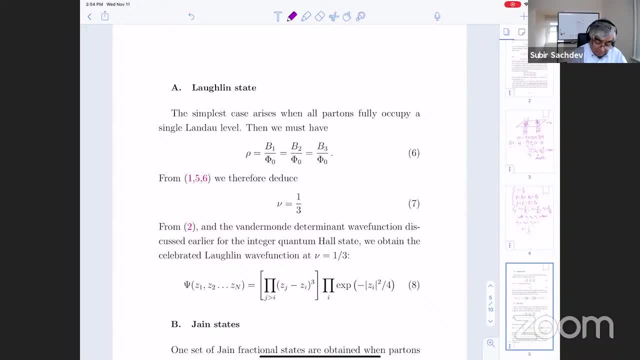 so, um, yeah, so b1 over five. yeah, this is the case where you have exactly this is the case where you have exactly this is the case where you have exactly one integer landau level filled, one integer landau level filled, one integer landau level filled, and nu is one third. 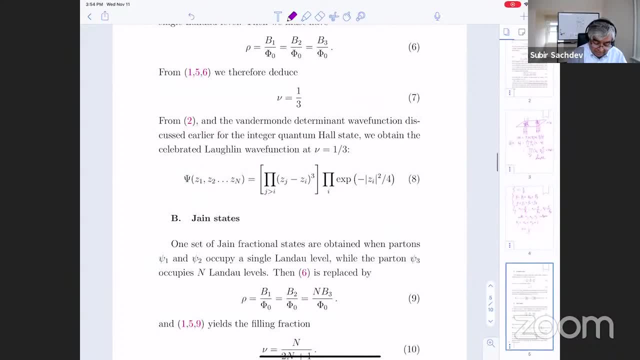 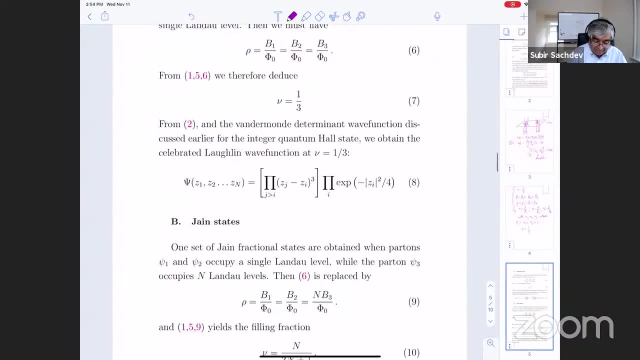 and nu is one third and nu is one third. uh, the other important case, uh, the other important case. uh, the other important case is: when is when is when? two of them are one and the third is two of them are one and the third is two of them are one and the third is some other integer. so case two: 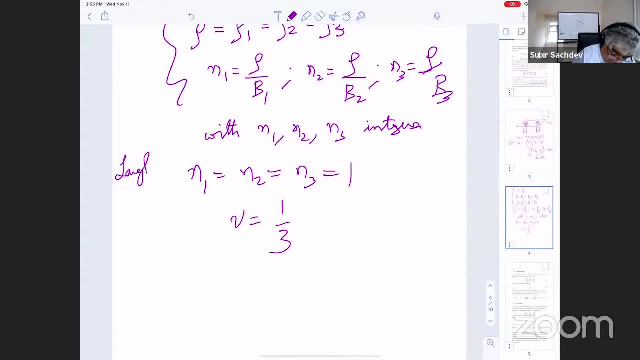 so this is the Laughlin case. so this is the Laughlin case. so this is the Laughlin case, and the other case is jane and i'm just, and the other case is jane and i'm just, and the other case is jane and i'm just taking the simplest. 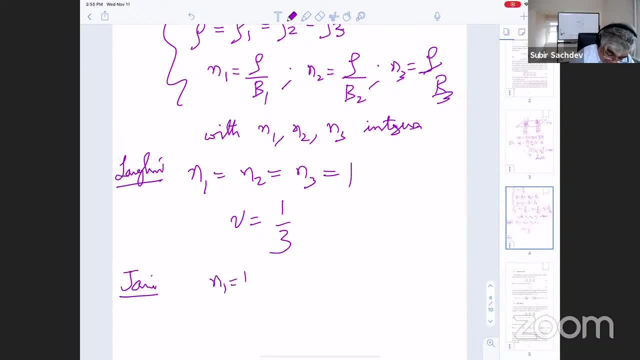 taking the simplest. taking the simplest: jane and Laughlin cases. jane and Laughlin cases. jane and Laughlin cases. that turns out to be n1 equals one, that turns out to be n1 equals one, that turns out to be n1 equals one, and two equals one. 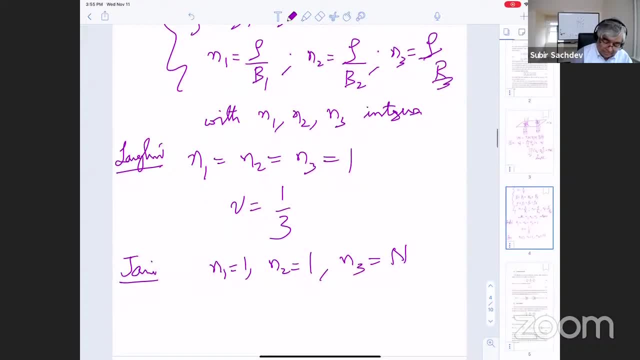 and two equals one and two equals one and three equals n and three equals n and three equals n? uh. and then if you work out the uh, and then if you work out the uh, and then if you work out the numerology, you'll find the filling. 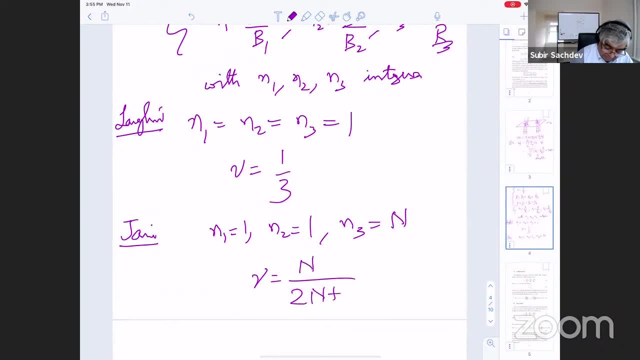 numerology. you'll find the filling numerology. you'll find the filling fraction is: nu is n. fraction is nu is n. fraction is nu is n over 2n plus one. in fact, you know, i, i remember this when i. in fact, you know i, i remember this when i. 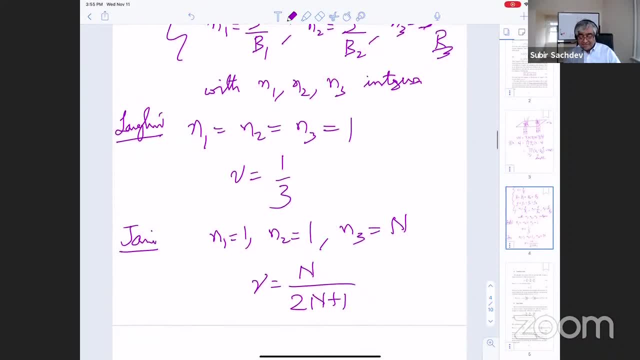 in fact, you know, i i remember this, when i was at yale in those days and jane was at yale in those days and jane was at yale in those days and jane was a postdoc, there was a postdoc, there was a postdoc there and there were all these experiments. 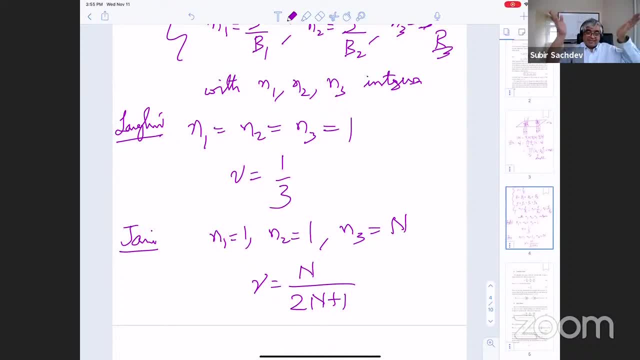 and there were all these experiments, and there were all these experiments going out, going out, going out showing this sequence of fractions, which showing this sequence of fractions, which showing this sequence of fractions which just happened to be n over 2n plus one, just happened to be n over 2n plus one. 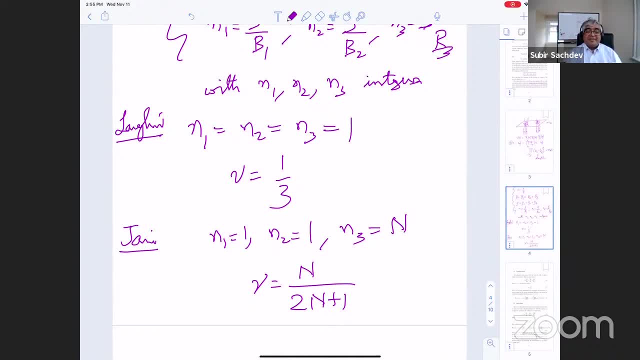 just happened to be n over 2n plus one, and there was this very elaborate theory, and there was this very elaborate theory, and there was this very elaborate theory of hierarchy, of hierarchy, of hierarchy, which, which, which famous people were talking about. famous people were talking about. 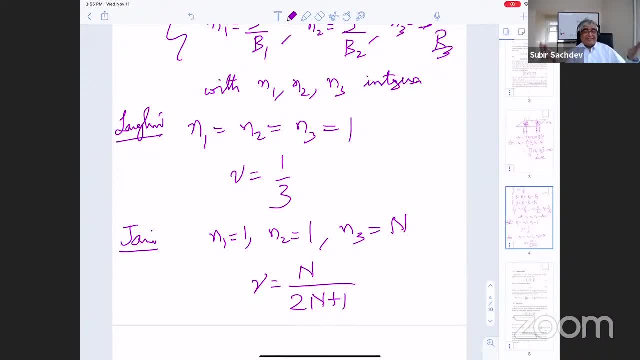 famous people were talking about which giving all kinds of fractions, but which giving all kinds of fractions, but which giving all kinds of fractions, but these particular fractions were nothing. these particular fractions were nothing. these particular fractions were nothing, presented, presented, presented. which gave this beautiful answer? smack on. 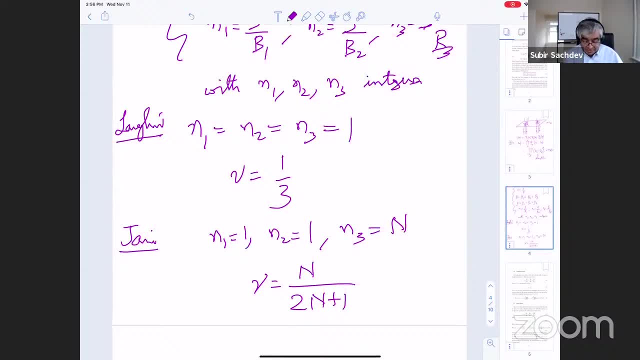 which gave this beautiful answer? smack on, which gave this beautiful answer? smack on uh to what uh. uh to what uh. uh to what uh. what's being observed? what's being observed, what's being observed? so you can see the. so you can see the. so you can see the. with the benefit of hindsight, this is one. 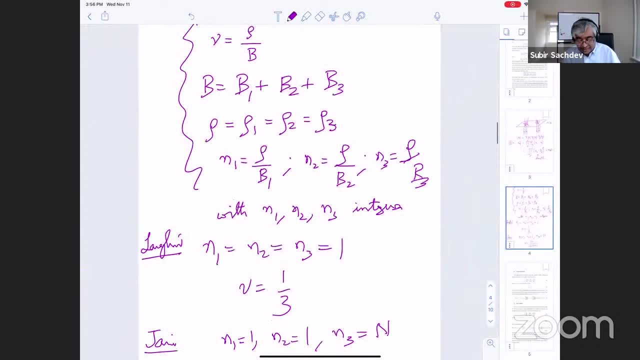 with the benefit of hindsight. this is one with the benefit of hindsight. this is one of the triumphs of the part-time, of the triumphs of the part-time, of the triumphs of the part-time approach, approach, approach where the basic idea is: you pick your. 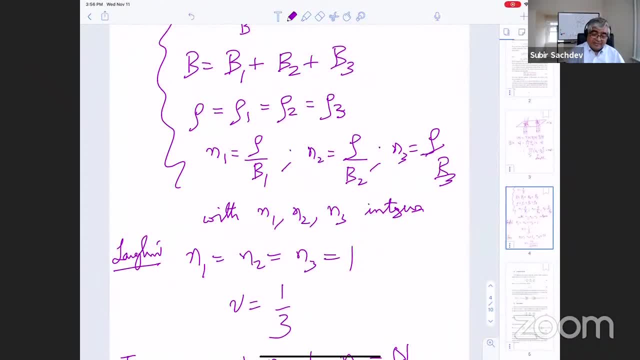 where the basic idea is: you pick your. where the basic idea is: you pick your. patterns carefully, patterns carefully, patterns carefully, and then try to find a mean field that, and then try to find a mean field that, and then try to find a mean field that has a gap. 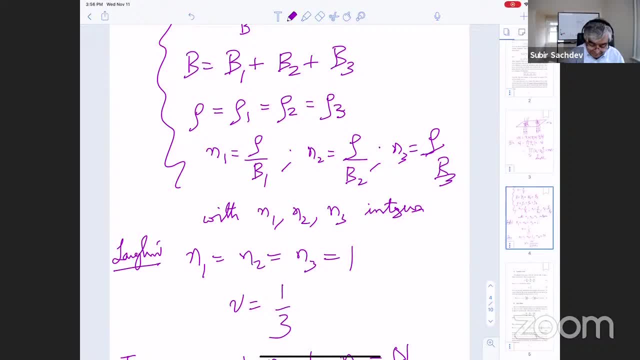 has a gap, has a gap, and then there's a pretty good bet. and then there's a pretty good bet, and then there's a pretty good bet- you're getting, you're on to something. you're getting, you're on to something. you're getting, you're on to something, okay, so that's what we all we're doing. okay, so that's what we all we're doing. okay, so that's what we all we're doing. you take our protons. you find a gap in you. take our protons, you find a gap in you. take our protons, you find a gap in the mean field, then we 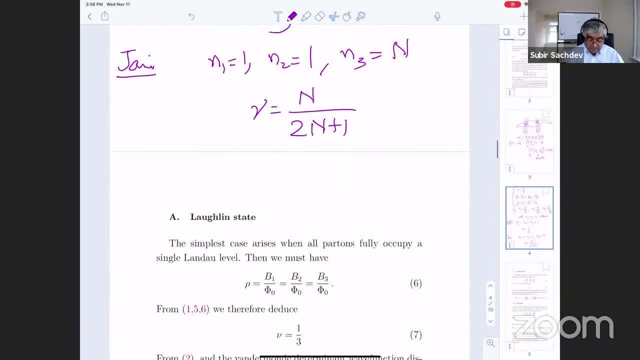 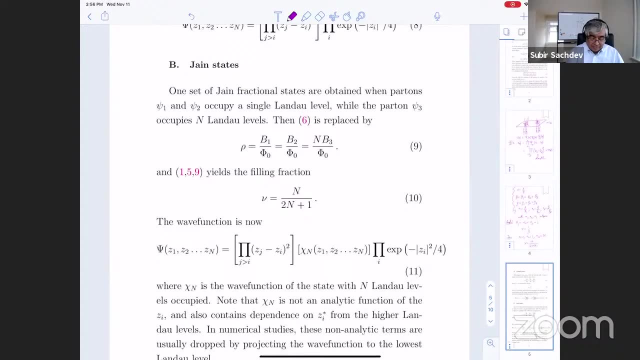 the mean field, then we the mean field, then we look at the gauge fluctuations. all right, all right, all right, so those are the jane states, so those are the jane states. so those are the jane states, and you can write down the wave function. and you can write down the wave function, then you have a wave function which has: 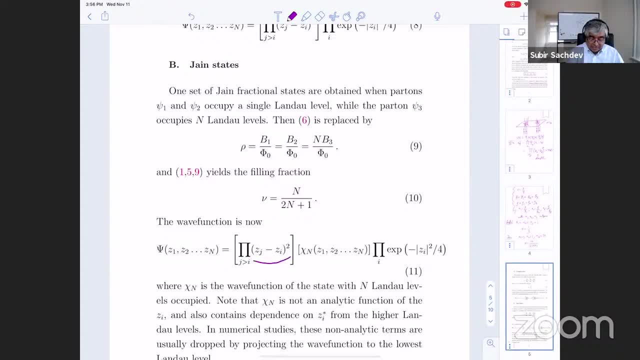 then you have a wave function which has: then you have a wave function which has this, this: this factor of zi minus zj, squared from the factor of zi minus zj, squared from the factor of zi minus zj squared from the first two protons, and then the wave. 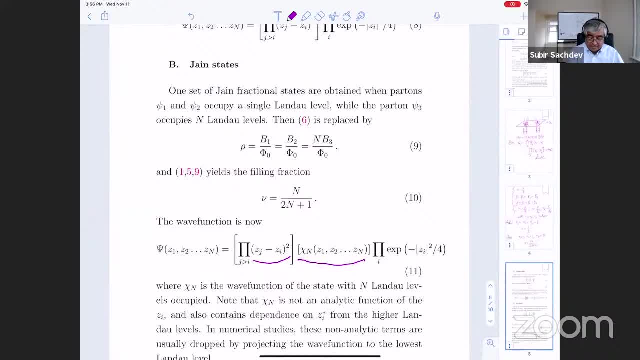 first two protons and then the wave. first two protons and then the wave. function of the particles, function of the particles, function of the particles in the higher land, all levels from the in the higher land, all levels from the in the higher land, all levels from the third part on. 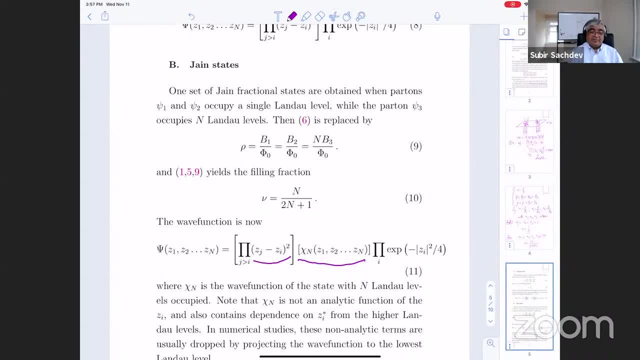 third part on. third part on: uh, this is no longer analytic. uh, this is no longer analytic. uh, this is no longer analytic, so it's not really a wave function. the- so it's not really a wave function. the- so it's not really a wave function. the lowest land all level. 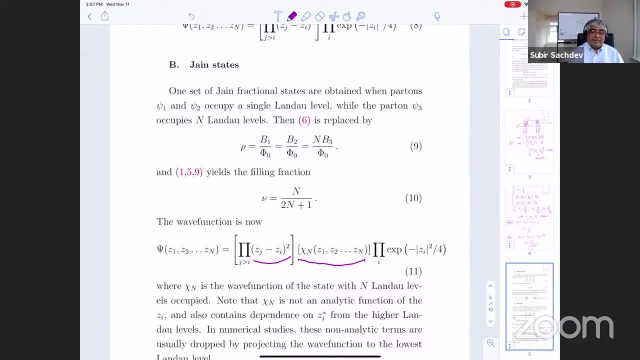 lowest land, all level. lowest land, all level, even though the filling the filling is, even though the filling the filling is, even though the filling the filling is less than one, less than one, less than one, uh, and that this was you know of some, uh, and that this was you know of some. 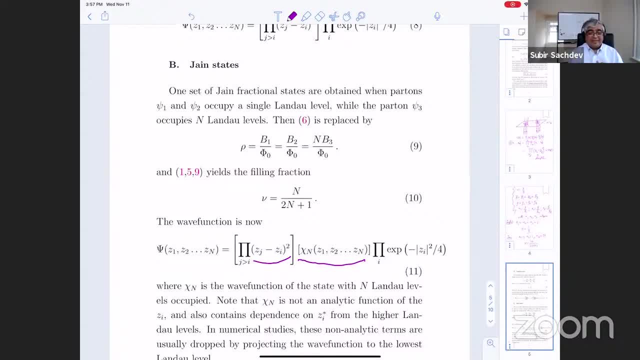 uh, and that this was, you know, of some concern i mean this is. i think that's the concern i mean this is. i think that's the concern i mean this is. i think that's the reason why, reason why, reason why other people didn't dare to write this. 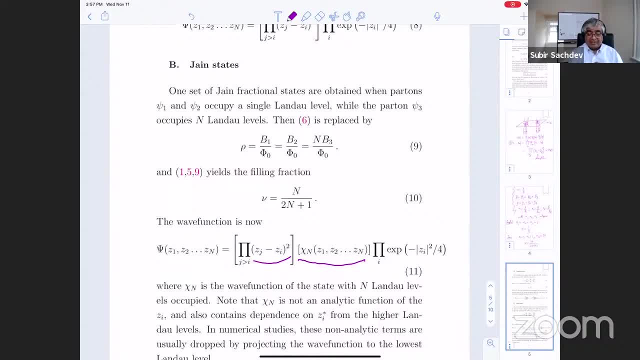 other people didn't dare to write this. other people didn't dare to write this down because they just there was this down, because they just there was this down, because they just there was this. dogma that whatever wave function you. dogma that whatever wave function you. 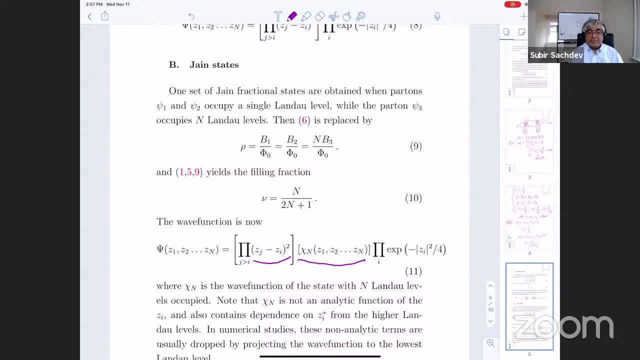 dogma that whatever wave function you write down must be analytic, write down must be analytic, write down must be analytic. uh, uh, uh. but it turned out that dogma was not. but it turned out that dogma was not. but it turned out that dogma was not correct. 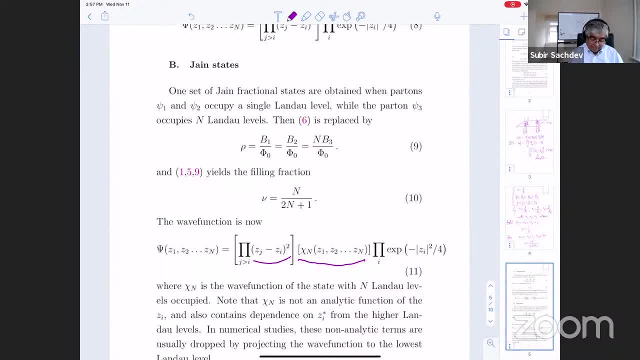 correct, correct. it's okay to have a little bit of. it's okay to have a little bit of. it's okay to have a little bit of analyticity and, in fact, what the way jn analyticity? and, in fact, what the way jn analyticity and, in fact, what the way jn fixed in numerical studies? you just drop. 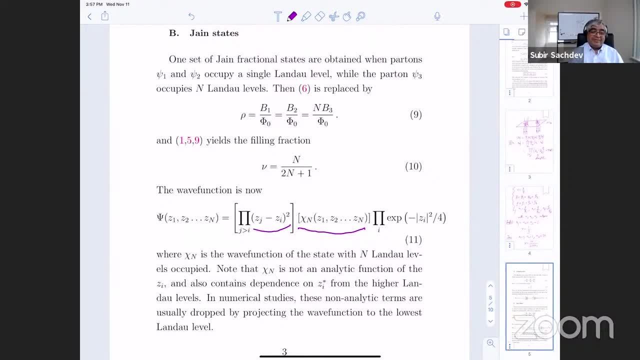 fixed in numerical studies, you just drop. fixed in numerical studies, you just drop the non-analytic term, you just project the non-analytic term. you just project the non-analytic term, you just project them out, them out, them out, uh, uh, uh, and then everything works and you know. 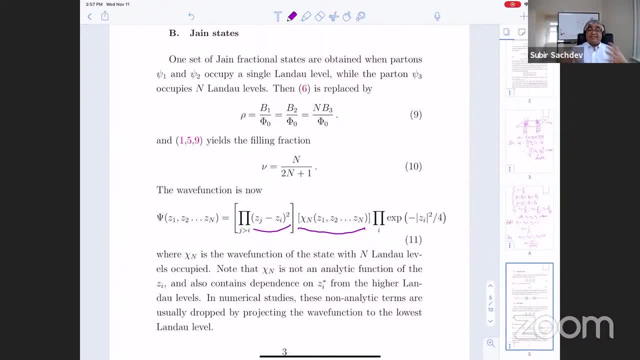 and then everything works and you know, and then everything works and you know. project them out is similar to project them out is similar to project them out is similar to doing the gauge integrals gauge, doing the gauge integrals gauge. doing the gauge integrals gauge fluctuations. 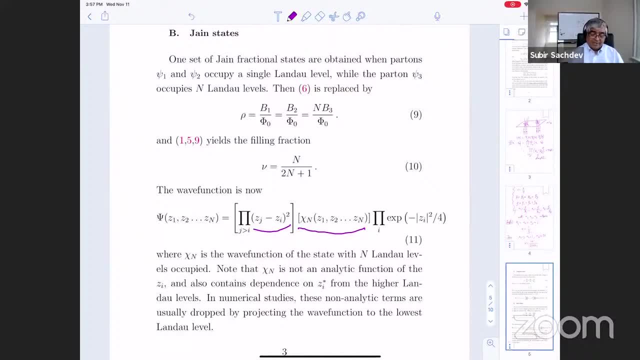 fluctuations, fluctuations, uh, uh, uh. and so this is the and so this is the and so this is the correct. the modern understanding would be correct. the modern understanding would be correct. the modern understanding would be: yes, yes, yes, you can project the gauge. you can project the gauge. 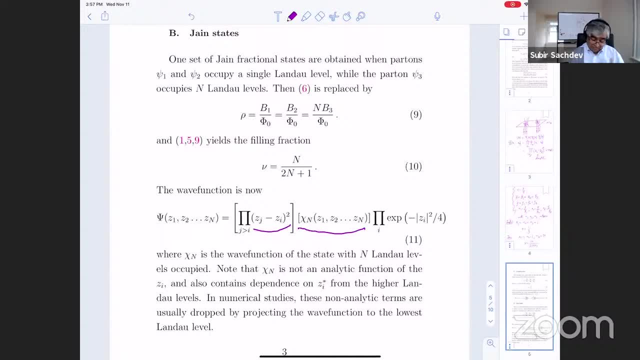 you can project the gauge, project out the non-analytic terms, project out the non-analytic terms, project out the non-analytic terms. that's like doing the theory of gauge, that's like doing the theory of gauge, that's like doing the theory of gauge fluctuations. and that's fine because the 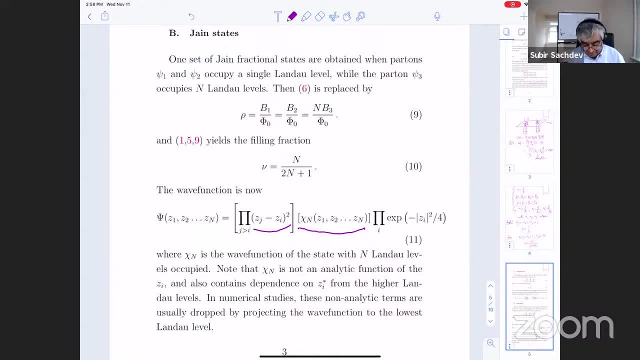 fluctuations and that's fine because the fluctuations. and that's fine because the gauge look there's a gap and the gauge gauge look there's a gap and the gauge gauge look there's a gap and the gauge fluctuations are all under control. fluctuations are all under control. 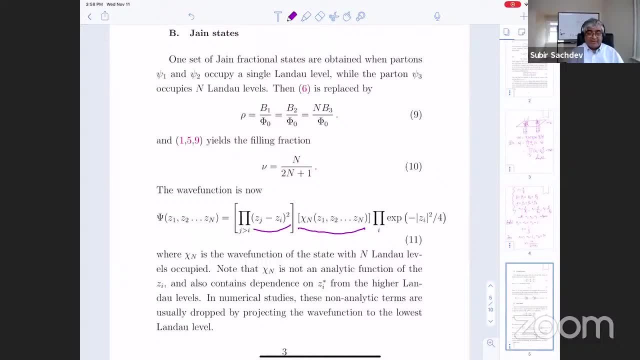 fluctuations are all under control. so the key really the key. so the key really the key. so the key really the key, key thing is able to find a mean field. key thing is able to find a mean field. key thing is able to find a mean field with a gap. 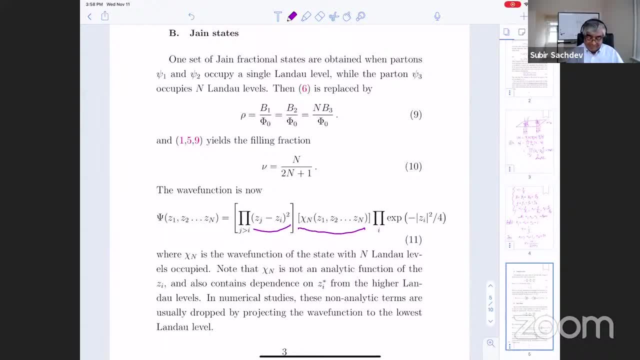 with a gap, with a gap, and that's more important than forcing, and that's more important than forcing, and that's more important than forcing. this analyticity, this analyticity, this analyticity, anyway, anyway, anyway, that's my two cents words, that's my two cents words. 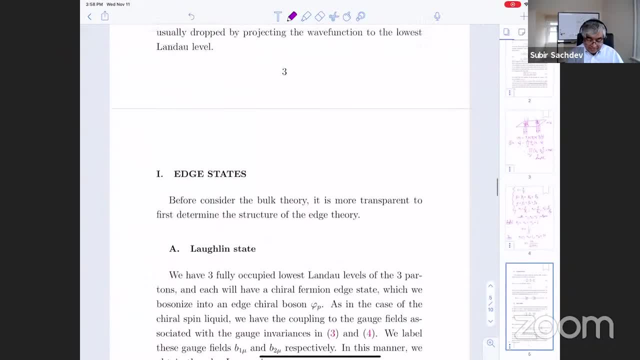 that's my two cents words. okay, okay, okay, uh, uh, uh, right, right, right. so there it is. so there it is. so there it is. and now that we have this part on, and now that we have this part on, and now that we have this part on construction, just like we did in the 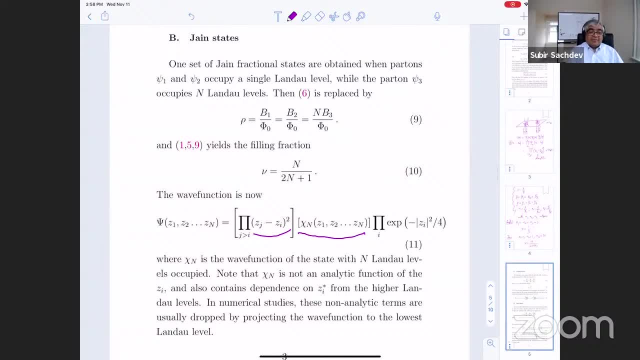 construction, just like we did in the construction, just like we did in the last chapter, last chapter, last chapter. uh, we can work out the chen simon's. uh, we can work out the chen simon's. uh, we can work out the chen simon's gauge theory. figure out the statistics. 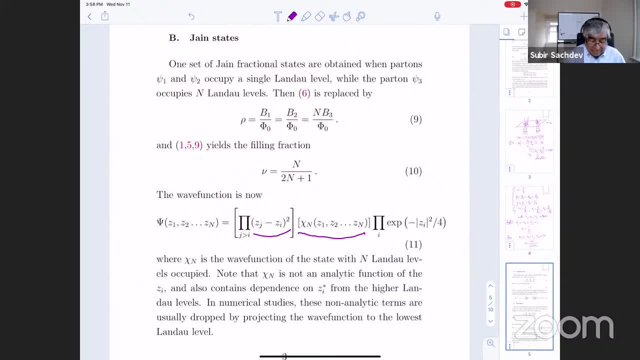 gauge theory: figure out the statistics. gauge theory: figure out the statistics. figure out the edge states. it's really a figure out the edge states. it's really a figure out the edge states. it's really a matter of turning the crank now. matter of turning the crank now. 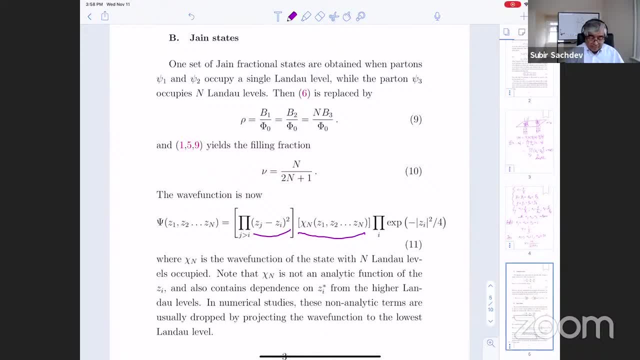 matter of turning the crank now. uh, uh, uh, but. but. but, in fact, the way i'm going to do it in, in fact, the way i'm going to do it in, in fact, the way i'm going to do it in this chapter, is the opposite of what i. this chapter is the opposite of what i. this chapter is the opposite of what i did in the previous chapter. we're going did in the previous chapter, we're going did in the previous chapter. we're going to do the edge states first because it to do the edge states first because it. 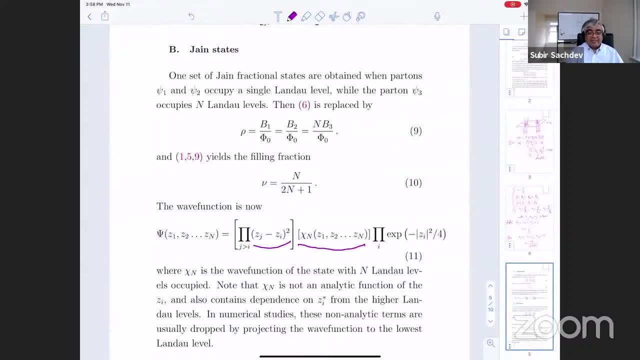 to do the edge states first, because it just turns out to be a bit simpler. just turns out to be a bit simpler, just turns out to be a bit simpler, um, because, on the edge states, as i um, because on the edge states, as i um, because on the edge states, as i showed you already, you can just do the. 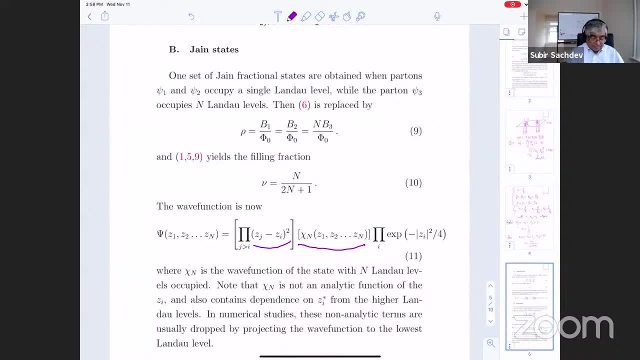 showed you already, you can just do the. showed you already, you can just do the integral, integral, integral, uh, uh, uh, over the, over the, over the, the gauge fields, exactly the gauge fields, exactly the gauge fields, exactly. and there was just this, very simple, and there was just this very simple. 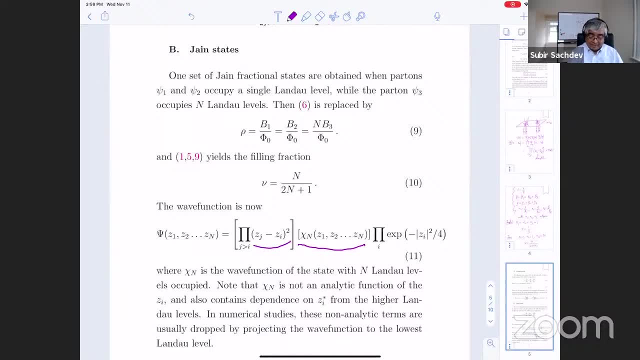 and there was just this very simple result: that phi up was minus phi down. result: that phi up was minus phi down. result: that phi up was minus phi down. and we'll get very similar things here, and we'll get very similar things here, and we'll get very similar things here. so 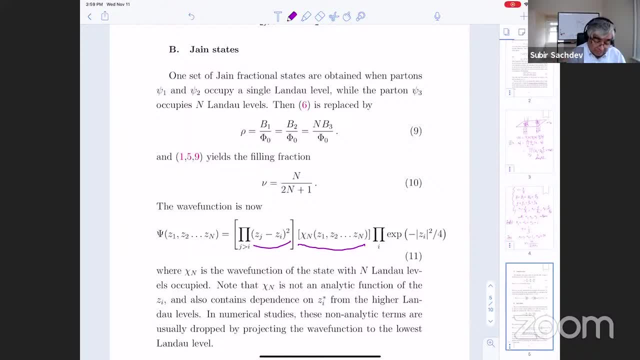 so so, and so this way you can get the full k, and so this way you can get the full k, and so this way you can get the full k matrix. it turns out that this integer f is the same as the that this integer f is the same as the. that this integer f is the same as the integer n, integer n, integer n. in the chern-simons gauge theories: the. in the chern-simons gauge theories, the. in the chern-simons gauge theories, the number of gauge fields. number of gauge fields. 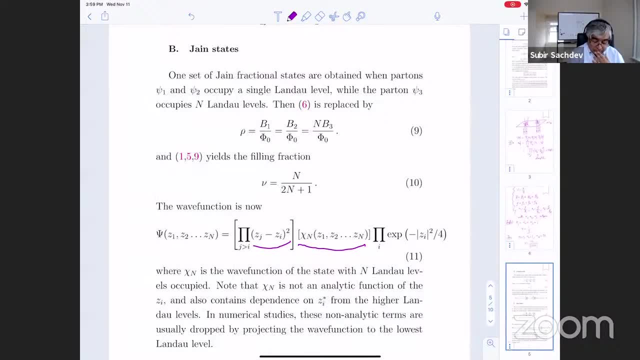 number of gauge fields are left over after you have done all the are left over after you have done all the projections, projections, projections, um. so that's why i called it capital um. so that's why i called it capital um. so that's why i called it capital n. so n equals one is the laughlin case. 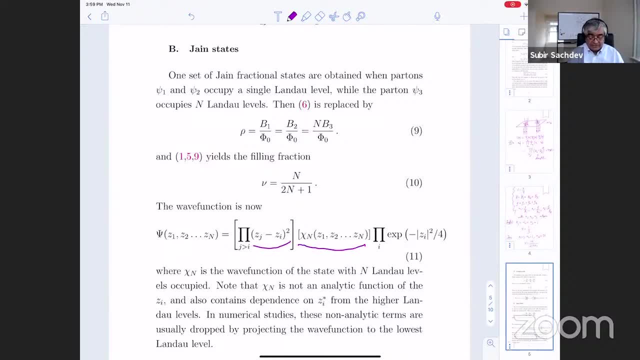 n, so n equals one is the laughlin case. n, so n equals one is the laughlin case. and so that for the jane states like n, and so that for the jane states like n, and so that for the jane states, like n equals two, which gives you the two. 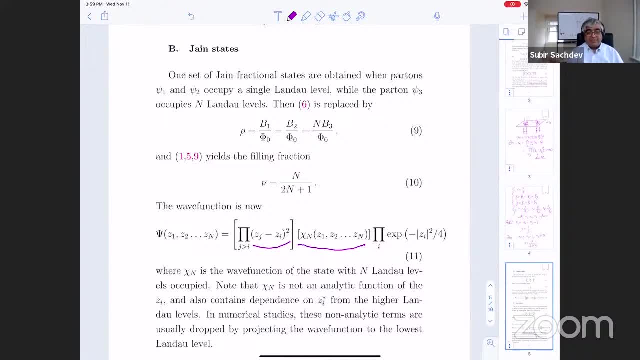 equals two, which gives you the two. equals two, which gives you the two. fifth fraction. fifth fraction. fifth fraction: is there is an example of the n equals? is there is an example of the n equals? is there is an example of the n equals two, case where there will be two? 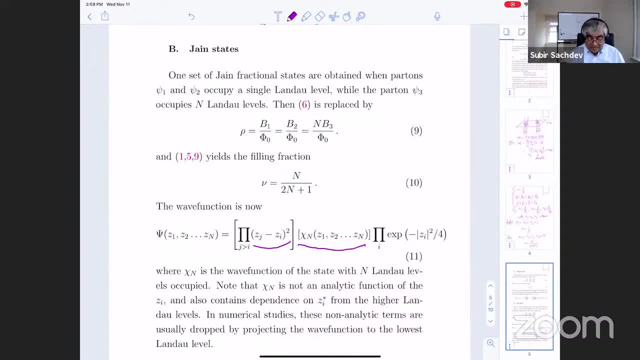 two case where there will be two. two case where there will be two independent edge modes, and so on. independent edge modes, and so on. independent edge modes, and so on. okay, i think that's four o'clock, so i. okay, i think that's four o'clock, so i. 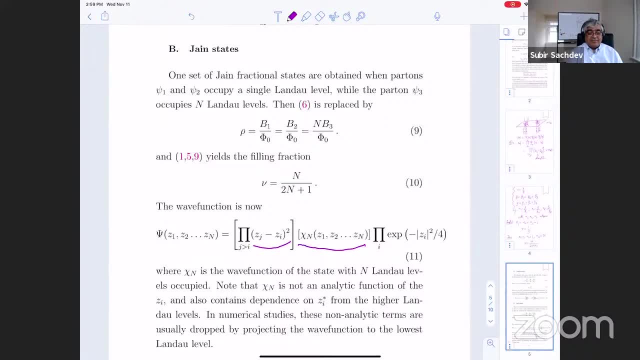 okay, i think that's four o'clock, so i will stop there, will stop, there, will stop there. uh, and the next uh, and the next uh, and the next. then we'll finish the jane state theory, then we'll finish the jane state theory, then we'll finish the jane state theory. uh, next time. and then i want to start. 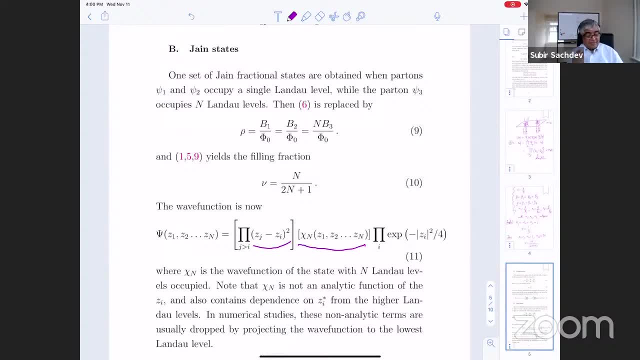 uh next time, and then i want to start uh next time and then i want to start uh really in some ways, the most uh really in some ways, the most uh really in some ways, the most spectacular of the spectacular of the spectacular of the fractionalized states. 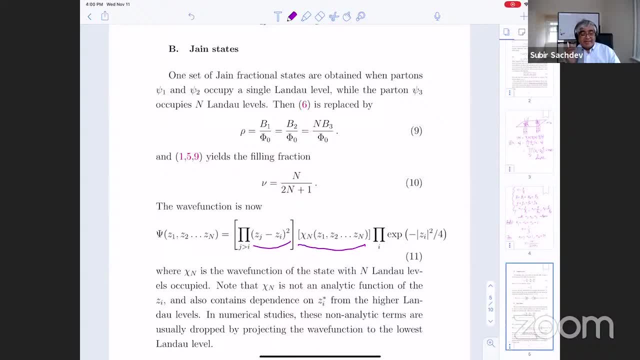 fractionalized states. fractionalized states, um, um, um, which is the, which is the, which is the non-abelian icing state of guitar. non-abelian icing state of guitar. non-abelian icing state of guitar. and again, i'll do it by the same this. 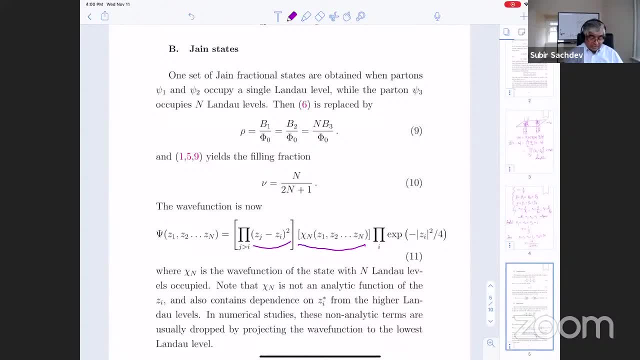 and again i'll do it by the same this and again i'll do it by the same this: this very general part-time type, this very general part-time type, this very general part-time type, approach, approach, approach. we'll see that. uh, we'll see that, uh. 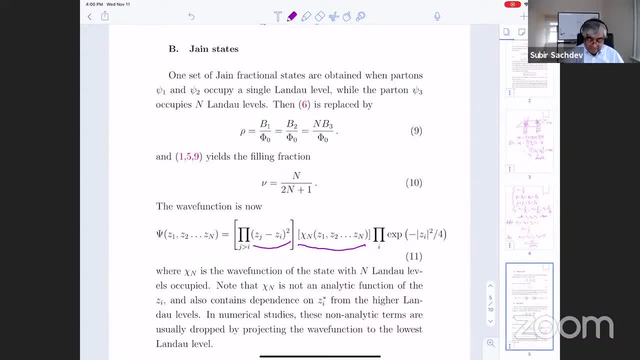 we'll see that, uh, it just comes from a very subtle twist. it just comes from a very subtle twist. it just comes from a very subtle twist on the z2 spin liquid, on the z2 spin liquid. on the z2 spin liquid is how you get the non-abelian states. 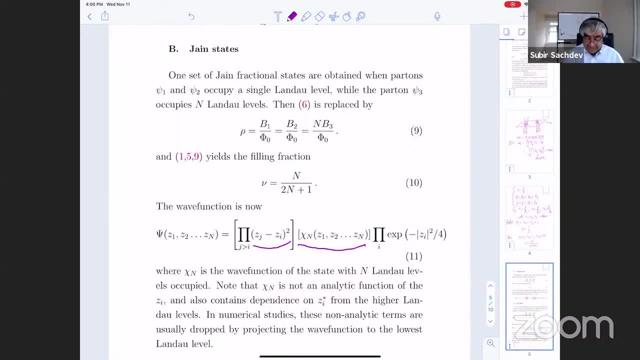 is how you get the non-abelian states is how you get the non-abelian states. i'm still learning up part of the. i'm still learning up part of the. i'm still learning up part of the non-abelian state myself. so i have the. 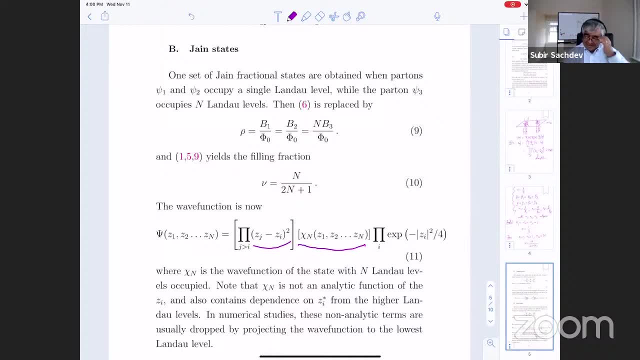 non-abelian state myself. so i have the non-abelian state myself, so i have the weekend to weekend to weekend to to get everything right. but i think i to get everything right, but i think i to get everything right, but i think i have. 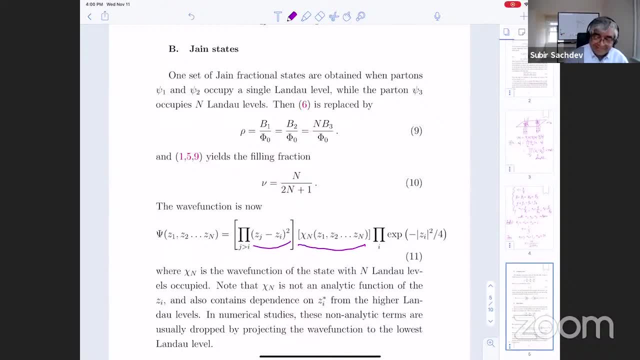 have have. i certainly have understood enough to. i certainly have understood enough to. i certainly have understood enough to give the lecture on friday. all right, any questions. all right, any questions. all right, any questions. hi, yeah, i actually have a question it. hi, yeah, i actually have a question it. 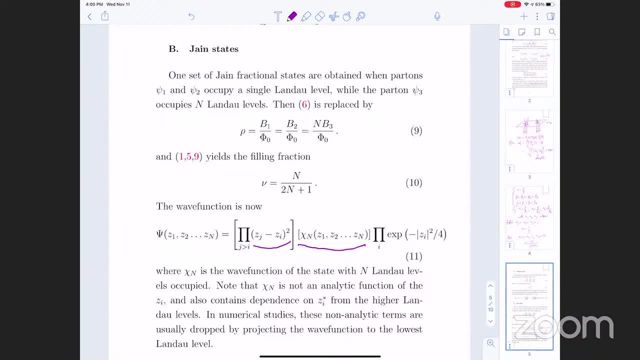 hi. yeah, i actually have a question. it sounded like. sounded like. sounded like we originally motivated having three. we originally motivated having three. we originally motivated having three part-times by this, part-times by this, part-times by this. new equals one-third uh case. yeah. new equals one-third uh case, yeah. 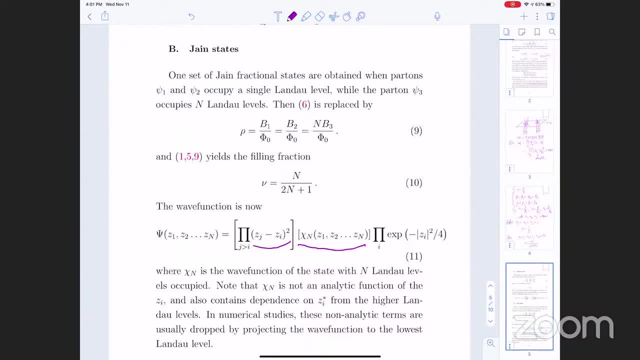 new equals one-third. uh case, yeah, exactly was three the one that exactly was three. the one that exactly was three, the one that we picked. or is like: why is three the we picked? or is like why is three the we picked? or is like why is three the one that works. 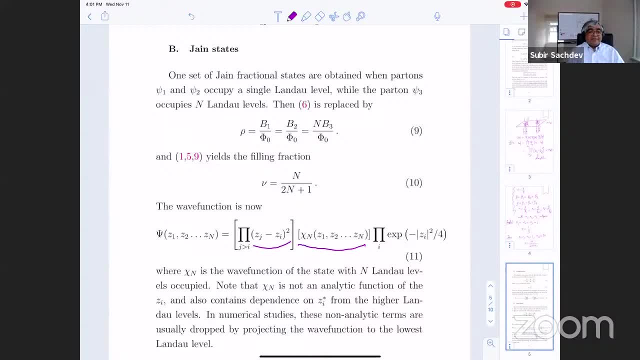 one that works. one that works? yeah, you can, you can pick others. so yeah, you can. you can pick others. so yeah, you can, you can pick others. so if you wanted to describe the fractional, if you wanted to describe the fractional, if you wanted to describe the fractional quantum state at nu equals one-fifth. 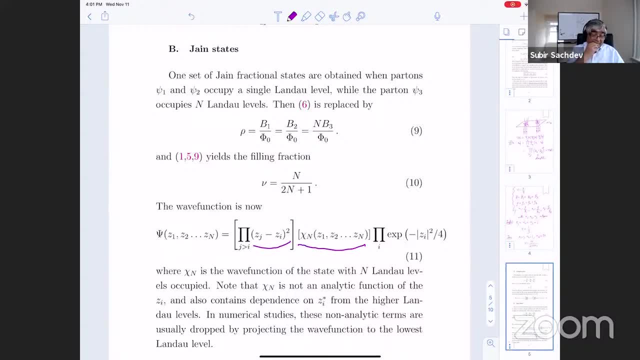 quantum state at nu equals one-fifth quantum state at nu equals one-fifth um, then you will have to pick five um. then you will have to pick five um. then you will have to pick five patterns, patterns, patterns, and do it that way. i mean, it's just. 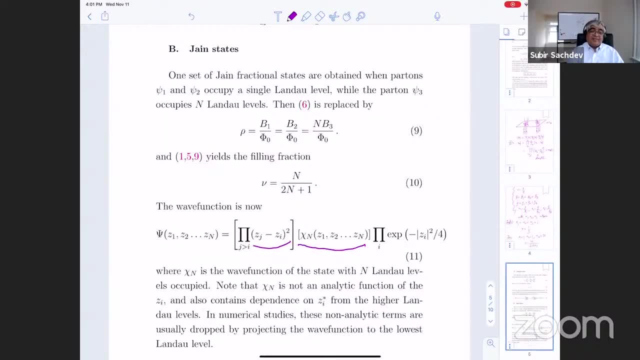 and do it that way, i mean it's just. and do it that way, i mean it's just more work. i'm just doing the simplest, more work. i'm just doing the simplest, more work. i'm just doing the simplest case, case, case, uh, i see, and then uh. 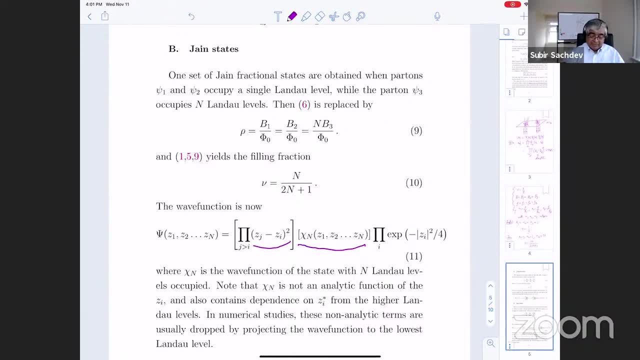 uh, i see, and then uh, uh, i see, and then, uh, you know, and there's the jane sequences, you know, and there's the jane sequences, you know, and there's the jane sequences with more than one jane sequence, this is. with more than one jane sequence, this is. 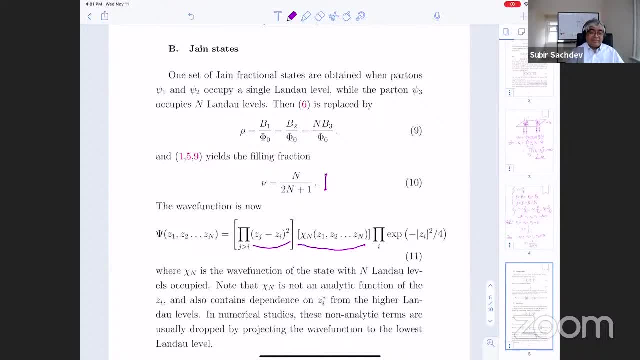 with more than one jane sequence. this is the simplest of the jane sequences. that the simplest of the jane sequences, that the simplest of the jane sequences that i'm i'm i'm describing here, so there's various other describing here, so there's various other describing here. so there's various other fractions that you get by. 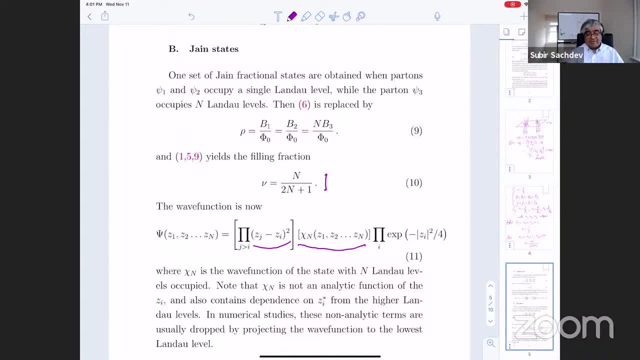 fractions that you get by, fractions that you get by um by putting one of those protons in um. by putting one of those protons in um, by putting one of those protons in a higher random levels, the others in the a higher random levels, the others in the. 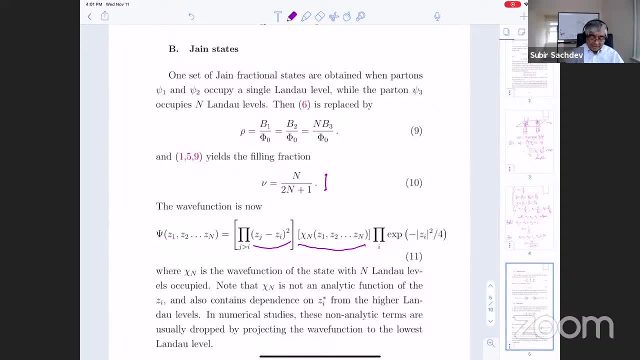 a higher random levels, the others in the lower one, and so on, lower one and so on, lower one, and so on. uh, i'm not an expert on this, but there's- uh, i'm not an expert on this, but there's- uh, i'm not an expert on this, but there's a incredible zoo of possibilities here. 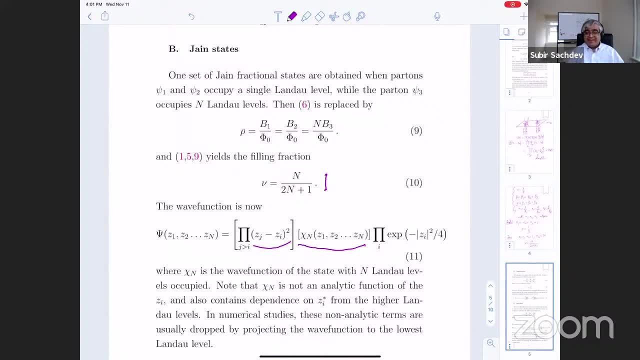 a incredible zoo of possibilities here. a incredible zoo of possibilities here. i'm just showing you the two simplest. i'm just showing you the two simplest. i'm just showing you the two simplest ones, ones, ones. but as far as i know every known state, but as far as i know every known state, 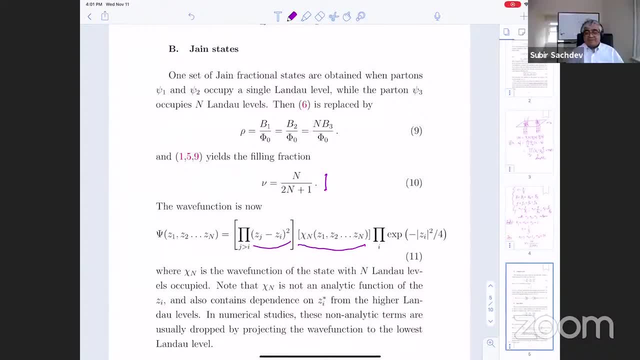 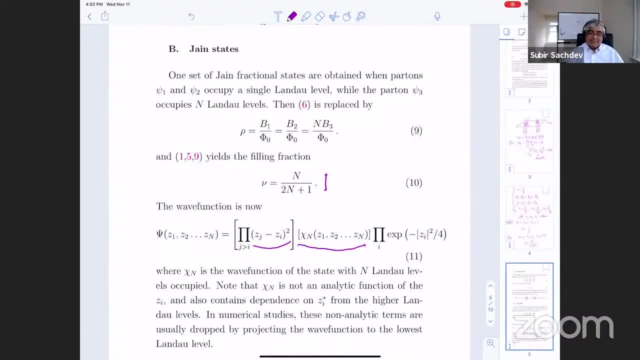 state. that's quite a bit more state, that's quite a bit more complicated, but complicated, but complicated. but you know that i won't describe. you know that i won't describe. you know that i won't describe. i i guess a follow-up, i don't know if. 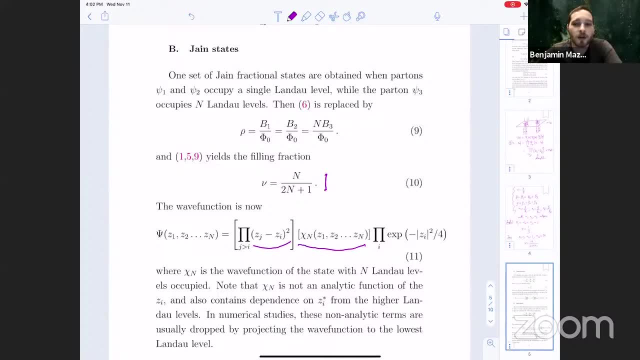 i, i guess a follow-up. i don't know if i i guess a follow-up. i don't know if this is something that you'd readily. this is something that you'd readily, this is something that you'd readily have the answer to, but are there? have the answer to, but are there? 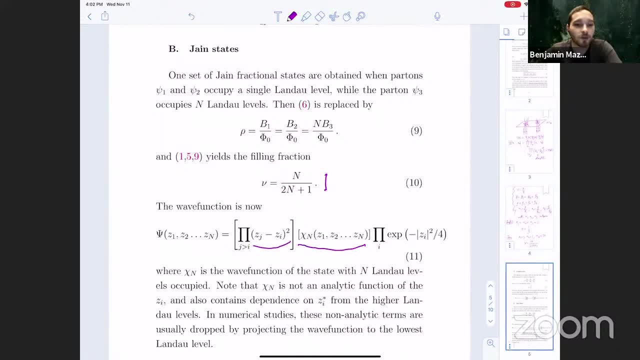 have the answer to. but are there some states that can be equally well? have the answer to. but are there some states that can be equally well? have the answer to. but are there some states that can be equally well described with different numbers of? described with different numbers of? 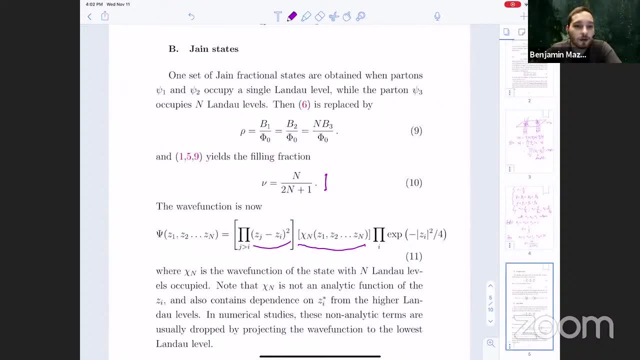 described with different numbers of partons. uh, uh, uh, it could be, but i, yeah, i'm not aware of it could be, but i, yeah, i'm not aware of it could be, but i, yeah, i'm not aware of. yeah, i mean, in the end, what's the, the invariant?